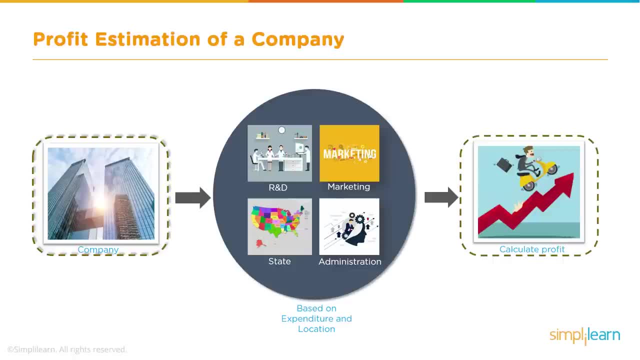 all this different information, we would like to calculate the profit Now. in actuality, there's usually about twenty three to twenty seven different markers that they look at. If they're looking at a company, they're looking at a company that's going to invest in it. If they're looking 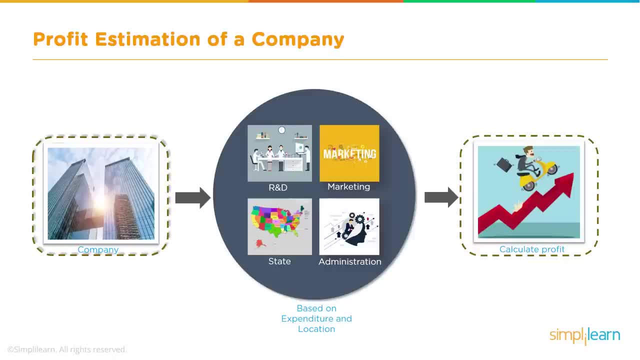 at a company that's going to invest in it. they're looking at a company that's going to invest in it or a heavy duty investor. We're only going to take a look at one basic one. We're going to come in and, for simplicity, let's consider a single variable R&D and find out which companies to 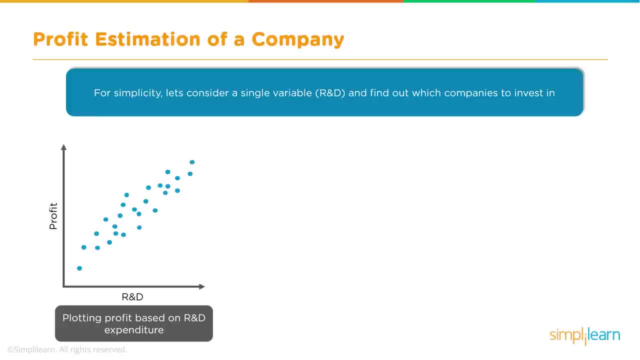 invest in based on that. So we take our R&D and we're plotting the profit based on the R&D expenditure, how much money they put into the research and development, and then we look at the profit that goes with that. We can predict a line to estimate the profit, so we can draw. 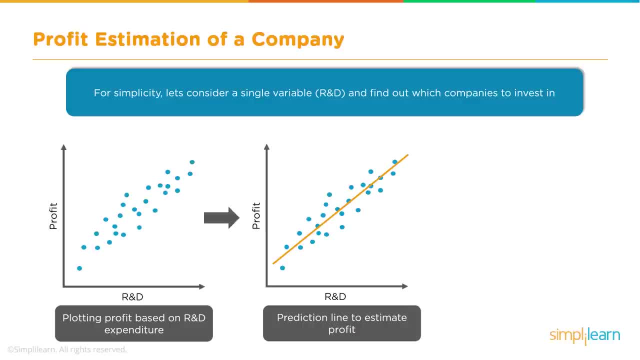 a line right through the data. When you look at that, you can see how much they invest in the R&D. There's a good marker as to how much profit they're going to make. We can also note that companies spending more on R&D make good profit. so let's invest in. 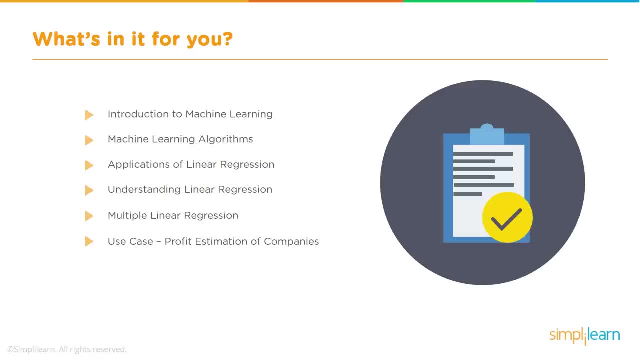 the ones that spend a higher rate in their R&D. What's in it for you? First, we'll have an introduction to machine learning, followed by machine learning algorithms. These will be specific to linear regression and, where it fits into the larger model, Then we'll. 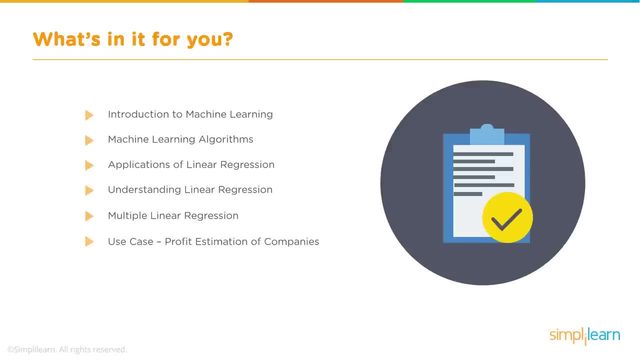 take a look at applications of linear regression, understanding linear regression and multiple linear regression. Finally, we'll roll up our sleeves and do a little programming in use case profit estimation of companies. Let's go ahead and jump in. Let's start with our introduction. 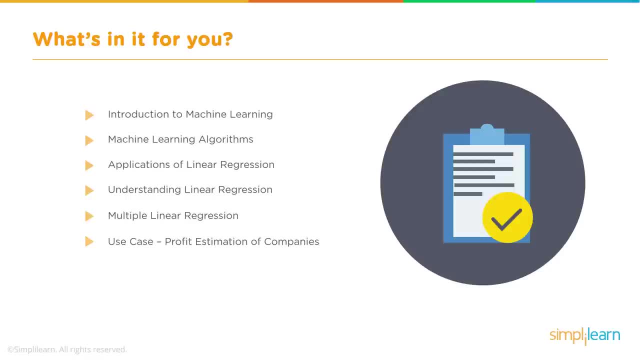 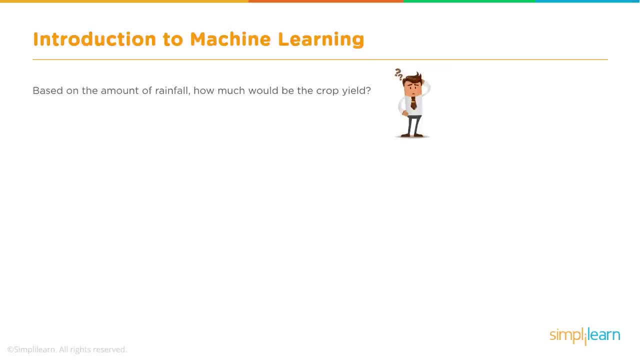 to machine learning, along with some machine learning algorithms and, where that fits in, with linear regression. Let's look at another example of machine learning. Based on the amount of rainfall, how much would be the crop yield? Here we have our crops, we have. 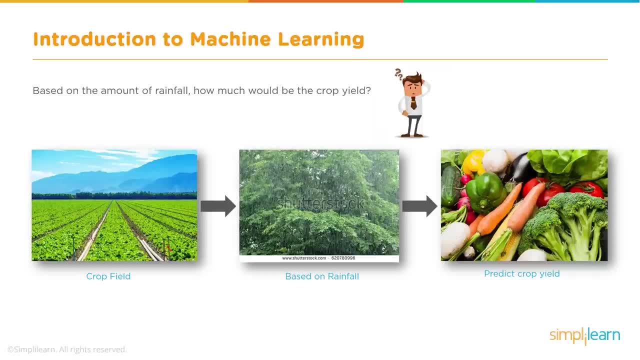 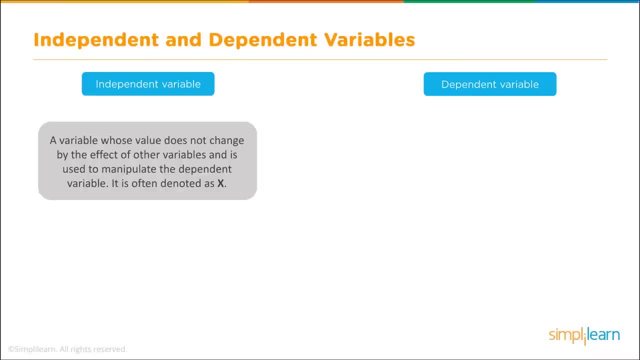 our rainfall and we want to know how much we're going to get from our crops. this year We're going to use two variables: independent and dependent. The independent variable is not changed by the effect of other variables and is used to manipulate the dependent variable. 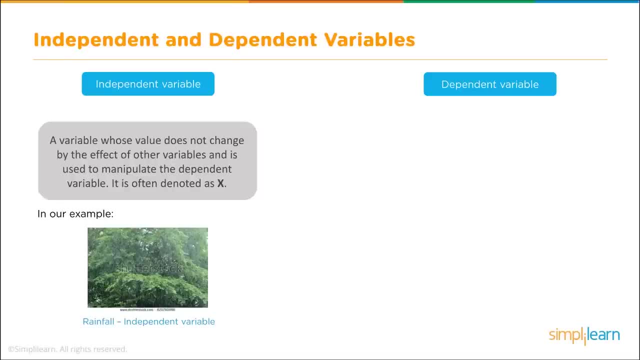 It is often denoted as X. In our example, rainfall is the independent variable. This is a wonderful example, because you can easily see that we can't control the rain, but the rain does control the crop. So we talk about the independent variable, controlling the dependent. 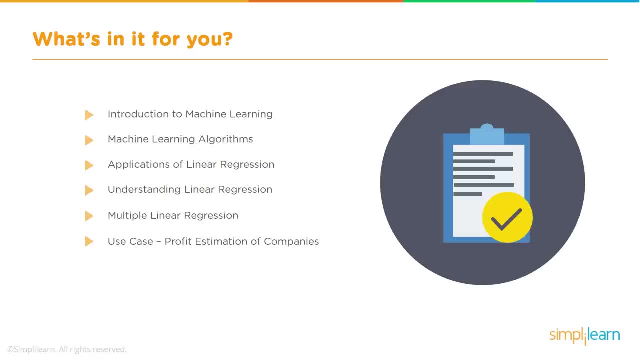 the ones that spend a higher rate in their R&D. What's in it for you? First, we'll have an introduction to machine learning, followed by machine learning algorithms. These will be specific to linear regression and, where it fits into the larger model, Then we'll. 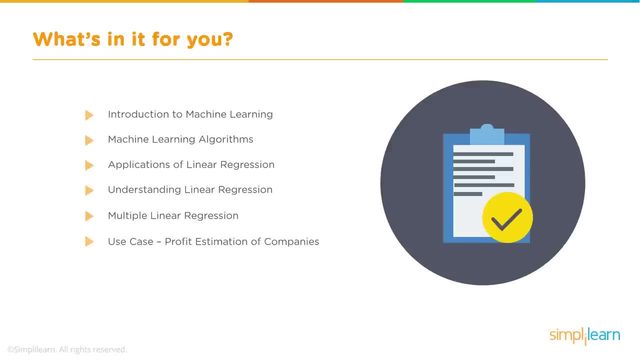 take a look at applications of linear regression, understanding linear regression and multiple linear regression. Finally, we'll roll up our sleeves and do a little programming in use case profit estimation of companies. Let's go ahead and jump in. Let's start with our introduction. 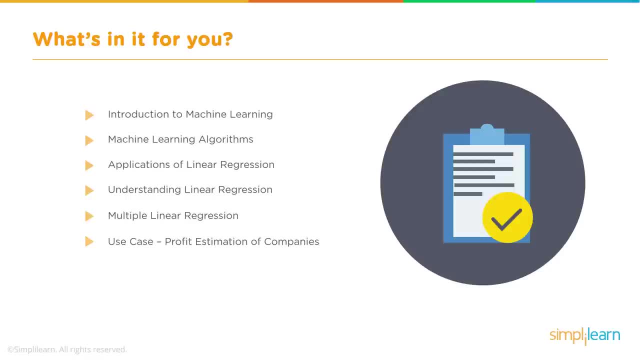 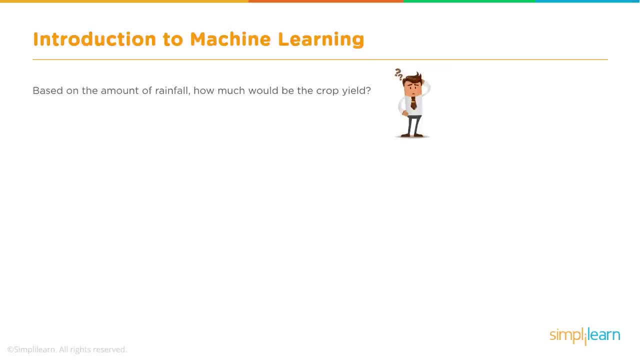 to machine learning, along with some machine learning algorithms and, where that fits in, with linear regression. Let's look at another example of machine learning. Based on the amount of rainfall, how much would be the crop yield? Here we have our crops, we have. 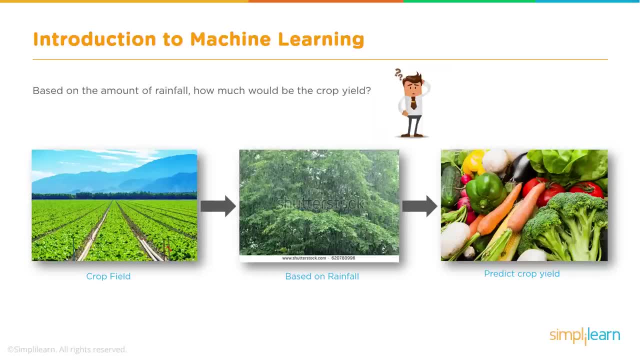 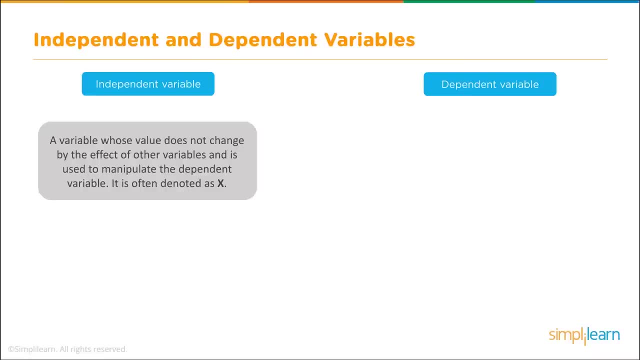 our rainfall and we want to know how much we're going to get from our crops. this year, We're going to use two variables: independent and dependent. The independent variable is a variable whose value is not changed by the effect of other variables and is used to manipulate the dependent variable. 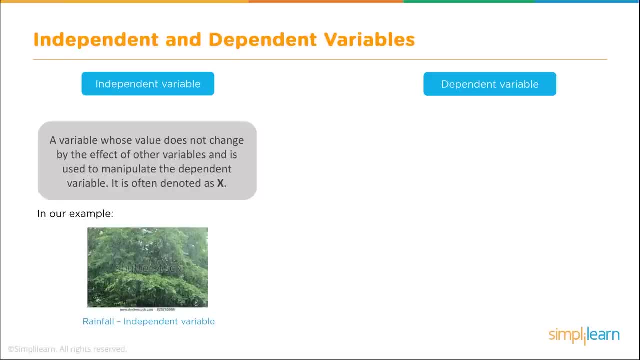 It is often denoted as X. In our example, rainfall is the independent variable. This is a wonderful example, because you can easily see that we can't control the rain, but the rain does control the crop. So we talk about the independent variable, controlling the dependent. 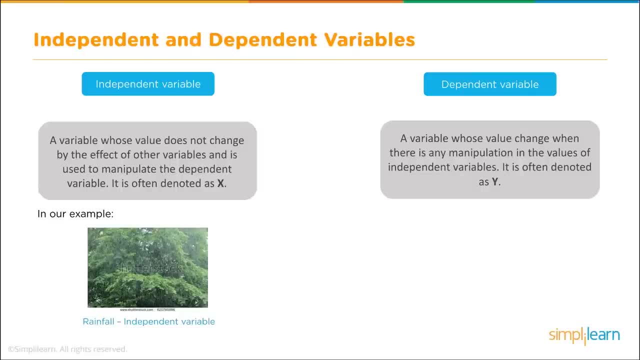 variable. Let's define dependent variable as a variable whose value change when there is any manipulation of the values of the independent variables. It is often denoted as Y. You can see here: our crop yield is dependent variable and it is dependent on the amount of rainfall received. 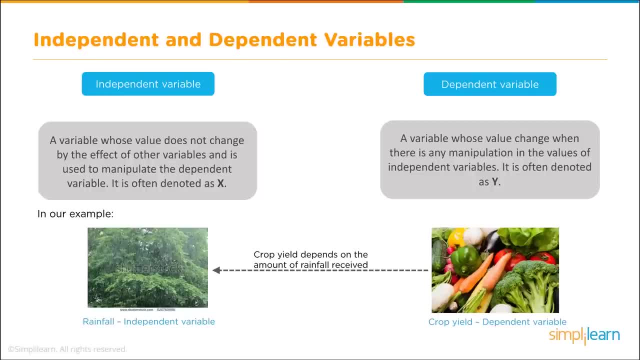 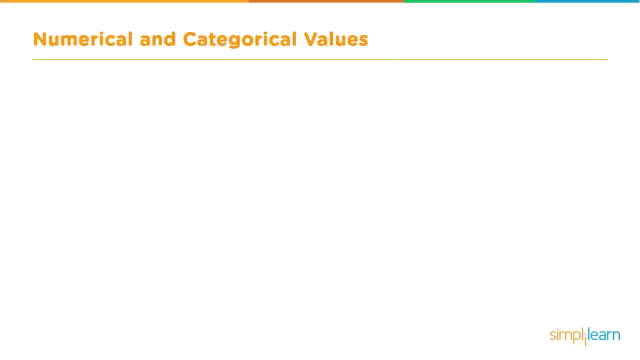 Now that we've taken a look at a real life example, let's go a little bit into the theory and some definitions on machine learning and see how that fits together with linear regression, Numerical and categorical values. Let's take our data coming in. This is kind of random. 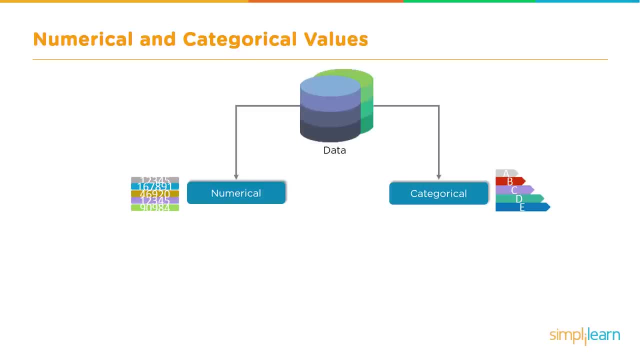 data from any kind of project. We want to divide it up into numerical and categorical. So numerical is numbers- age, salary, height- where categorical would be a description, the color a dog's breed, gender. Categorical is limited to very specific items, where numerical is a range of information. Now that you've 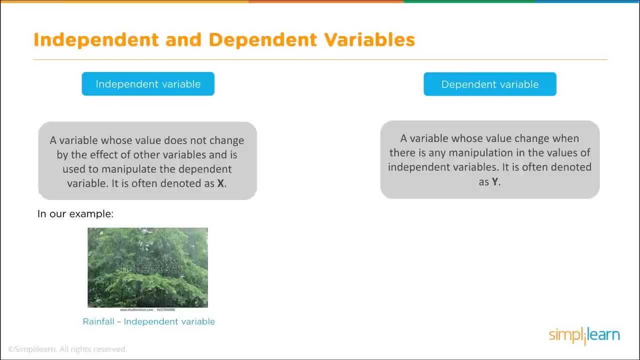 variable. Let's define dependent variable as a variable whose value change when there is any manipulation of the values of the independent variables. It is often denoted as Y And you can see here: crop yield is dependent variable and it is dependent on the amount of rainfall. 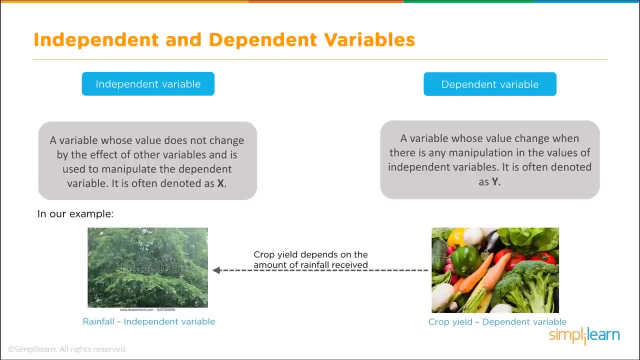 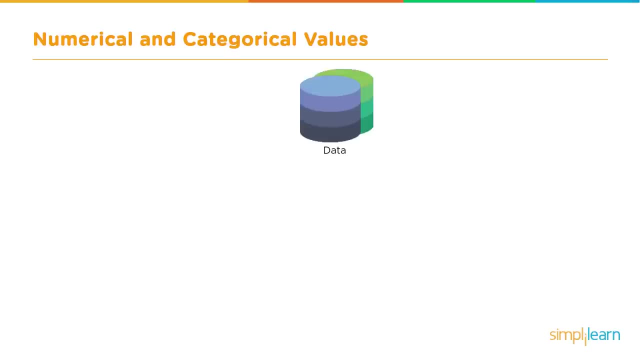 received. Now that we've taken a look at a real-life example, let's go a little bit into the theory and some definitions on machine learning and see how that fits together with linear regression, Numerical and categorical values. Let's take our data coming in. This is kind of random data from any kind of project We 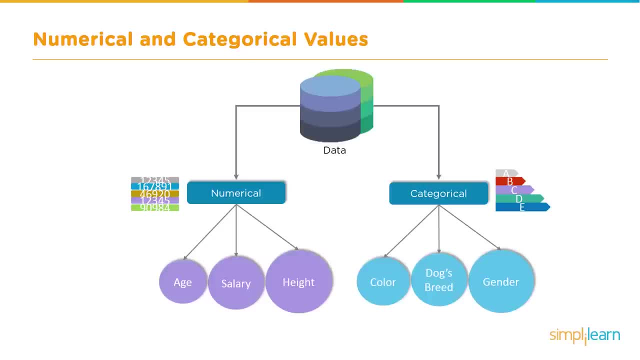 want to divide it up into numerical and categorical. So numerical is numbers- age, salary, height- where categorical would be a description, the color a dog's breed, gender. Categorical is limited to very specific items, where numerical is a range of information. Now that you've seen the difference between numerical, 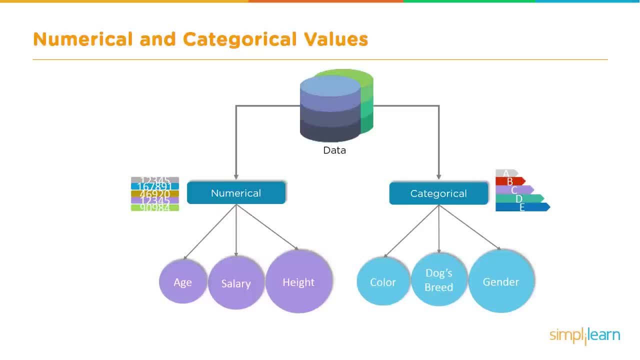 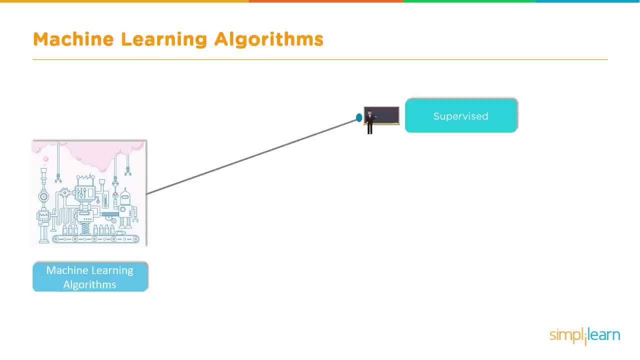 and categorical data. let's take a look at some different machine learning definitions. When we look at a different machine learning algorithms, we can divide them into three areas: Supervised, unsupervised and categorical. We can divide them into three areas: Supervised- unsupervised. 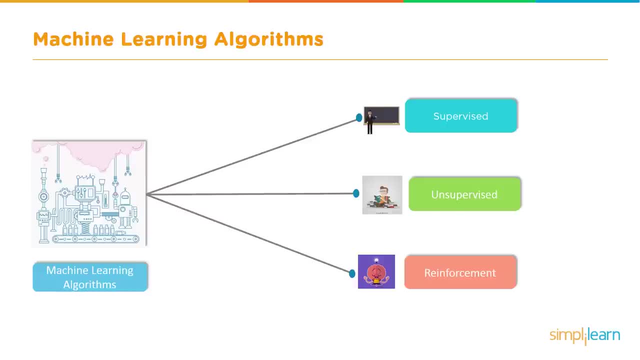 reinforcement. We're only going to look at supervised today. Unsupervised means we don't have the answer, so we're just grouping things. Reinforcement is where we give positive and negative feedback to our algorithm to program it, and it doesn't have the information until after the fact. But today we're just looking at 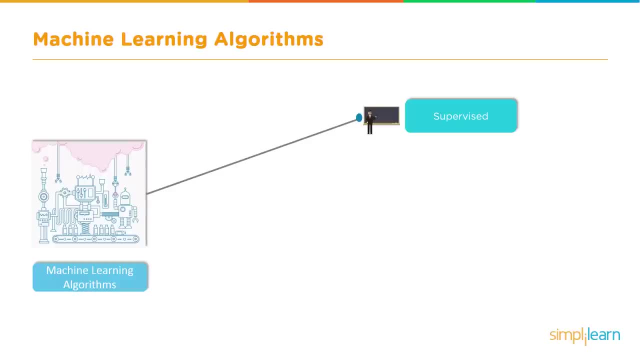 supervised, because that's where linear regression fits in. In supervised data we have our data already there and our answers for a group, and then we use that to program our model and come up with an answer. The two most common uses for that is through the regression and classification. Now we're doing linear. 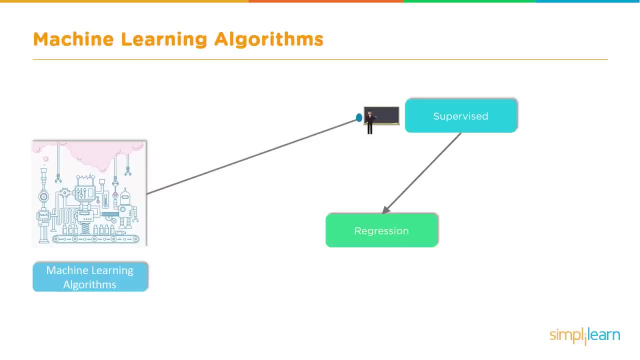 regression. so we're just going to focus on the regression side. And in the regression we have simple linear regression, we have multiple linear regression and we have polynomial linear regression. Now, on these three, simple linear regression is the examples we've looked at so far where we have a lot of 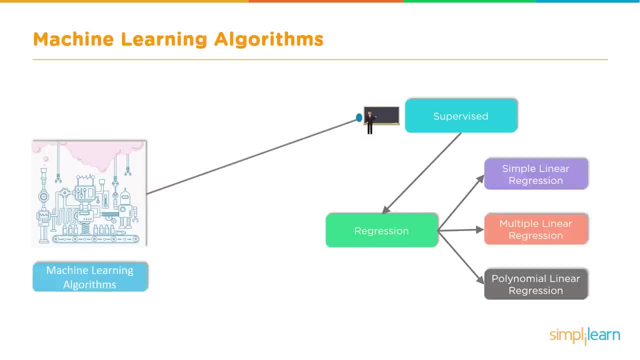 data and we draw a straight line through it. Multiple linear regression means we have multiple variables. Remember where we had the rainfall and the crops- and we might add additional variables in there, like how much food to we give our crops, When do we harvest them. Those would be additional information add into. 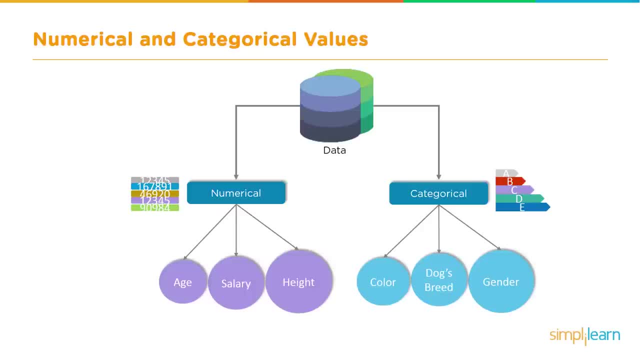 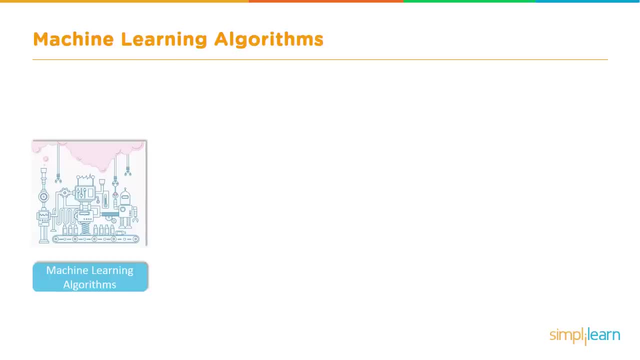 seen the difference between numerical and categorical data. let's take a look at some different machine learning definitions. When we look at our different machine learning algorithms, we can divide them into three areas: Supervised, unsupervised, reinforcement. We're only going to look at supervised today. Unsupervised means we don't have the answers. 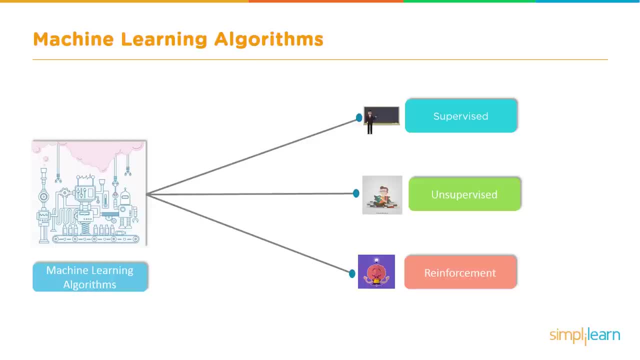 and we're just grouping things. Reinforcement is where we give positive and negative feedback to our algorithm to program it, and it doesn't have the information until after the fact. But today we're just looking at supervised, because that's where linear regression fits in In supervised data. we have our data already there and our answers for a group and then 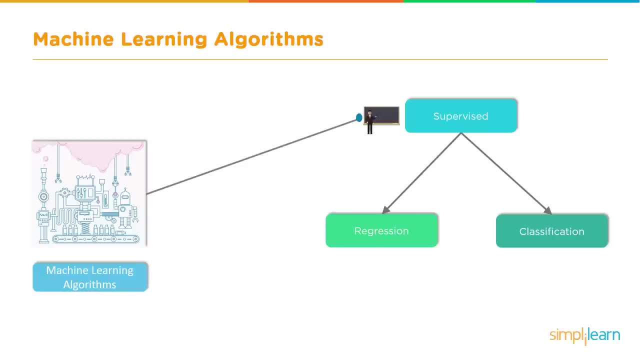 we use that to program our model and come up with an answer. The two most common uses for that is through the regression and the algorithm, Supervised and unsupervised, are the most common uses for linear regression and classification. Now we're doing linear. 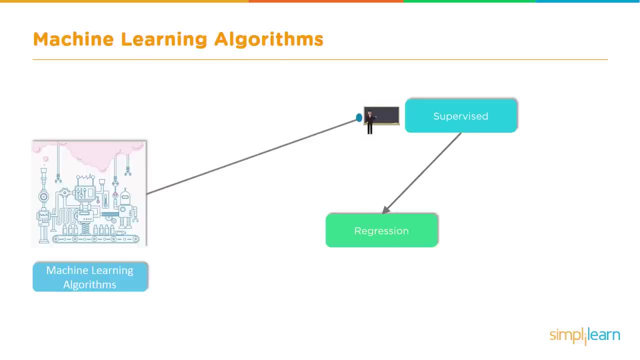 regression. so we're just going to focus on the regression side. And in the regression we have simple linear regression, we have multiple linear regression and we have polynomial linear regression. Now, on these three, simple linear regression is the examples we've looked. 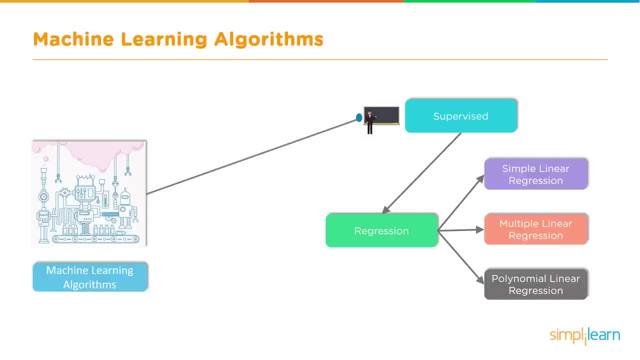 at so far where we have a lot of data and we draw a straight line through it. Multiple linear regression means we have multiple variables. Remember where we had the rainfall and the crops. We might add additional variables to that. We might add additional variables to. 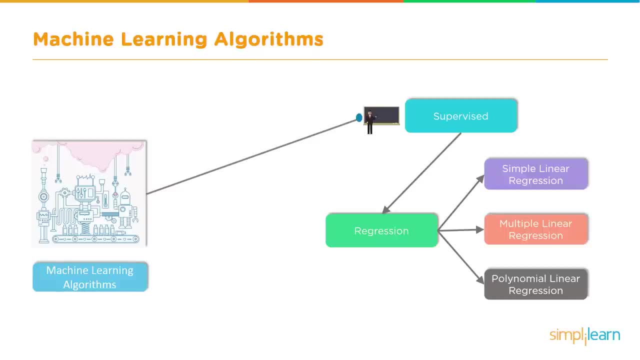 that We might add additional variables in there, like how much food do we give our crops, When do we harvest them. Those would be additional information added into our model And that's why it would be multiple linear regression. And finally we have polynomial linear regression. 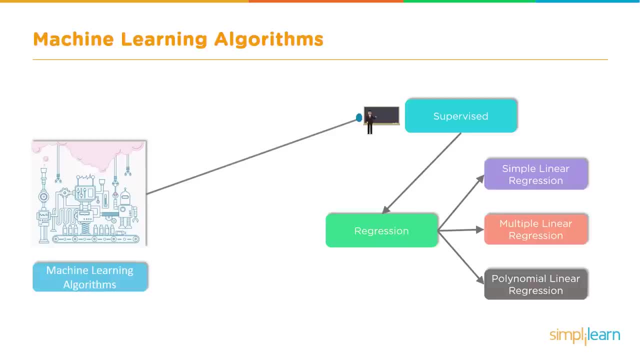 That is, instead of drawing a line, we can draw a curved line through it. Now that you see where regression model fits into the machine learning algorithms- and we're specifically looking at linear regression- let's go ahead and take a look at applications for linear. 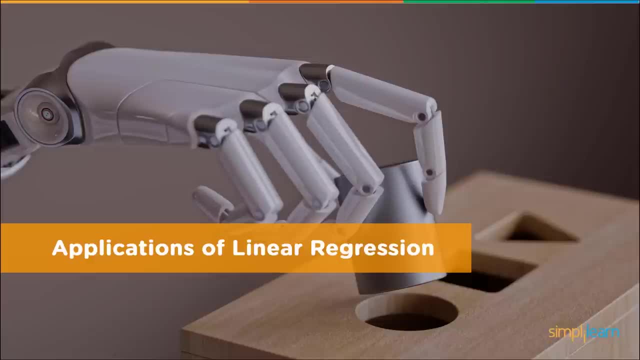 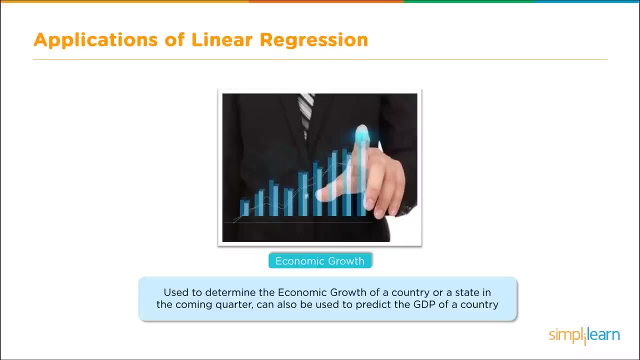 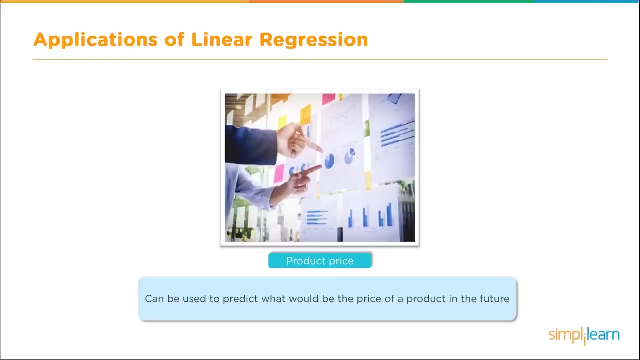 regression. Let's look at a few applications of linear regression. Economic growth Used to determine the economic growth of a country or a state in the coming quarter Can also be used to predict the GDP of a country. Product price Can be used to predict what would be the price of a product in the future. 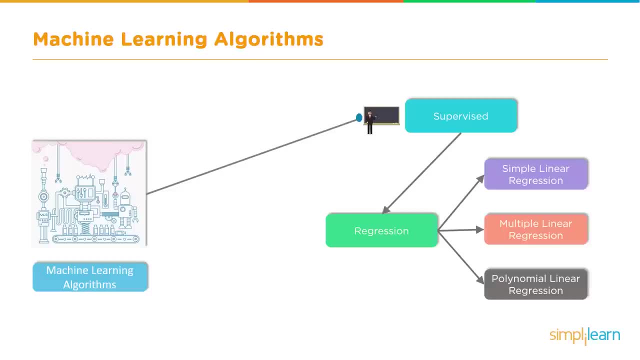 our model And that's why it would be multiple linear regression. And finally, we have polynomial linear regression, that is, instead of drawing a line, we can draw a curved line through it. Now that you see where a regression model fits into the machine learning algorithms- and we're specifically looking at linear 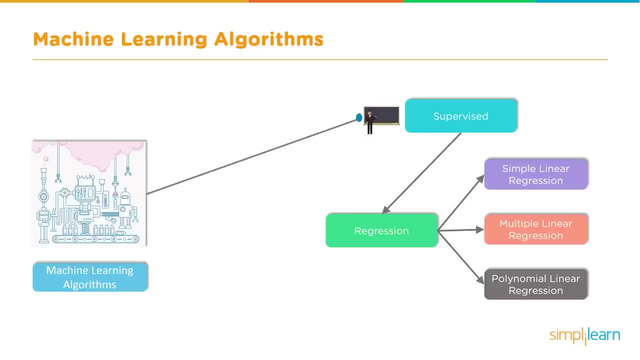 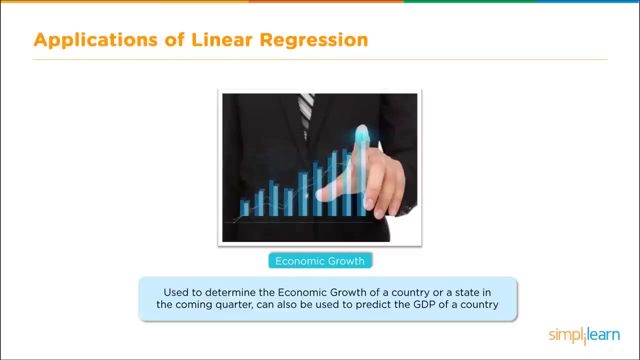 regression. let's go ahead and take a look at applications for linear regression. let's look at a few applications. implications of linear regression. Economic growth- used to determine the economic growth of a country or a state in the coming quarter, can also be used to predict the GDP of a country. 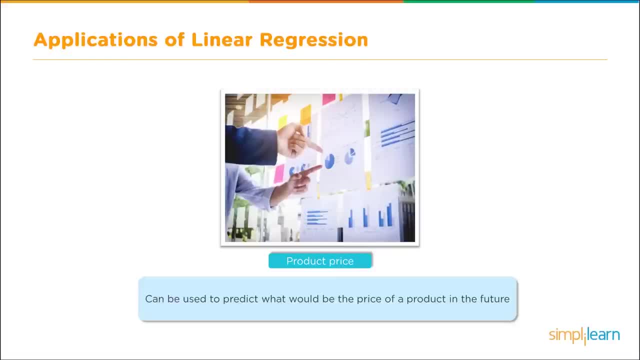 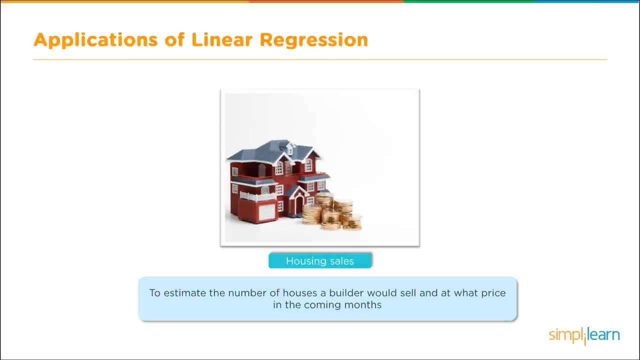 Product price can be used to predict what would be the price of a product in the future. We can guess whether it's going to go up or down. or should I buy today Housing sales to estimate the number of houses a builder would sell and what price in the coming months? Score predictions. 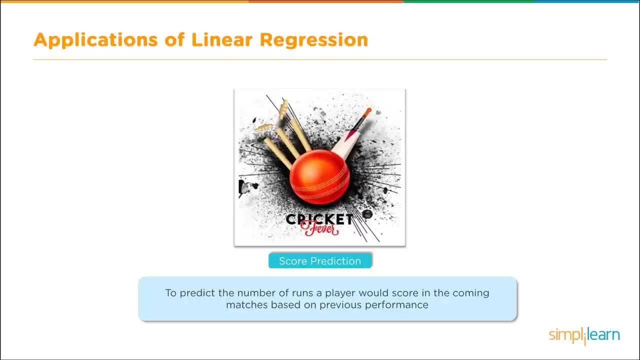 Cricket fever to predict the number of runs a player would score in the coming matches based on the previous performance. I'm sure you can figure out other applications you could use linear regression for. So let's jump in and let's understand linear regression and dig into the 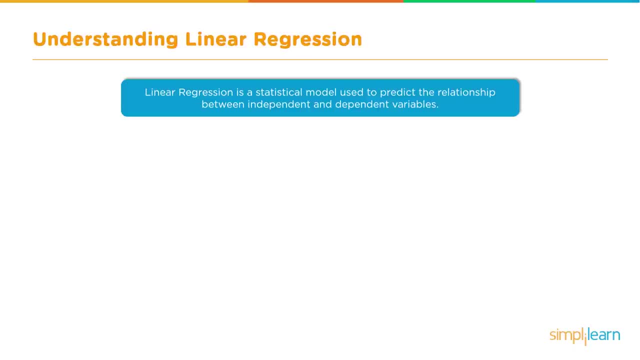 theory Understanding linear regression. Linear regression is the statistical model used to predict the relationship between independent and dependent variables by examining two factors. The first important one is which variables in particular are significant predictors of the outcome variable, And the second one that we need to look at closely is how significant is the regression line to make. 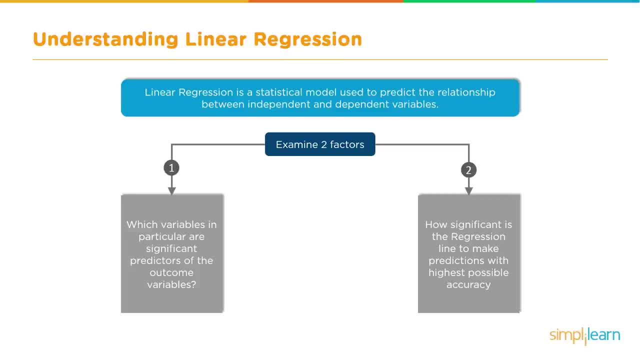 predictions with the highest possible accuracy. If it's inaccurate, we can't use it. So it's very important we find out the most accurate line we can get, Since linear regression is based on drawing a line through data. we're going to jump back and take a look at some 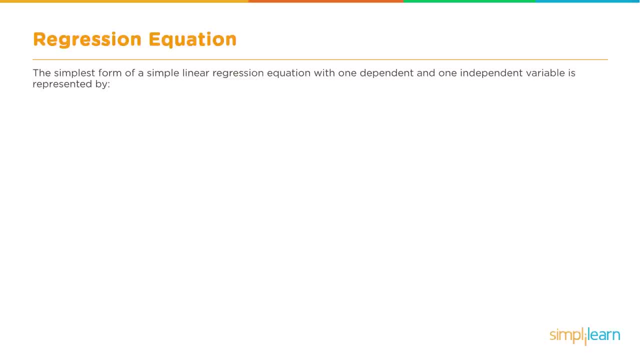 Euclidean geometry, The simplest form of a simple linear regression equation with one dependent and one independent variable, is represented by: y equals m times x plus c. And if you look at our model here, we plotted two points on here: x one and y one, x two and y two, Y been 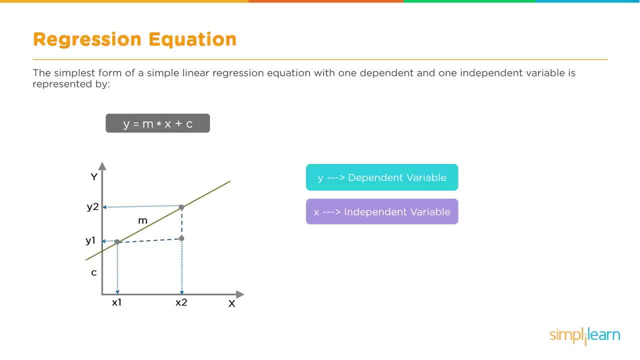 the dependent variable- remember that from before- and x being the independent variable. So y depends on whatever x is. m in this case is the slope of the line Where m equals the difference in the y2 minus y1, and x2 minus x1.. 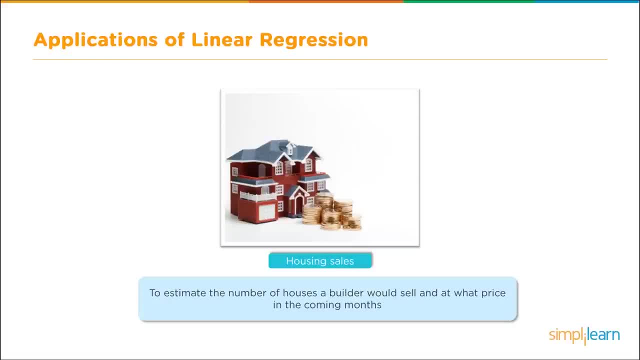 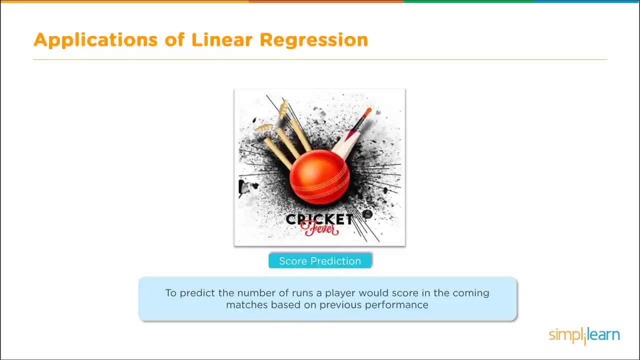 We can guess whether it's going to go up or down? or should I buy today? Housing sales To estimate the number of houses a builder would sell, and what price, in the coming months. Score predictions- Cricket fever: To predict the number of runs a player would score in. 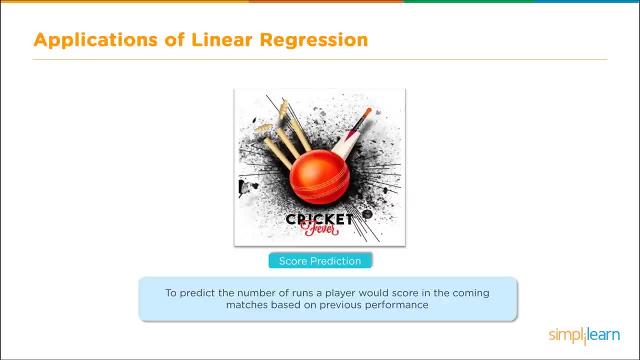 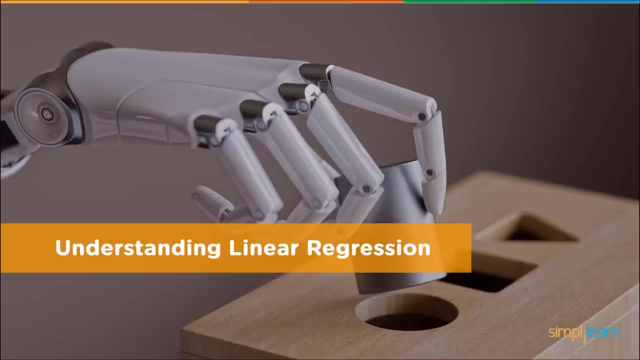 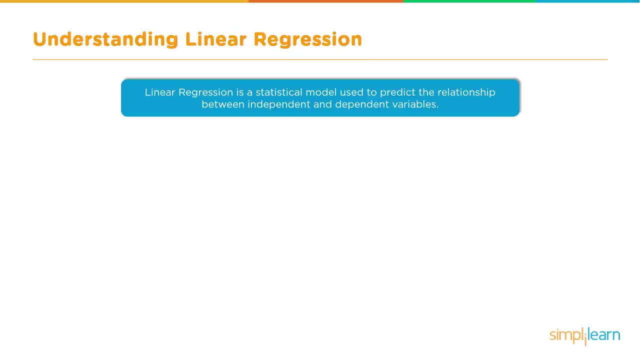 the coming matches based on the previous performance. I'm sure you can figure out other applications you could use linear regression for. So let's jump in and let's understand linear regression and dig into the theory Understanding Linear Regression. Linear regression is the statistical model used to predict the 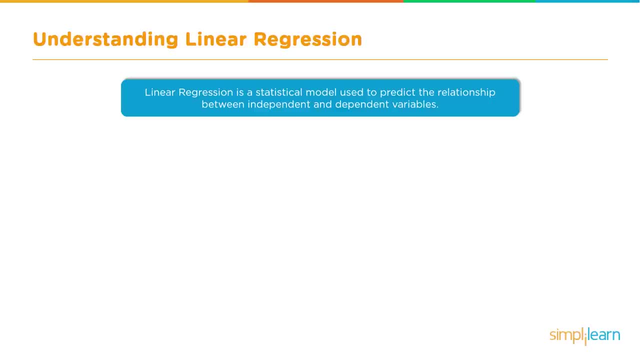 relationship between independent and dependent variables by examining two factors. The first important one is which variables in particular are significant predictors of the outcome variable that we need to look at closely is how significant is the regression line to make predictions with the highest possible accuracy? If it's inaccurate, we can't use it, so it's very. 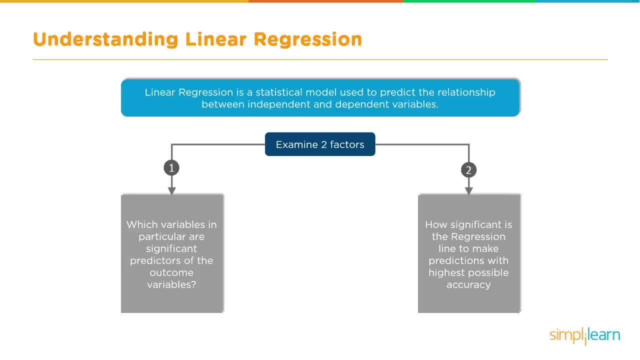 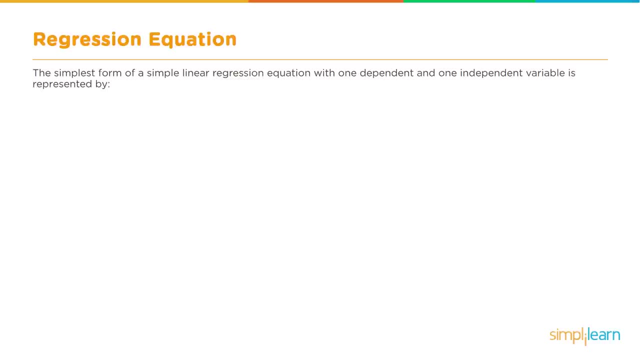 important we find out the most accurate line we can get. Since linear regression is based on drawing a line through data, we're going to jump back and take a look at some Euclidean geometry, The simplest form of a simple linear regression equation with one dependent and 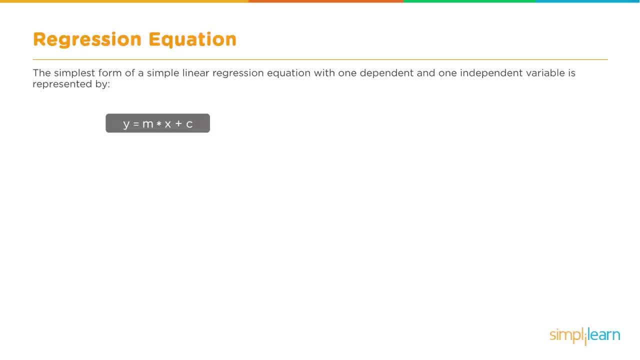 one independent variable is represented by: y equals m times x plus c. If you look at our model here, we plotted two points on here: x1 and y1,, x2 and y2, y being the dependent variable- remember that from before- and x being the independent variable. So y depends. 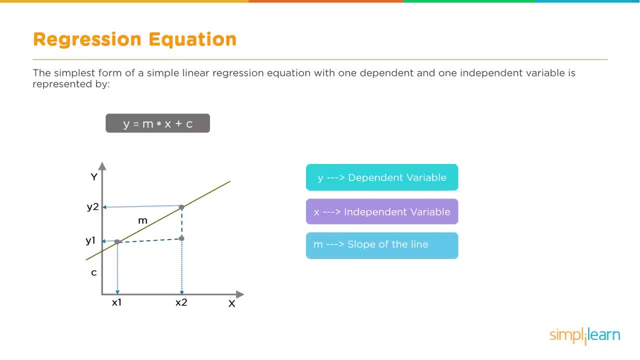 on whatever x is. m, in this case, is the slope of the line, where m equals the difference in the y2 minus y2.. y1 and x2 minus x1.. And finally we have c, which is the coefficient of the line, or. 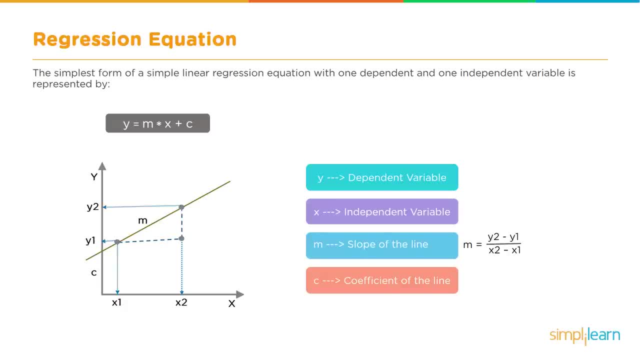 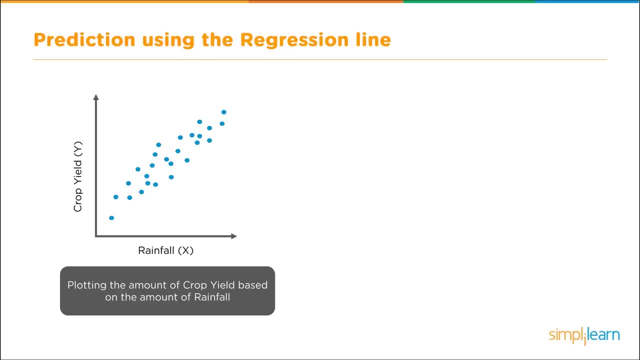 where it happens to cross the zero axes. Let's go back and look at an example we used earlier of linear regression. We're going to go back to plotting the amount of crop yield based on the amount of rainfall, And here we have our rainfall. Remember, we cannot change rainfall. 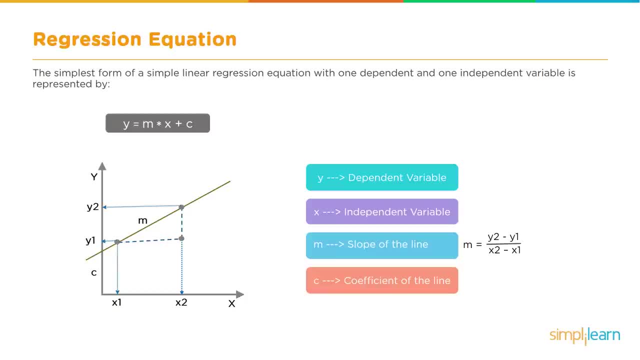 And finally we have c, which is the coefficient of the line, or where it happens to cross the zero axes. Let's go back and look at an example we used earlier of linear regression. We're going to go back to plotting the amount of crop yield. 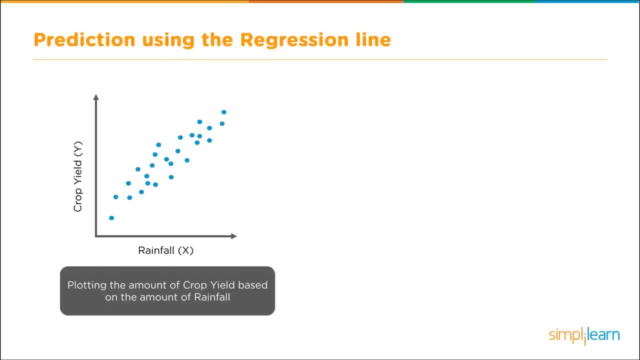 based on the amount of rainfall. And here we have our rainfall- Remember, we cannot change rainfall- And we have our crop yield, which is dependent on the rainfall. So we have our independent and our dependent variables. We're going to take this and draw a line through it. 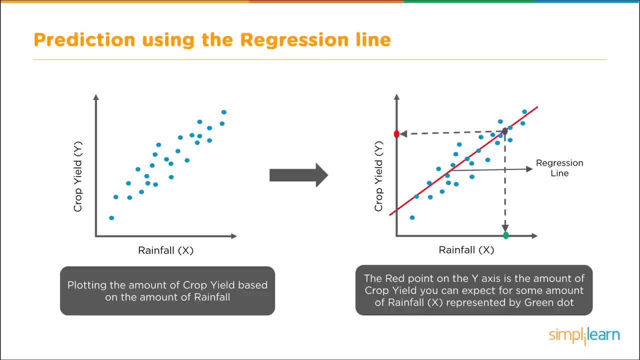 as best we can through the middle of the data And then we look at that, we put the red point on the y-axis is the amount of crop yield you can expect for the amount of rainfall represented by the green dot. So if we have an idea what the rainfall is for this year, 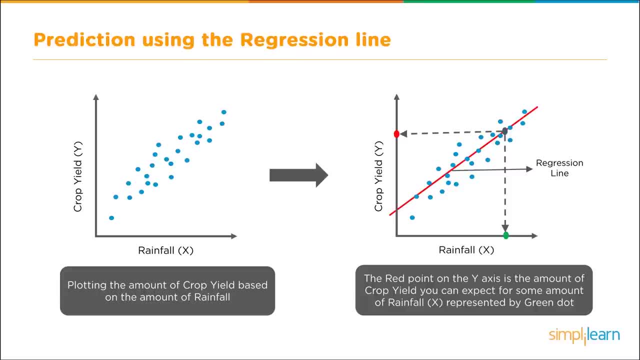 and what's going on. then we can guess how good our crops are going to be. And we've created a nice line right through the middle to give us a nice mathematical formula. Let's take a look and see what the math looks like behind the scenes. 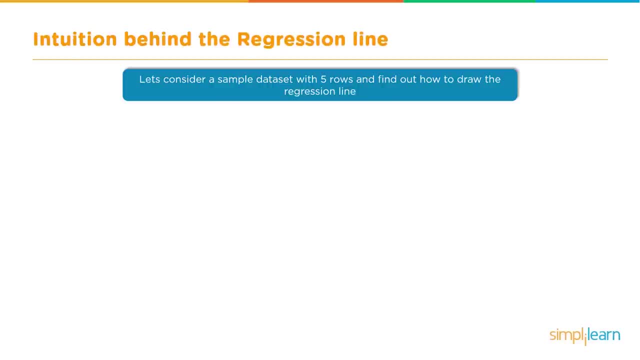 Let's look at the intuition behind the regression line. Now, before we dive into the math and the formulas that go behind this and what's going on behind the scenes, I want you to note that when we get into the case study and we actually apply some Python script, 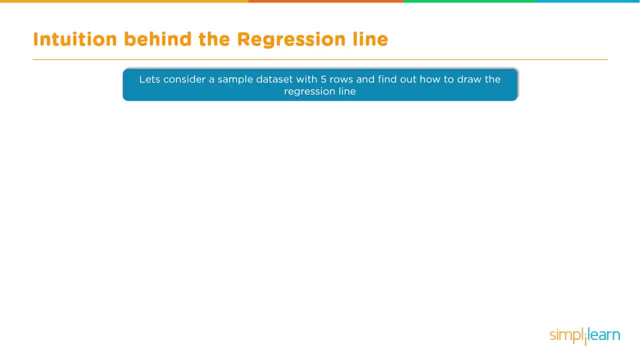 that this math that you're going to see here is already done automatically for you. You don't have to have it memorized. It is, however, good to have an idea what's going on, so if people reference the different terms, you'll know what they're talking about. 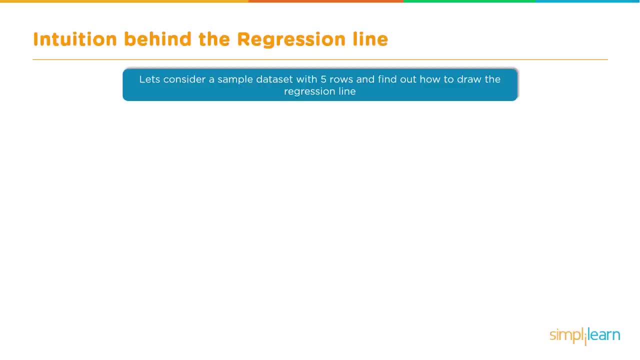 Let's consider a sample data set with five rows and find out how to draw the regression line. We're only going to do five rows because if we did like the rainfall, with hundreds of points of data, that would be very hard to see what's going on with the mathematics. 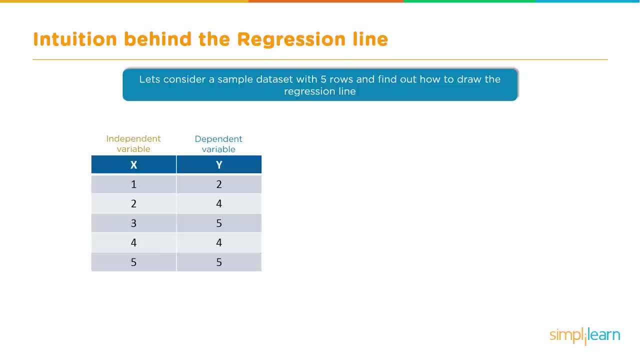 So we'll go ahead and create our own two sets of data and we have our independent variable x and our dependent variable y, And when x was one, we got y equals two. When x was two, y was four, and so on. 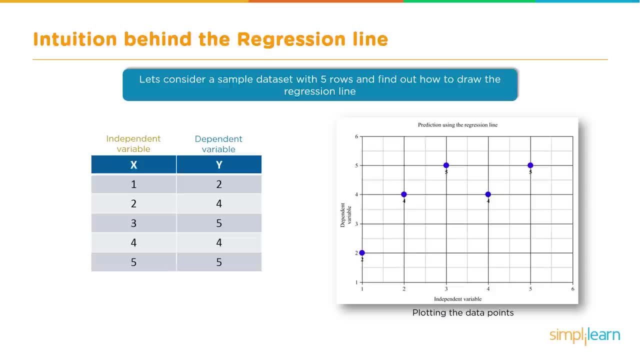 And so on and so on. If we go ahead and plot this data on a graph, we can see how it forms a nice line through the middle. You can see where it's kind of grouped, going upwards to the right. The next thing we want to know is what the means is. 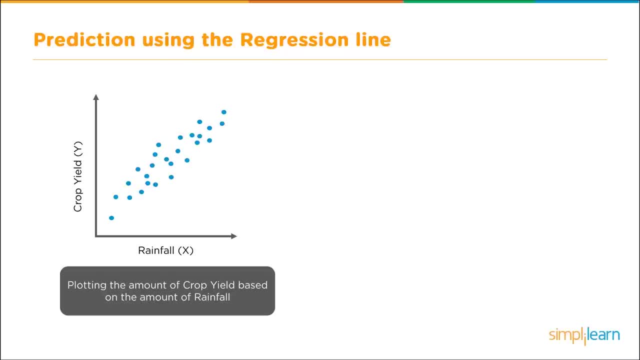 And we have our crop yield, which is dependent on the rainfall. So we have our independent and our dependent variables. We're going to take this and draw a line through it as best we can through the middle of the data, And then we look at that. we put the red point on the y-axis is the amount of crop. 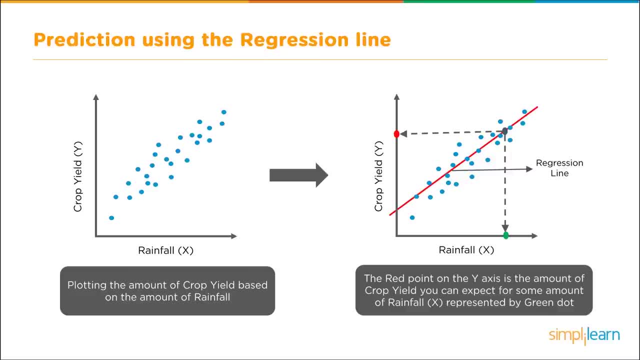 yield you can expect for the amount of rainfall represented by the green dot. So if we have an idea what the rainfall is for this year and what's going on, then we can guess how good our crops are going to be. And we've created a nice line right through the middle. 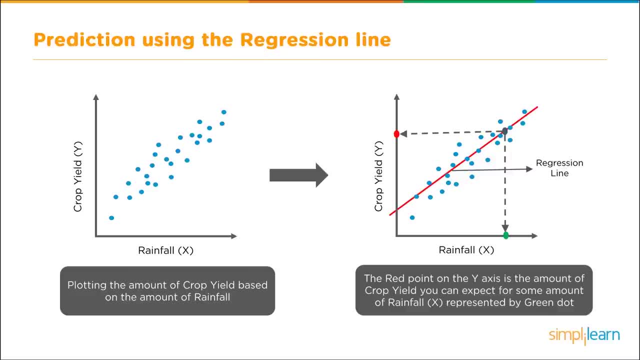 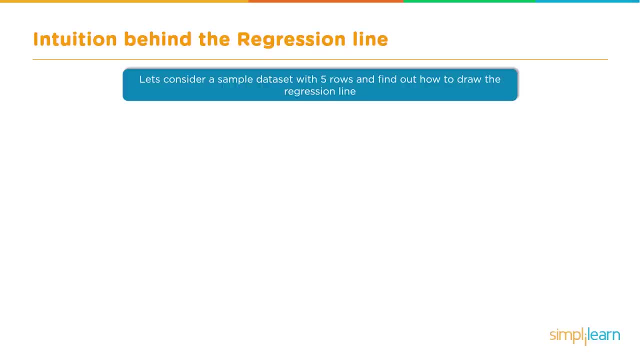 to give us a nice mathematical formula. Let's take a look and see what the math looks like behind this. Now, before we dive into the math and the formulas that go behind this and what's going on behind the scenes, I want you to note that when we get into the case study and we actually 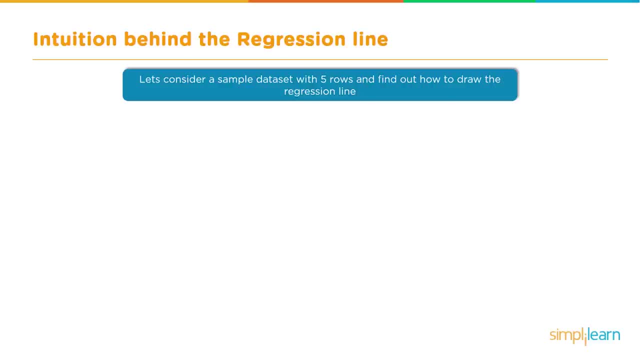 apply some Python script that this math that you're going to see here is already done automatically for you. You don't have to have it memorized. It is, however, good to have an idea what's going on, so if people reference the different terms, you'll know what they're talking about. 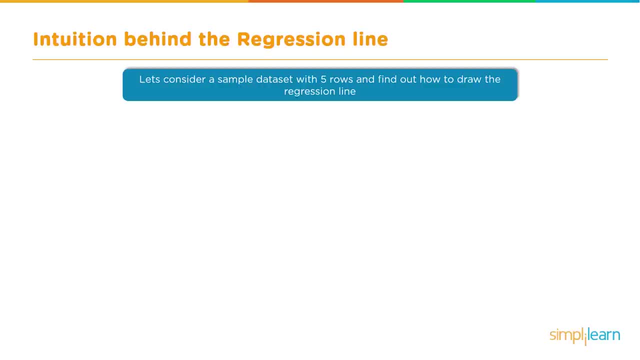 Let's consider a sample data set. Let's start with five rows and find out how to draw the regression line. We're only going to do five rows because if we did the rainfall with hundreds of points of data, that would be very hard to see what's going on with the mathematics. So we'll go ahead and create. 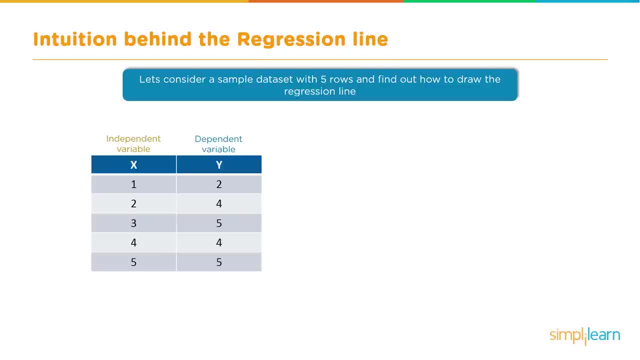 our own two sets of data And we have our independent variable, x, and our dependent variable, y. And when x was one, we got y equals two, When x was two, y was four, and so on and so on. If we go ahead and plot this data on a graph, we're going to be able to see what's going. 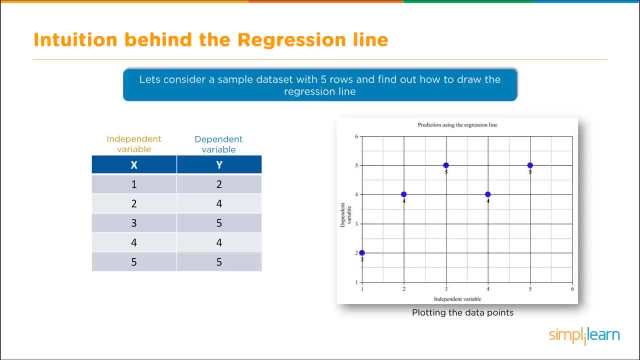 on in the graph We can see how it forms a nice line through the middle. You can see where it's kind of grouped, going upwards to the right. The next thing we want to know is what the means is of each of the data coming in: the x and the y. The means doesn't mean. 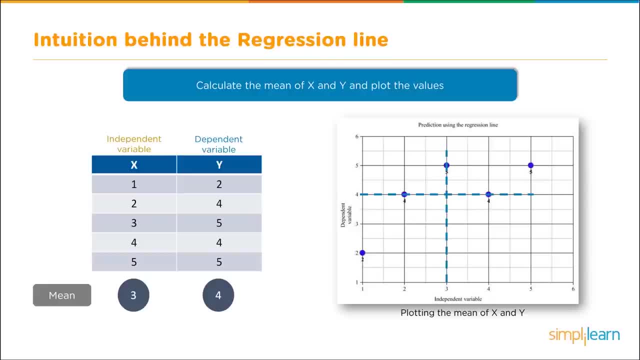 anything other than the average. So we add up all the numbers and divide by the total. So one plus two plus three plus four plus five over five equals three And the same for y: We get four. If we go ahead and plot the means on the graph, we'll see we get three. 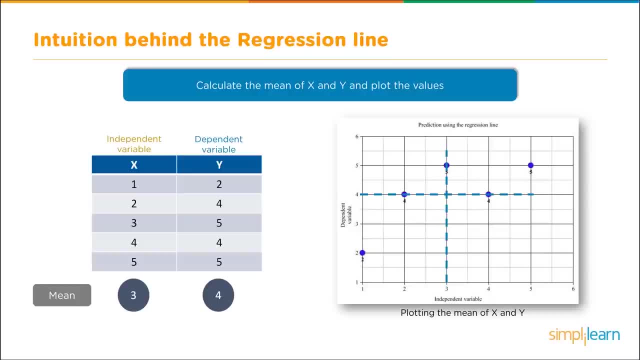 of each of the data coming in the x and the y. The means doesn't mean anything other than the average. So we add up all the numbers and divide by the total. So one plus two plus three plus four plus five over five equals three. 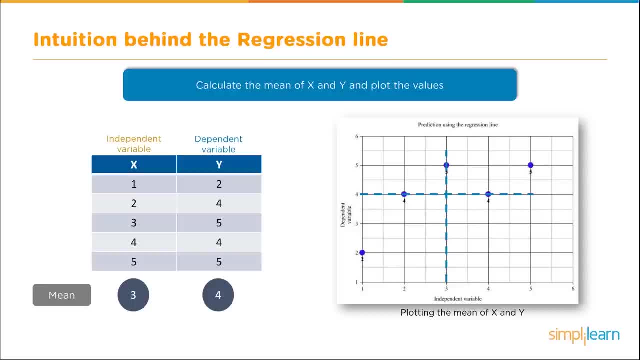 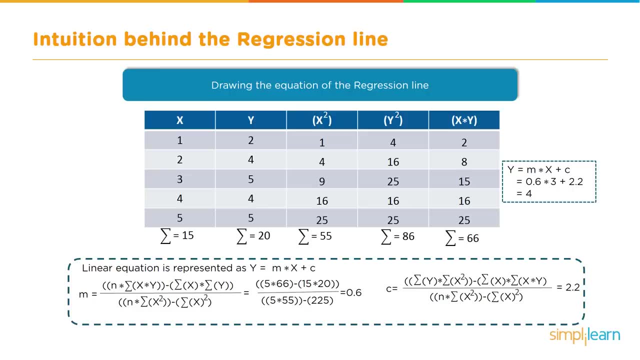 And the same for y, we get four. If we go ahead and plot the means on the graph, we'll see we get three comma four, which draws a nice line down the middle. a good estimate Here. we're gonna dig deeper into the math. 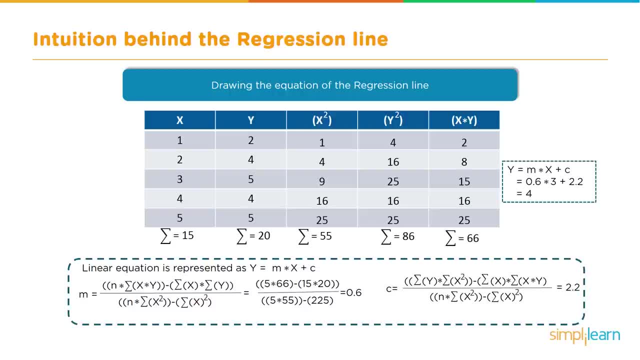 behind the regression line. Now remember before I said, you don't have to have all these formulas memorized or fully understand them, even though we're gonna go into a little more detail of how it works. And if you're not a math whiz, 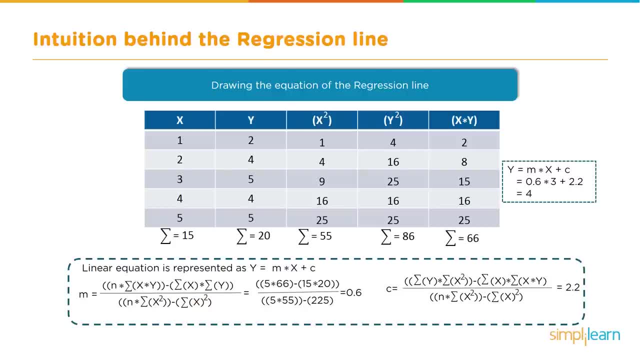 and you don't know if you've never seen the sigma character before, which looks a little bit like an e that's opened up. that just means summation, That's all that is. So when you see the sigma character, it just means we're adding everything in that row. 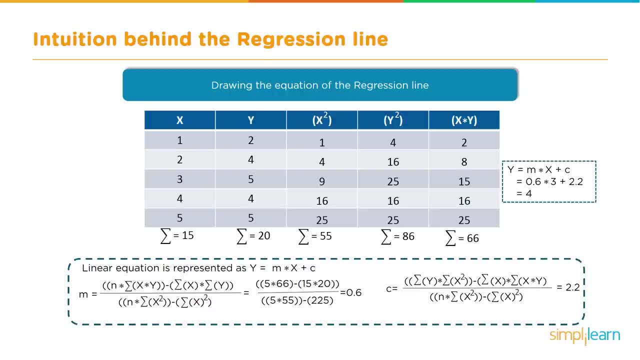 And for computers. this is great because as a programmer you can easily iterate through each of the xy points and create all the information you need. So in the top half you can see where we've broken that down into pieces and as it goes through the first two points. 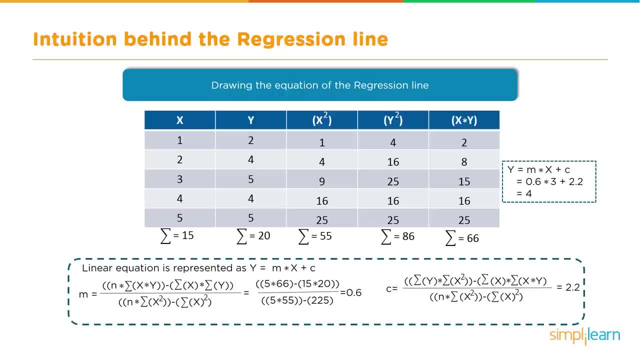 it computes the squared value of x, the squared value of y, and x times y, And then it takes all of x and adds them up, all of y adds them up, all of x squared adds them up, and so on, and so on. 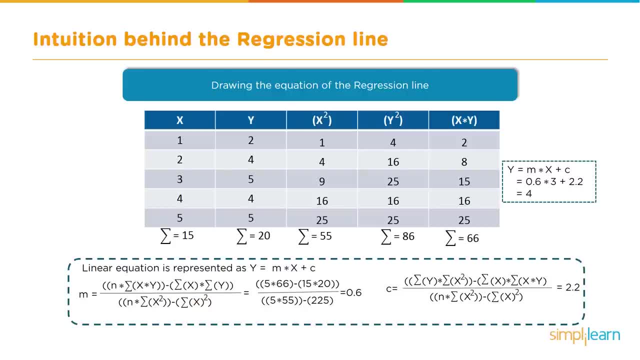 And you can see we have: the sum is equal to 15, the sum is equal to 20, all the way up to x times y, where the sum equals 66. This all comes from our formula for calculating a straight line where y equals the slope times x plus the coefficient c. 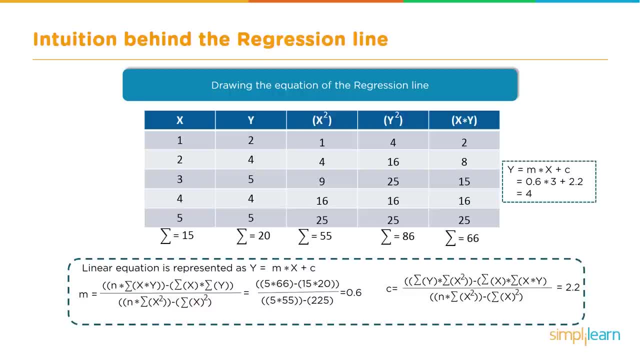 So we go down below and we're gonna compute more like the averages of these and we're gonna explain exactly what that is in just a minute and where that information comes from. It's called the square means error, But we'll go into that in detail. 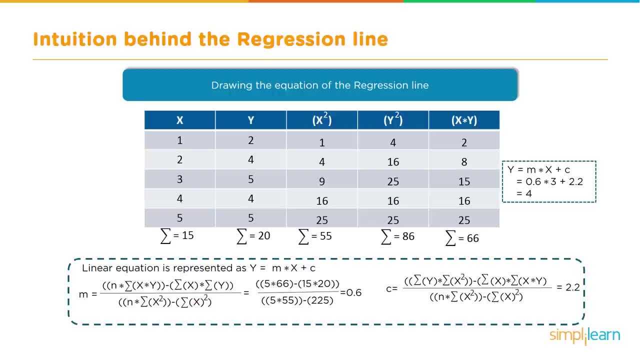 in just a minute. All you need to do is look at the formula and see how we've gone about computing it line by line, instead of trying to have a huge set of numbers pushed into it, And down here you'll see where the slope m equals. 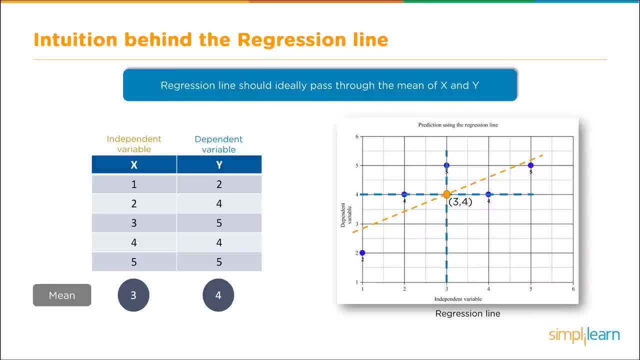 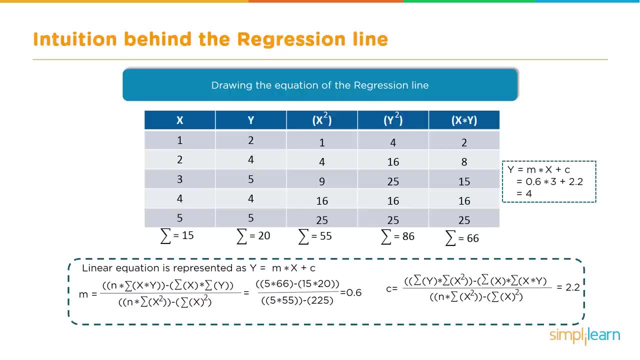 minus four, which draws a nice line down the middle Good estimate. Here we're going to dig deeper into the math behind the regression line. Now remember before I said you don't have to have all these formulas memorized or fully understand them, even though 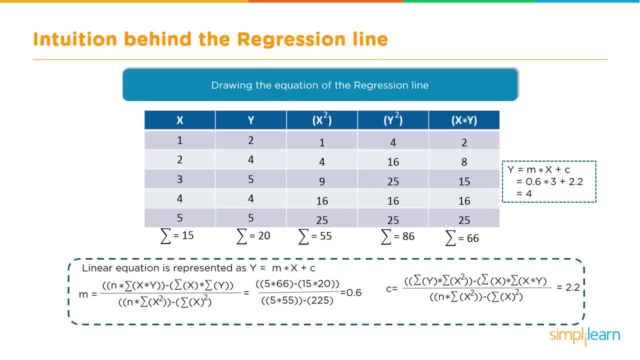 we're going to go into a little more detail of how it works. And if you're not a math wiz and you don't know, if you've never seen the sigma character before, which looks a little bit like an e that's opened up. that just means summation. That's all that is. 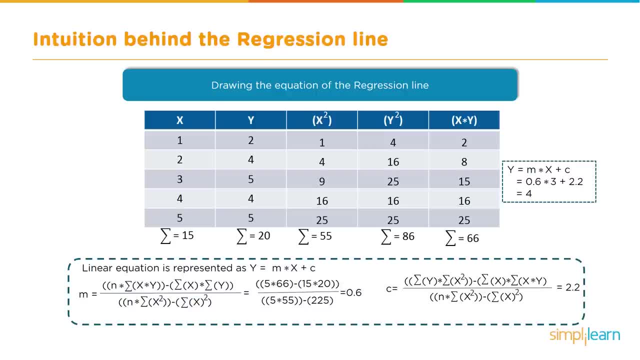 So when you see the sigma character, it just means we're adding up the numbers. Now let's just remember the units in front of that unit. Now, when you look at those units, the units adding everything in that row, And for computers this is great because as a programmer you can. 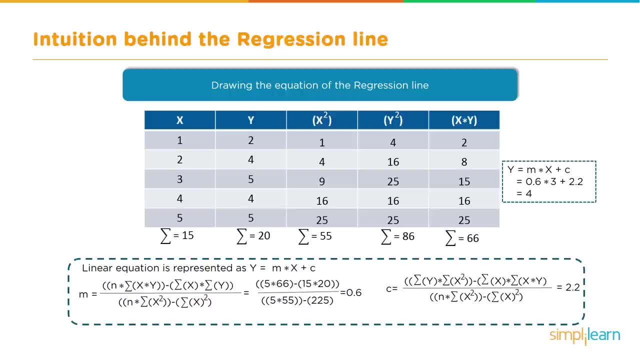 easily iterate through each of the xy points and create all the information you need. So in the top half you can see where we've broken that down into pieces. and as it goes through the first two points it computes the squared value of x, the squared value of y and x times y, And then it 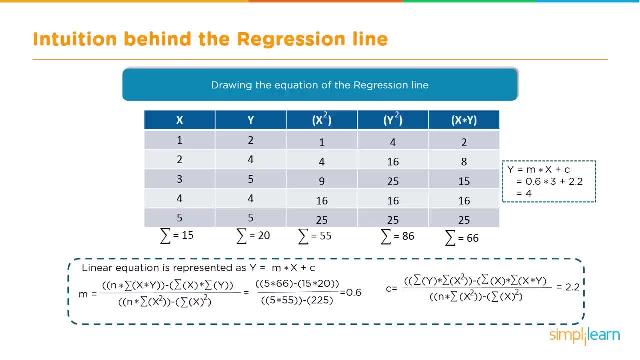 takes all of x and adds them up, all of y, adds them up, all of x squared, adds them up, and so on, and so on, And you can see we have the sum of equal to 15, the sum is equal to 20, all the way. 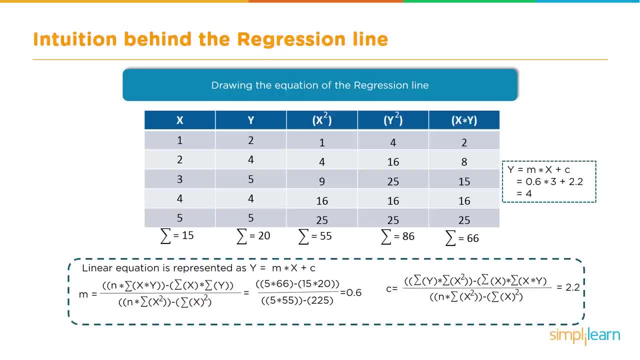 up to x times y, where the sum equals 66. This all comes from our formula for calculating a straight line where y equals the slope times x plus the coefficient c. So we go down below and we're going to compute more like the averages of these and we'll explain exactly what that is in just a 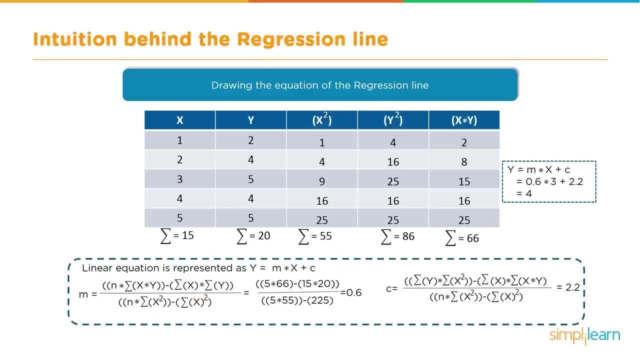 minute and where that information comes from is called the square means error, But we'll go into that in detail in a few minutes. All you need to do is look at the formula and see how we've gone about computing it line by line, instead of trying to 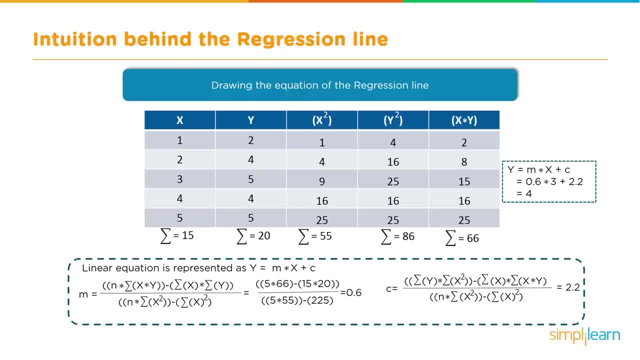 have a huge set of numbers pushed into it And down here you'll see where the slope m equals. and in the top part, if you read through the brackets, you have the number of data points times the sum of x times y, which we computed one line at a time there, and that's just the 66.. 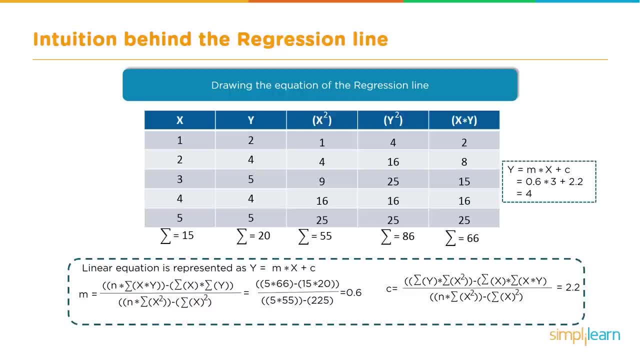 And take all that and you subtract it from the sum of x times the sum of y, and those have both been computed, So you have 15 times 20.. And on the bottom we have the number of lines times the sum of x squared, easily computed as 86. for the sum minus. I'll take all. 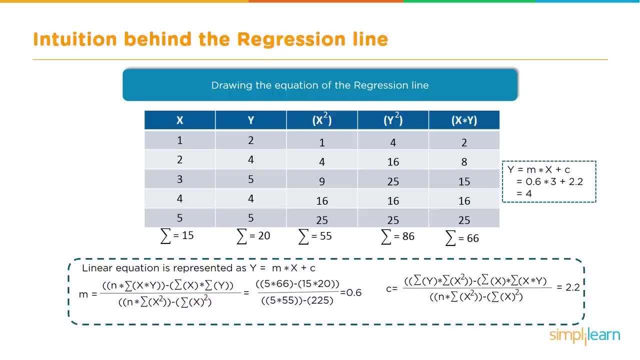 and in the top part, if you read through the brackets, you have the number of data points times the sum of x times y, which we computed one line at a time there, and that's just the 66. And take all that and you subtract it. 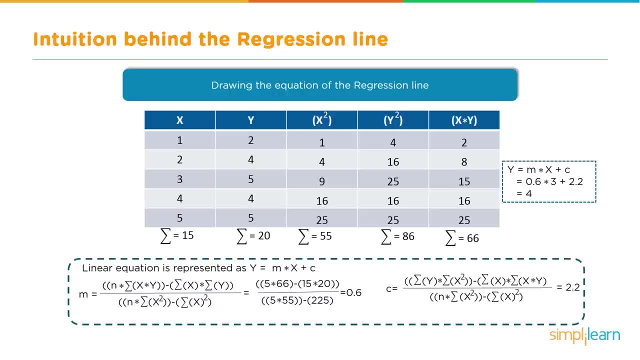 from the sum of x times y and you subtract it from the sum of x times the sum of y, And those have both been computed, So you have 15 times 20.. And on the bottom we have the number of lines times the sum of x squared, easily computed as 86. 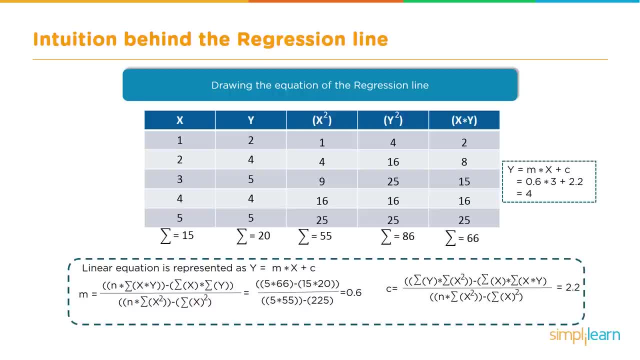 for the sum minus. I'll take all that and subtract the sum of x squared And we end up as we come across with our formula. you can plug in all those numbers, which is very easy to do on the computer. 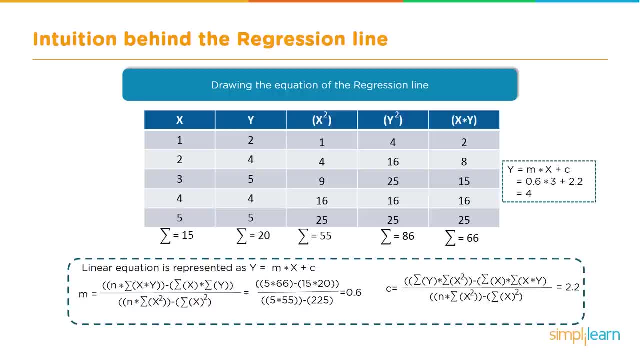 You don't have to do the math on a piece of paper or a calculator And you'll get a slope of .6, and you'll get your c coefficient. If you continue to follow through that formula, you'll see it comes out as equal to 2.2.. 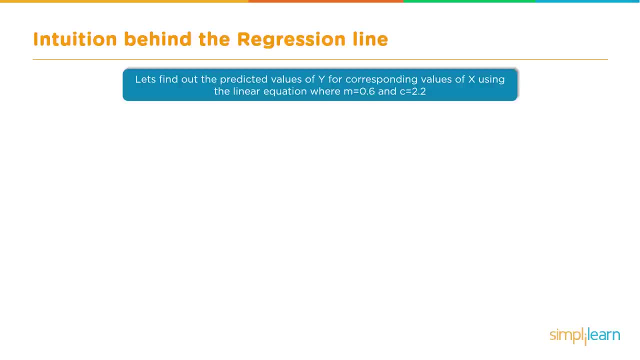 Continuing deeper into what's going behind the scenes, let's find out the predicted values of y for corresponding values of x using the linear equation where m equals .6, and c equals 2.2.. We're going to take these values. 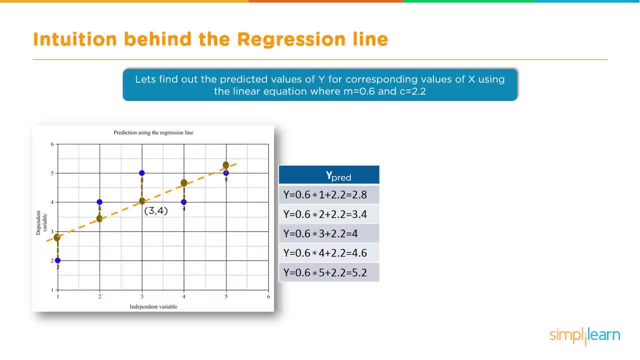 and we're going to go ahead and plot them, We're going to predict them. so y equals .6 times where x equals 1, plus 2.2 equals 2.8, so on and so on. And here the blue points, we're going to take them and we're 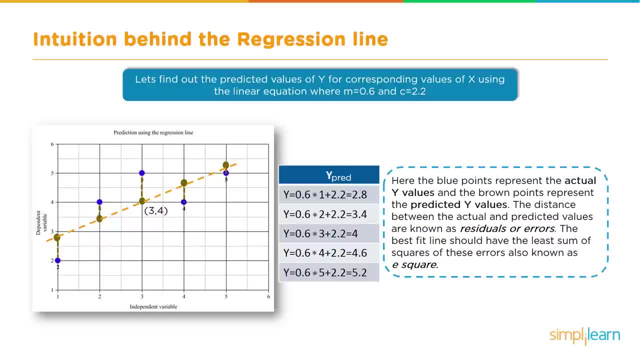 going to take these values and we're going to go ahead and plot them And we're going to predict them. so y equals .6 times, where x represent the actual y values and the brown points represent the predicted y values. based on the model we created, The distance between the actual and predicted values is known as. 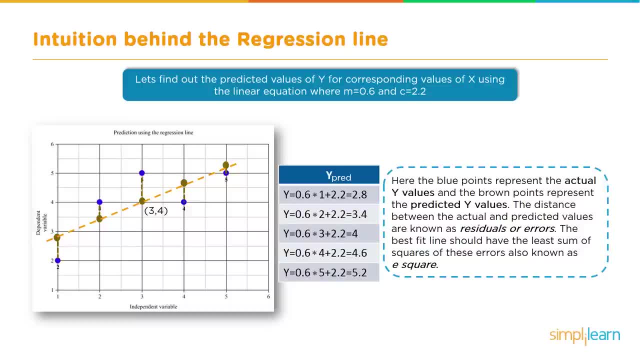 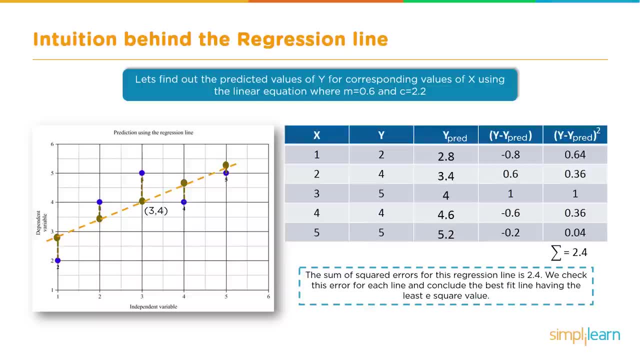 residuals or errors, The best fit line should have the least sum of squares of these errors, also known as e-square. If we put these into a nice chart where you can see x and you can see y, what the actual values were and you can see y predicted, you can easily see. 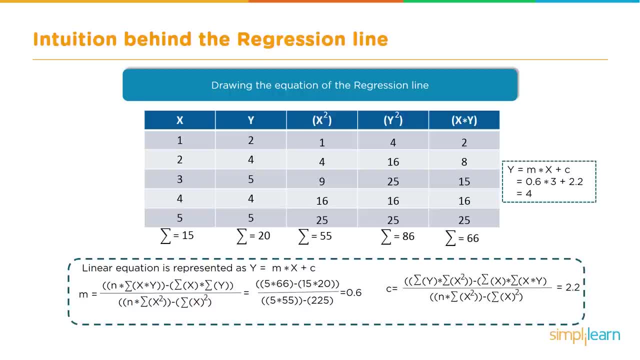 that and subtract the sum of x squared And we end up as we come across with our formula. you can plug in all those numbers, which is very easy to do on the computer- you don't have to do the math on a piece of paper or calculator- and you'll get a slope of 0.6.. And you'll get your c coefficient. 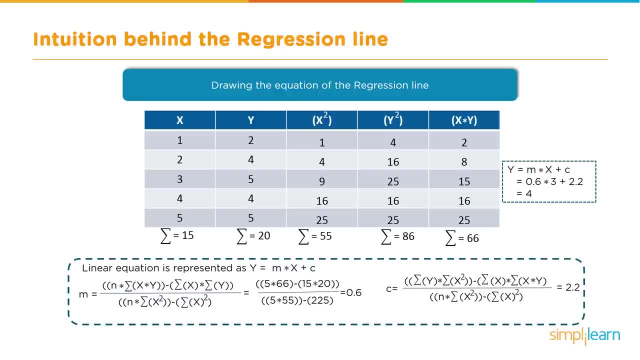 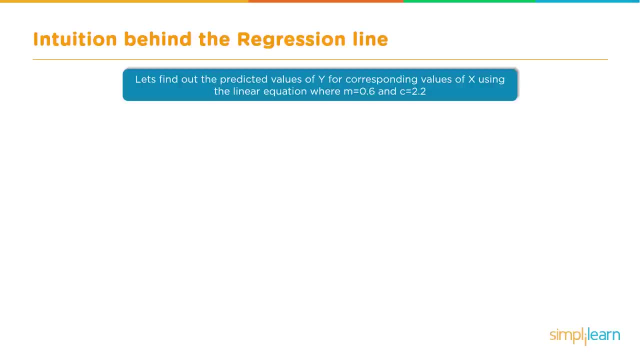 if you continue to follow through that formula, you'll see it comes out as equal to 2.2.. Continuing deeper into what's going behind the scenes, let's find out the predicted values of y for corresponding values of x using the linear equation, where m equals 0.6 and c equals 2.2.. 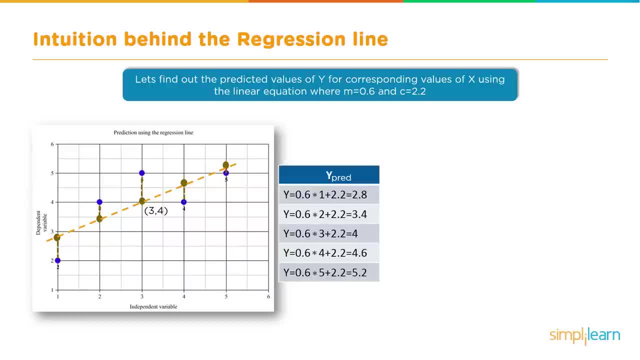 We're going to take these values and we're going to go ahead and plot them, We're going to predict them. so y equals 0.6 times where x equals 1, plus 2.2 equals 2.8, so on and so on. And here, 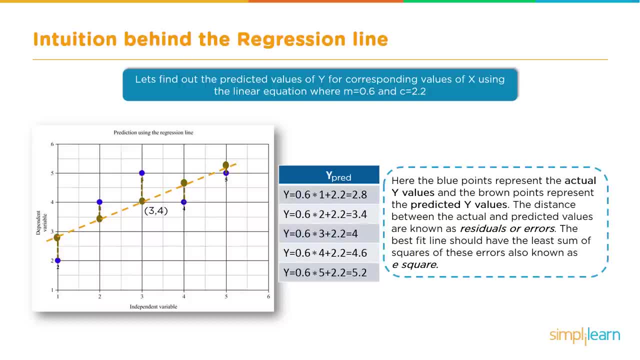 the blue points represent the actual y values and the brown points represent the predicted y values. based on the model we created, The distance between the actual predicted values is known as residuals or errors. The best fit line should have the least sum of squares of these errors, also known as e squared. If we put 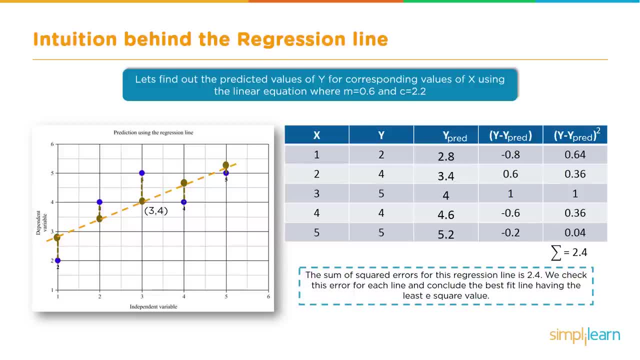 these into a nice chart where you can see x and you can see y- what the actual values were- and you can see y predicted. you can easily see where we take y minus y predicted and we get an answer. What is the difference between those two? And if we square that- y minus y, 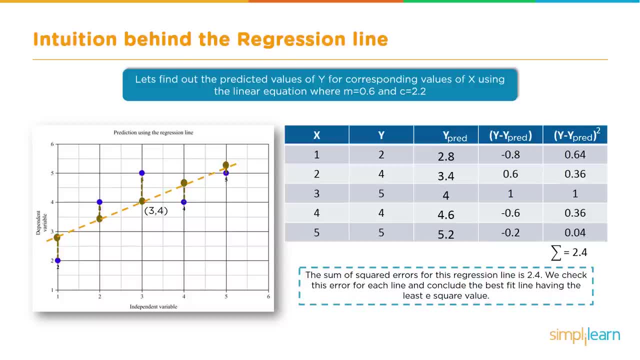 prediction squared, we can then sum those squared values. That's where we get the 0.64 plus the 0.36 plus 1, all the way down until we have a summation equals 2.4.. So the sum of squared errors for this 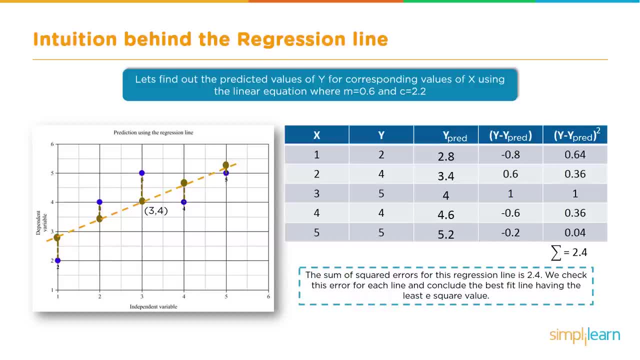 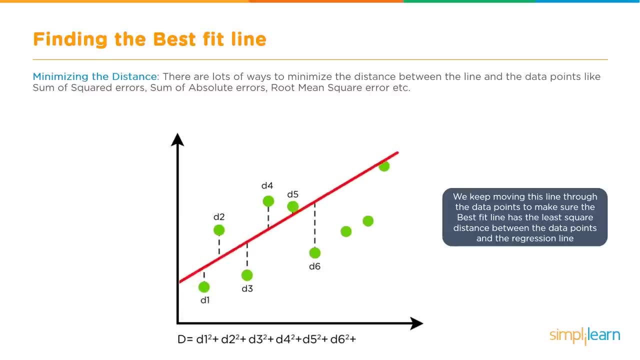 regression line is 2.4.. We check this error for each line and conclude the best fit line having the least e squared value In a nice graphical representation. we can see here where we keep moving this line and we can see that we have a sum of squares of this regression line and we can 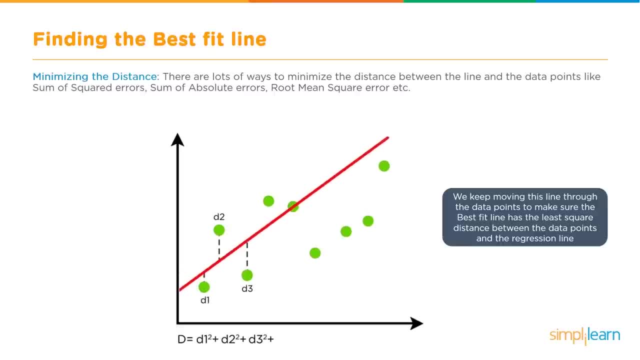 see here where we keep moving this line and we can see that we have a sum of squares of this regression line through the data points to make sure the best fit line has the least squared distance between the data points and the regression line. Now we only looked at the most commonly used formula for minimizing. 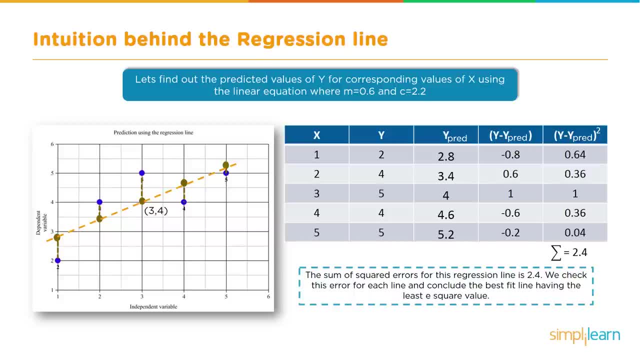 where we take y minus y predicted and we get an answer. What is the difference between those two? And if we square that y minus y prediction squared, we can then sum those squared values. That's where we get the .64 plus the .36 plus 1, all the way down until. 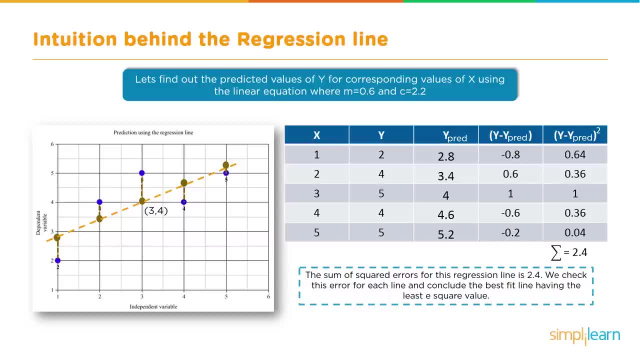 we have a summation equals 2.4.. So the sum of squared errors for this regression line is 2.4.. We check this error for each line and conclude the best fit line having the least e-square value In a nice graphical representation. 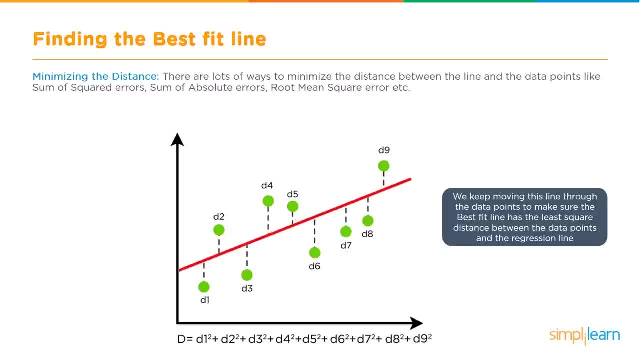 we can see here where we keep moving this line through the data points to make sure the best fit line has the least squared distance between the data points and the regression line. Now we only looked at the most commonly used formula for minimizing the distance. 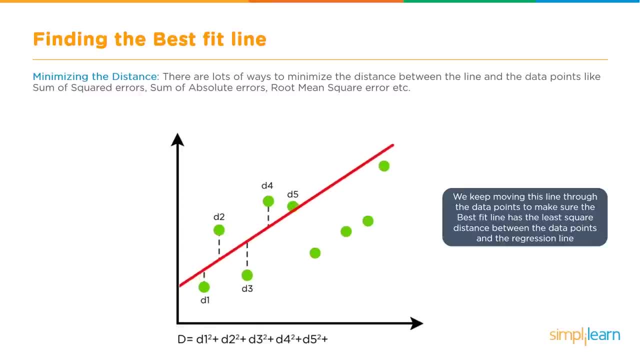 There are lots of ways to minimize the distance between the line and the data points, like sum of squared errors, sum of absolute errors, root mean, square error, etc. What you want to take away from this is: whatever formula is being used, you can use it to solve any. 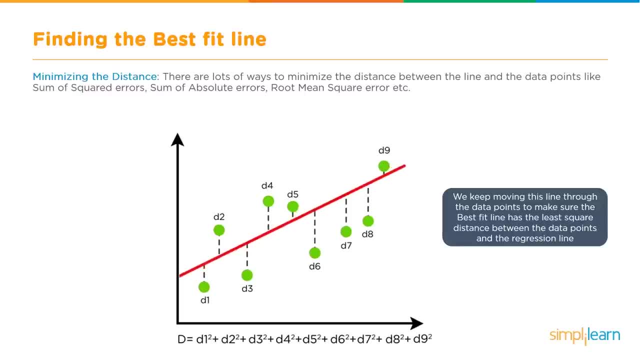 problem In the case of a computer. you can easily use a computer program and iterate through the data, calculate the different parts of it. That way these complicated formulas you see, with the different summations and absolute values, are easily computed one piece at a. 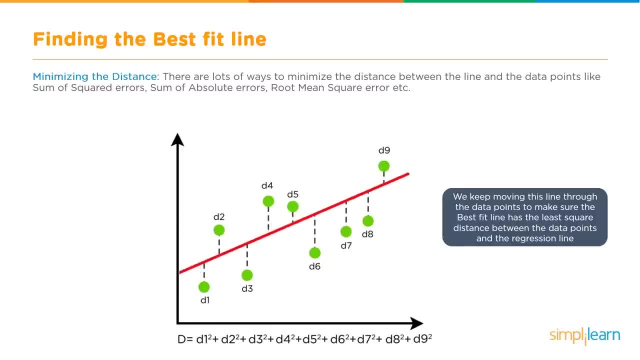 time. Up until this point, we've only been looking at two values: x and y. Well, in the real world, it's very rare that you only have two values when you're figuring out a solution. So let's move on to the next topic: multiple linear regression. Let's take a brief look. 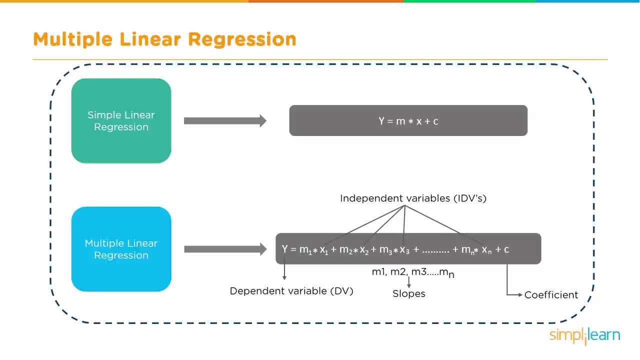 what happens when you have multiple inputs. So in multiple linear regression we have. well, we'll start with the simple linear regression where we had y equals m plus x plus c and we're trying to find the value of y. Now, with multiple linear regression, we have multiple variables coming in. 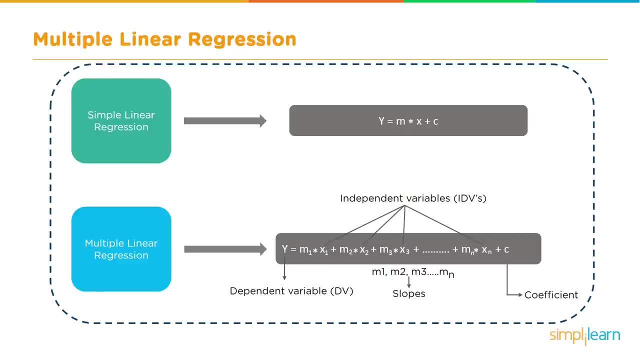 So instead of having just x, we have x1, x2, x3, and instead of having just one slope, each variable has its own slope attached to it. As you can see here we have m1, m2, m3 and we still just have the single coefficient. 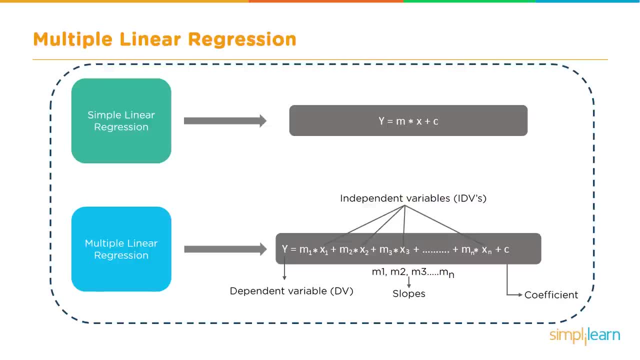 So when you're dealing with multiple linear regression, you basically take your single linear regression and you spread it out, So you have y equals m1 times x1 plus m2 times x2, so on all the way to m to the nth, x to the nth, and then you add your coefficient on there. 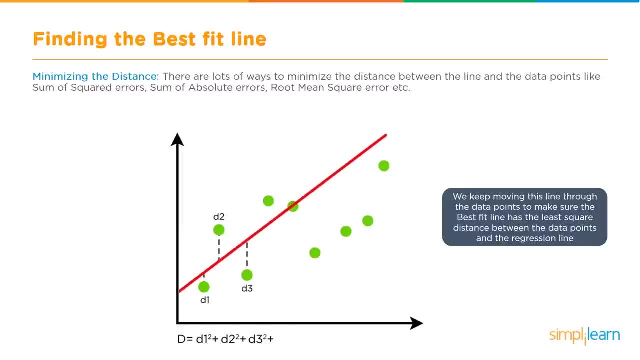 the distance. There are lots of ways to minimize the distance between the line and the data points, like sum of squared errors, sum of absolute errors, root mean, square error, etc. What you want to take away from this is: whatever formula is being used, you can easily using a computer program. 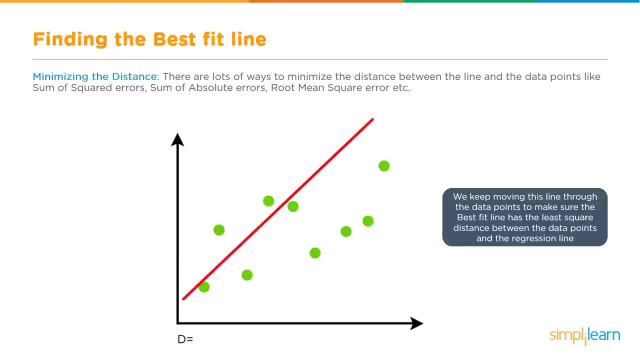 and, iterating through the data, calculate the different parts of it. That way, these complicated formulas you see, with the different summations and absolute values, are easily computed one piece at a time. Up until this point we've only been looking at two values, x and y. Well, in the real world it's very rare that. 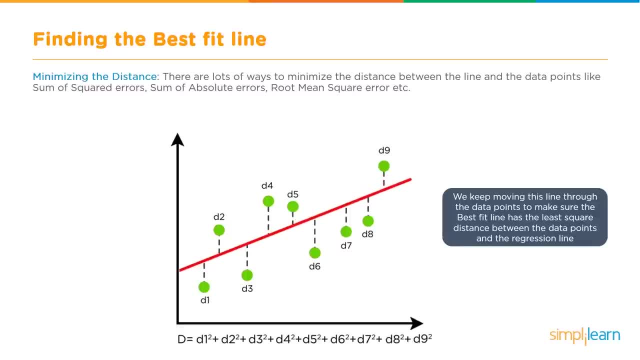 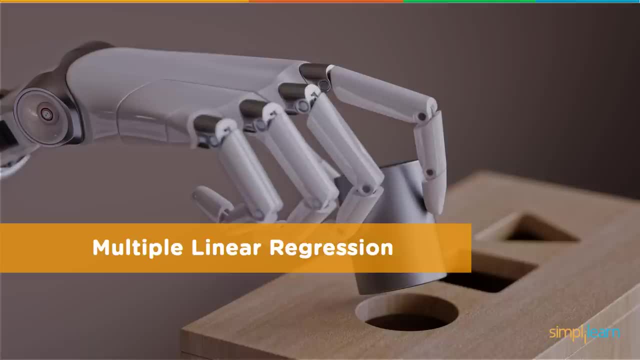 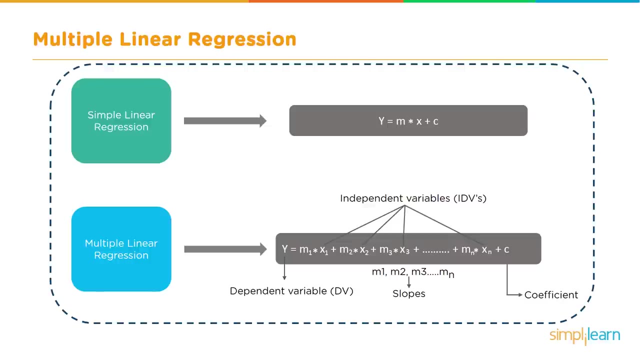 you only have two values when you're figuring out a solution. So let's move on to the next topic, multiple linear regression. Let's take a brief look at what happens when you have multiple inputs. So in multiple linear regression we'll start with the simple linear regression where we had y equals m plus x plus c. 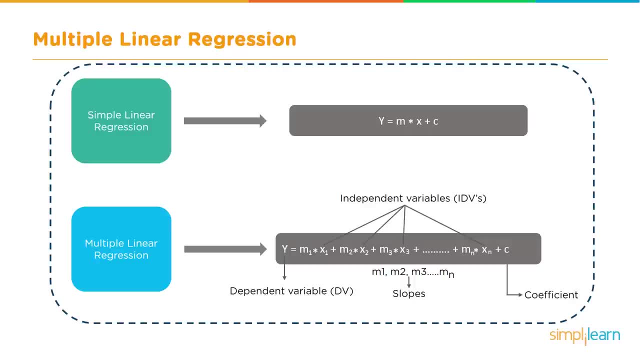 We're trying to find the value of y. Now, with multiple linear regression, we have multiple variables coming in. So instead of having just x, we have x1, x2, x3.. Instead of having just one slope, each variable has its own. 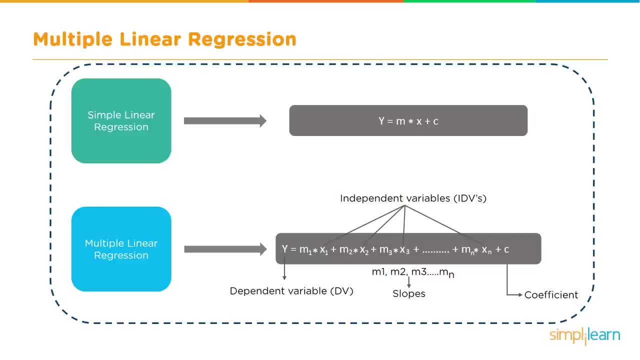 slope attached to it. As you can see, here we have m1, m2,, m3 and we still just have the single coefficient and all the other. So when you're dealing with multiple linear regression, you basically take your single linear regression and you spread it out. 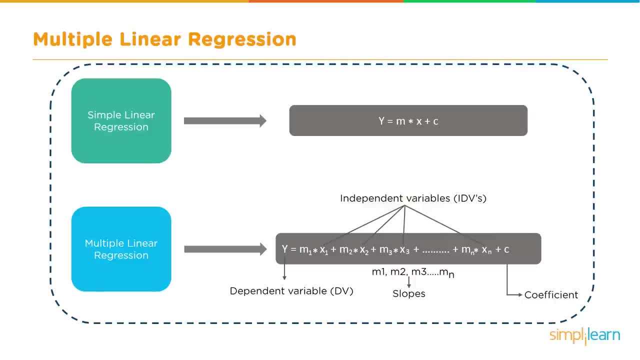 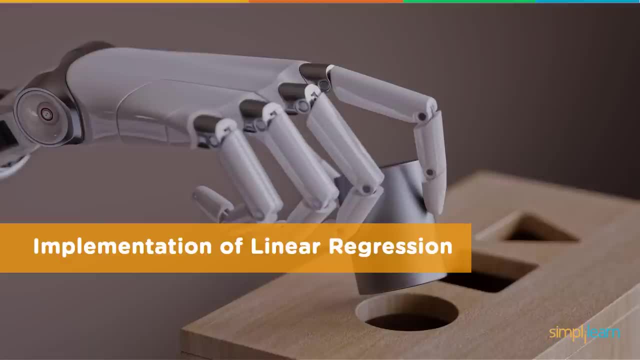 So you have: y equals m1 times x1 plus m2 times x2, so on all the way to m to the nth, x to the nth, and then you add your coefficient on there. Implementation of linear regression. Now we get into my favorite part. 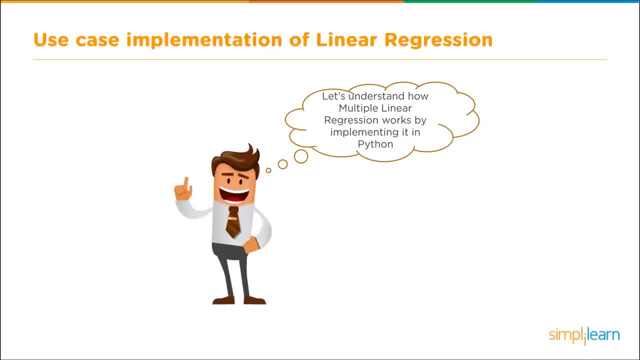 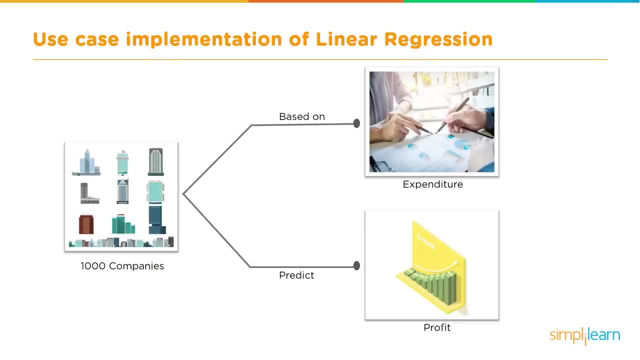 Let's understand how multiple linear regression works by implementing it in Python. If you remember, before we were looking at a company and, just based on its R&D, trying to figure out its profit. We're going to start looking at the expenditure of the company, we're going to go back to that and we're going to predict its profit. 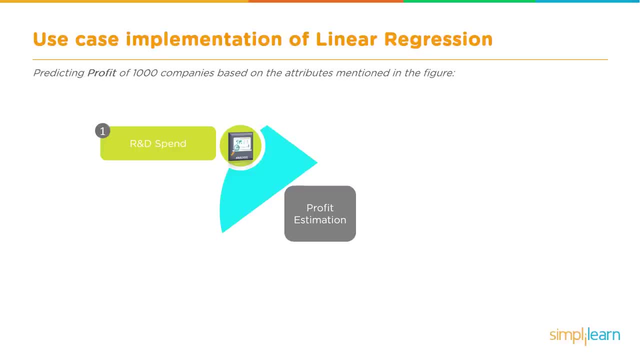 But instead of predicting it just on the R&D, we're going to look at other factors like administration costs, marketing costs and so on, And from there we're going to see if we can figure out what the profit of that company is going to be. 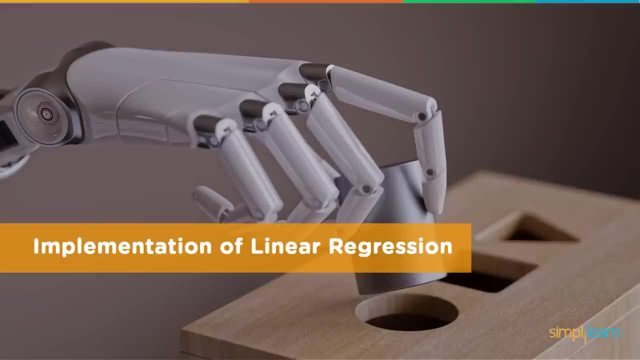 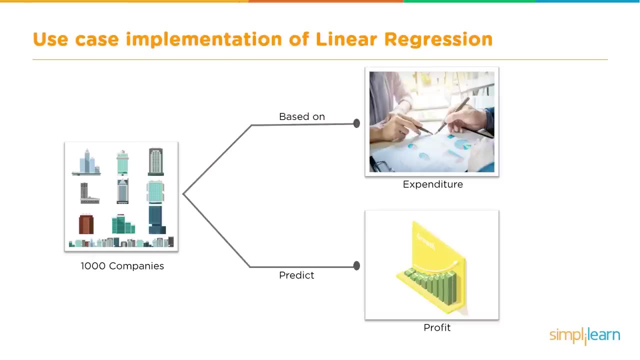 Implementation of linear regression. Now we get into my favorite part. Let's understand how multiple linear regression works by implementing it in python. If you remember, before we were looking at a company and, just based on its R&D, trying to figure out its profit. we're going to start looking at the 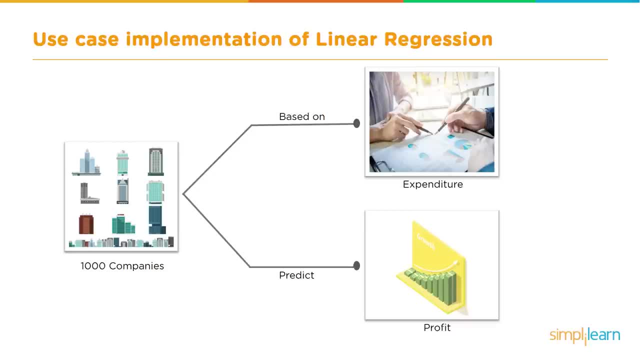 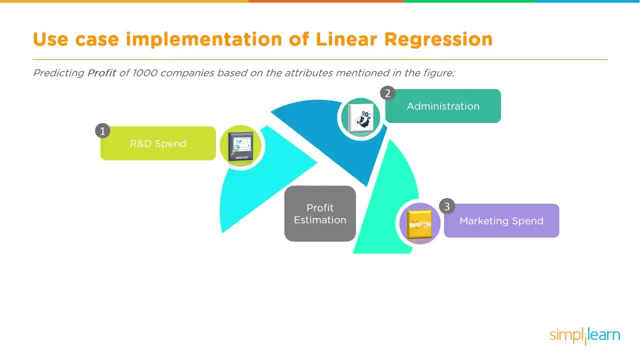 expenditure of the company. we're going to go back to that. we're going to predict its profit. but instead of predicting it just on the R&D, we're going to look at other factors like administration costs, marketing costs and so on, and from there we're going to see if we can figure out. 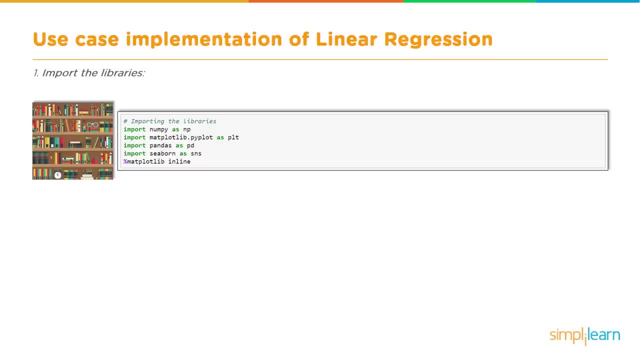 what the profit of that company is going to be. To start our coding, we're going to begin by importing some basic libraries and we're going to be looking through the data before we do any kind of linear regression. We're going to take a look at the data to 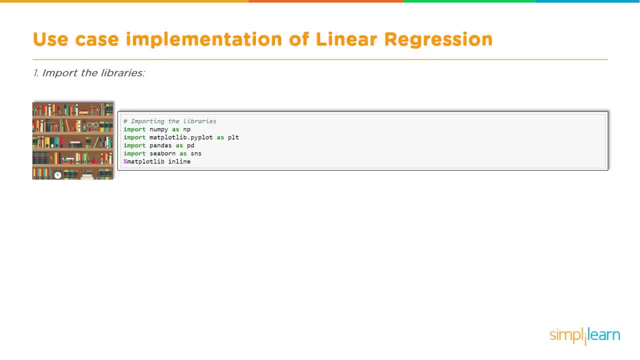 see what we're playing with. then we'll go ahead and format the data to the format we need to be able to run it in the linear regression model and then from there we'll go ahead and solve it and just see how valid our solution is. So let's start with importing the basic libraries. 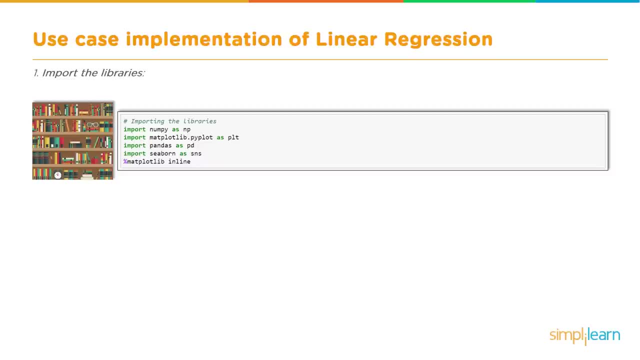 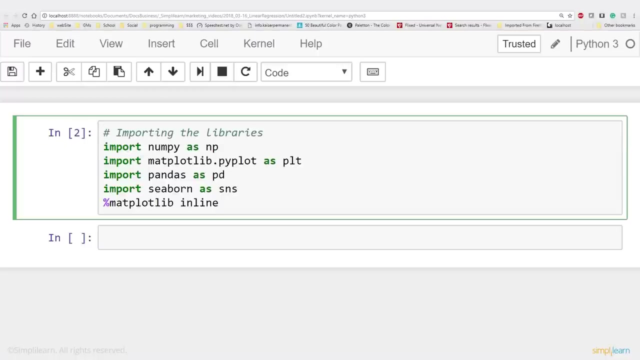 Now I'm going to be doing this in anaconda jupyter notebook, a very popular IDE. I enjoy it because it's such a visual to look at and so easy to use. Just any IDE for python will work just fine for this. So here we are in our jupyter notebook. let me go ahead and paste our 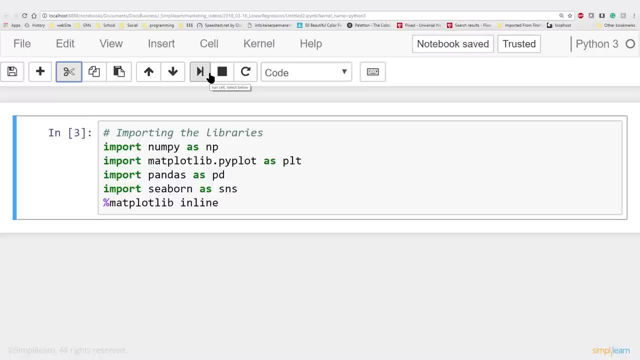 first piece of code in there and let's walk through what libraries we're importing. First we're going to import numpy as np and then I want you to skip one line and look at import pandas as pd. These are very common tools that you need with most of your linear regression. The numpy, which stands for number python. 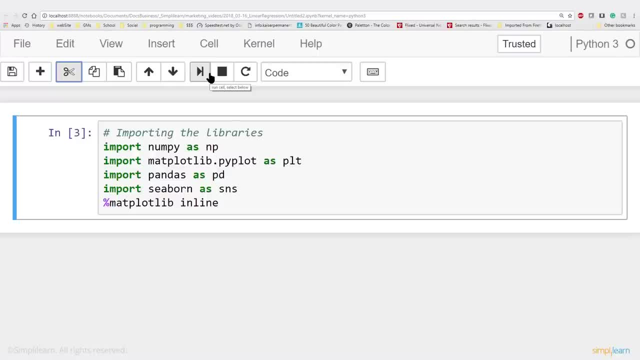 is usually denoted as np, and you have to almost have that for your sklearn toolbox, so you always import that right off the beginning. Pandas, although you don't have to have it for your sklearn libraries, it does such a wonderful job of importing data, setting it up into a data frame so we can manipulate it rather. 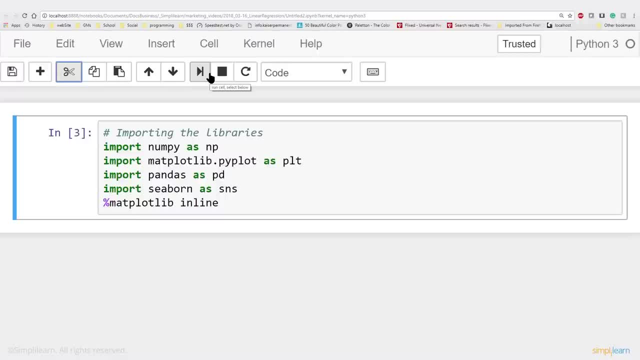 easily, and it has a lot of tools also in addition to that. So we usually like to use the pandas when we can, and I'll show you what that looks like. The other three lines are for us to get a visual of this data and take a look at it. So we're. 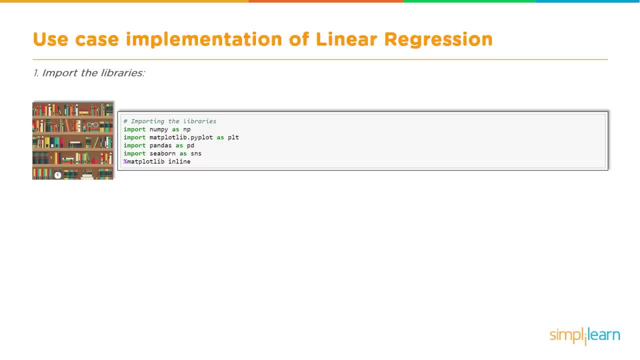 To start our coding. we're going to begin by importing some basic libraries And we're going to be looking Through the data before we do any kind of linear regression. we're going to take a look at the data to see what we're playing with. 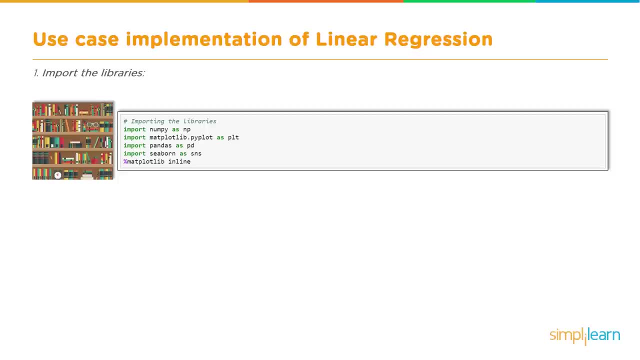 Then we'll go ahead and format the data to the format we need to be able to run it in the linear regression model, And then from there we'll go ahead and solve it and just see how valid our solution is. So let's start with importing the basic libraries. 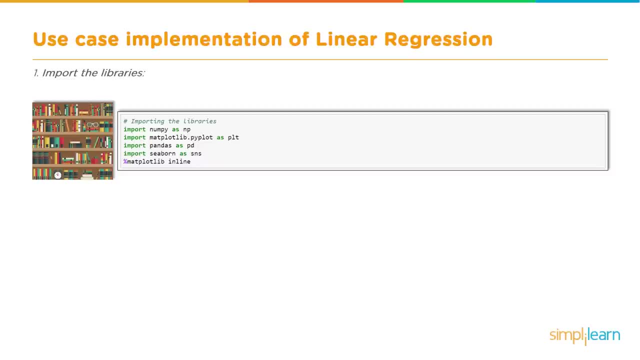 Now I'm going to be doing this in Anaconda Jupyter Notebook, a very popular IDE. I enjoy it because it's such a visual to look at and so easy to use. Just any IDE for Python will work Just fine for this. 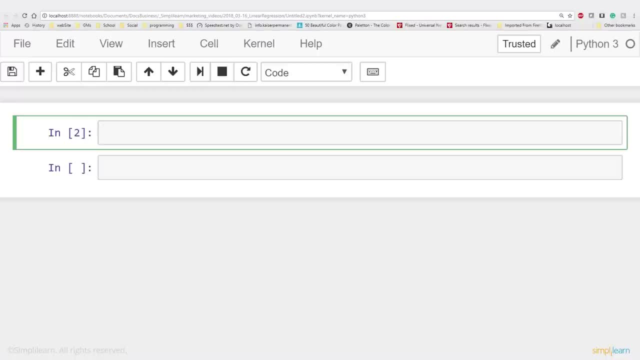 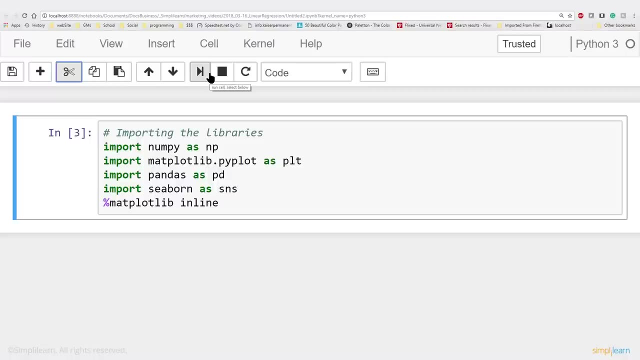 So break out your favorite Python IDE. So here we are in our Jupyter Notebook. Let me go ahead and paste our first piece of code in there And let's walk through what libraries we're importing. First we're going to import NumPy as np. 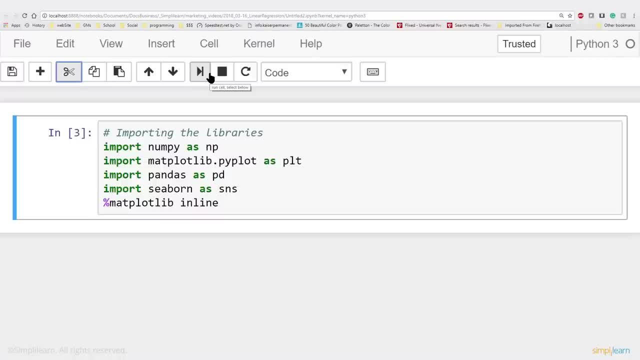 And then I want you to skip one line and look at import pandas as pd. These are very common tools that you need with most of your linear regression. The NumPy, which stands for number Python, is usually denoted as np, And you have to almost have that for your sklearn toolbox. 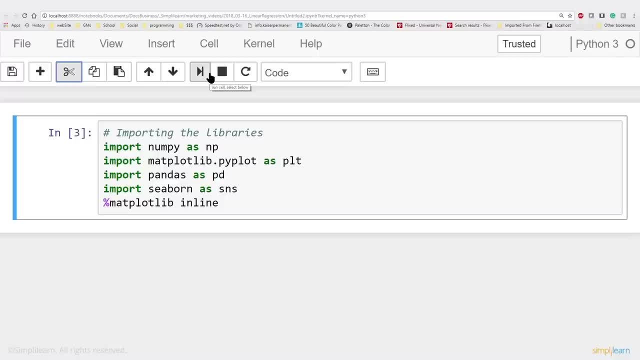 So you always import that right off Pandas, although you don't have to have it for your sklearn libraries. it does such a wonderful job of importing data, setting it up into a data frame so we can manipulate it rather easily, And it has a lot of tools also in addition to that. 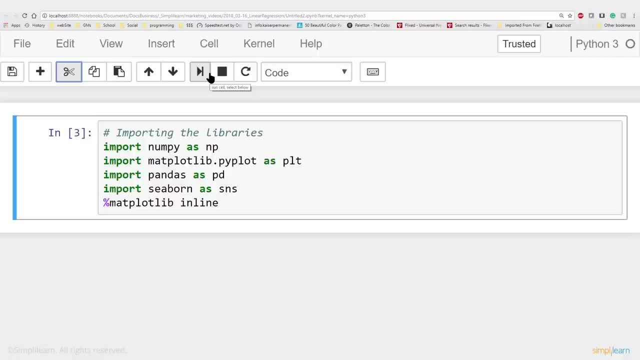 So we usually like to use the pandas when we can, And I'll show you what that looks like. The other three lines are for us to get a visual of this data and take a look at it. So we're going to import matplotlibrarypyplot as plt. 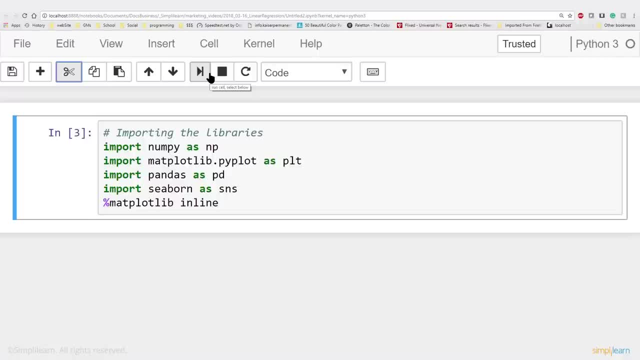 And then seaborn as sns. Seaborn works well. It's with the matplotlibrary, So you have to always import matplotlibrary and then seaborn sits on top of it And we'll take a look at what that looks like. You could use any of your own plotting libraries you want. 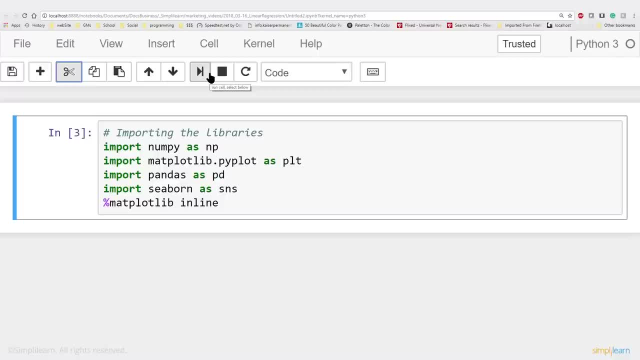 There's all kinds of ways to look at the data. These are just very common ones, And the seaborn is so easy to use that it just looks beautiful. It's a nice representation that you can actually take and show somebody. And the final line is the ambersign matplotlibrary inline. 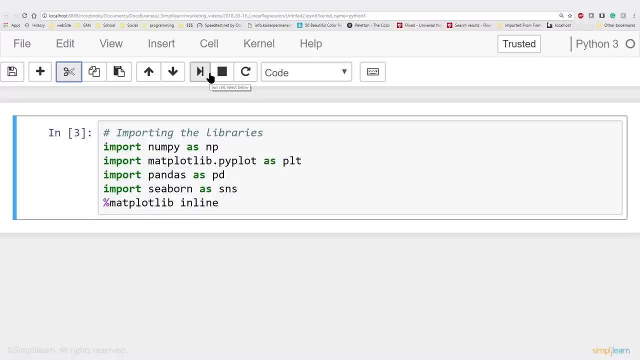 That is only because I'm doing an inline IDE. My interface in the anaconda Jupyter notebook requires I put that in there or you're not going to see the graph when it comes up. Let's go ahead and run this. It's not going to be that interesting. 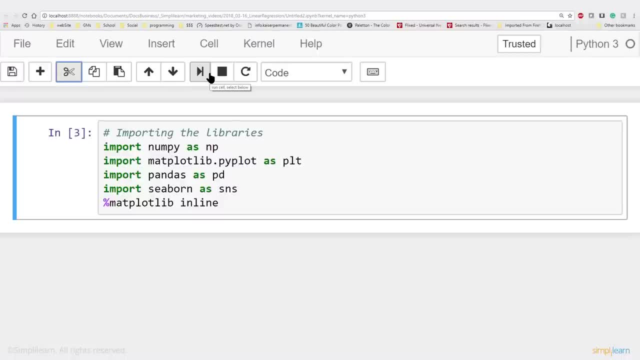 going to import matplotlibrarypyplot as plt and then seaborn as sns. Seaborn works with the matplot library, so you have to always import matplot library and then seaborn sits on top of it and we'll take a look at what that looks like. You could use any of your own. 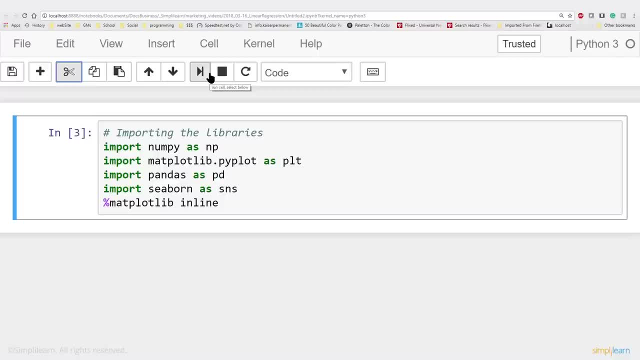 plotting libraries you want. There's all kinds of ways to look at the data. These are just very common ones, and the seaborn is so easy to use. it just looks beautiful. It's a nice representation that you can actually take and show somebody. And the final line is the amberson matplot library inline. That is. 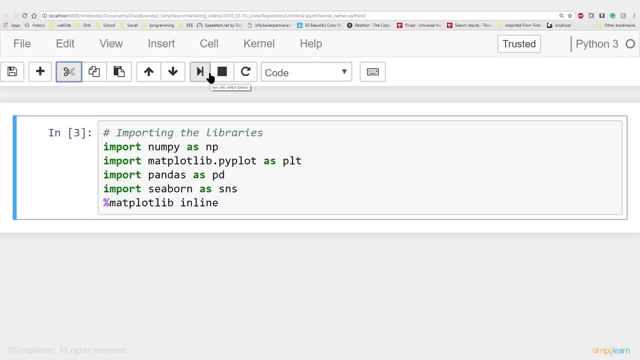 only because I'm doing an inline IDE. My interface in the anaconda jupyter notebook is a little bit more complicated than the other ones, So I'm going to go ahead and run this. It's not going to be that interesting because we're just setting. 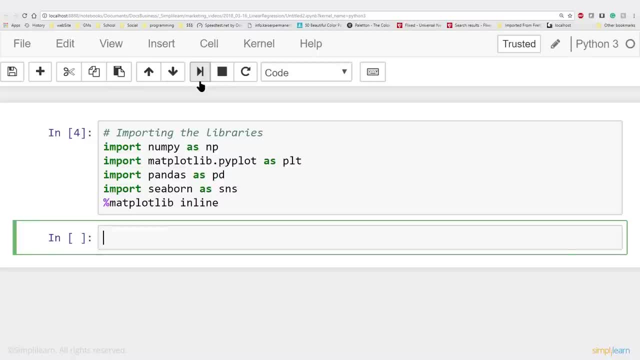 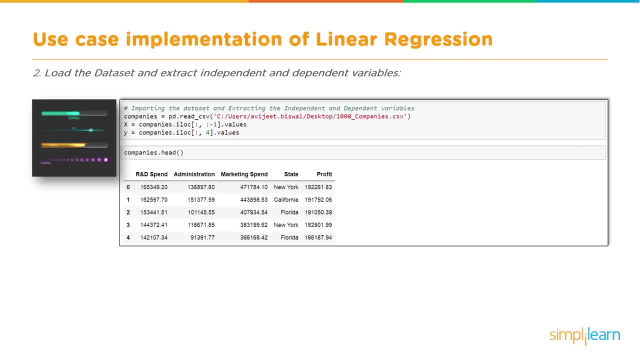 up variables. In fact, it's not going to do anything that we can see, but it is importing these different libraries and setup. The next step is load the data set and extract independent and dependent variables. Now here in the slide you'll see companies equals pdreadcsv and it has a long line there with the file at. 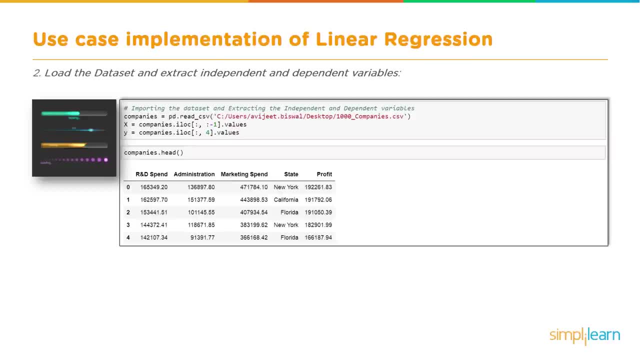 the end 1000 companiescsv. You're going to have to change this to fit whatever setup you have In the file itself. you can request: Just go down to the commentary below this video and put a note in there and simply learn. will try. 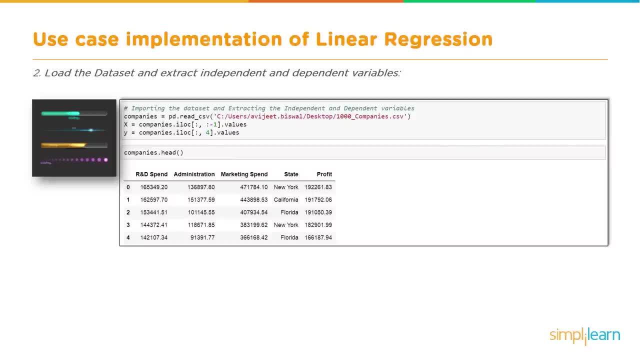 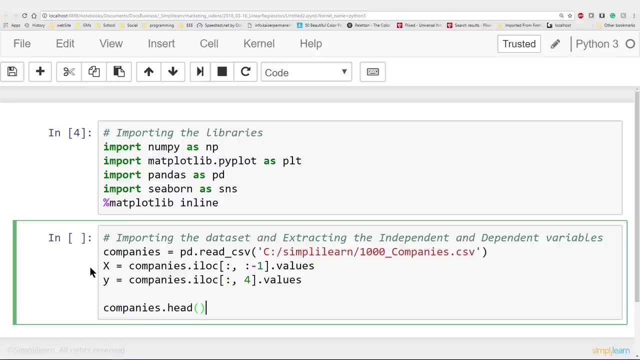 to get in contact with you and supply you with that file so you can try this coding yourself. So we're going to add this code in here and we're going to see that I have companies equals, pdreader underscore CSV, and I've changed this path to match my computer c colon slash. simply learn: slash 1000 underscore. 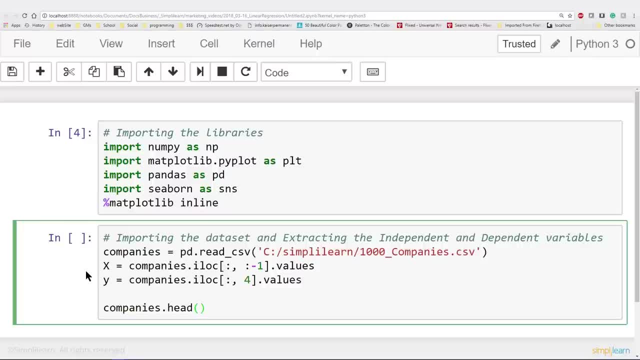 companies dot, CSV and then below there we're going to set: the X equals to companies under the i location and because this is companies is a PD data set, I can use this nice notation that says: take every row, that's what the colon, the first colon, is comma, except for the. 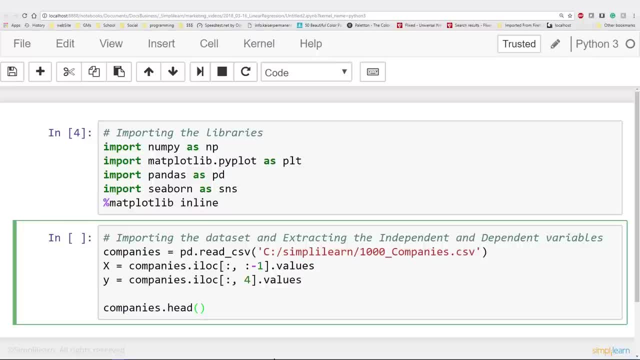 last column. That's what the second part is, where we have a colon minus one and we want the values set into there. So x is no longer a data set, a pandas data set, but we can easily extract the data from our pandas data set with this notation. And then y we're going to set equal to the last. 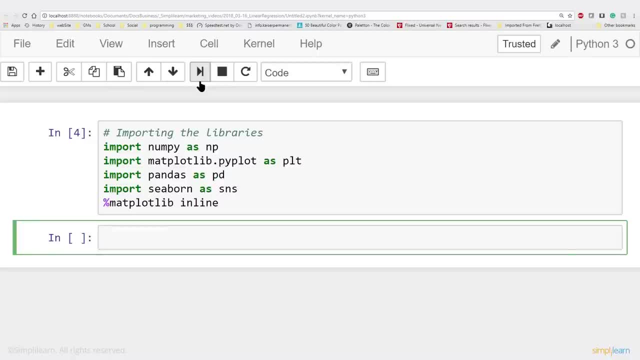 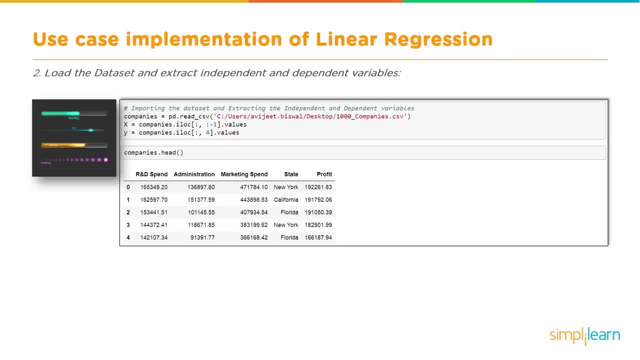 So we're just setting up variables. In fact, it's not going to do anything that we can see, but it is importing these different libraries and setup. The next step is load the data set and extract independent and dependent variables. Now here in the slide you'll see companies equals pdreadcsv. 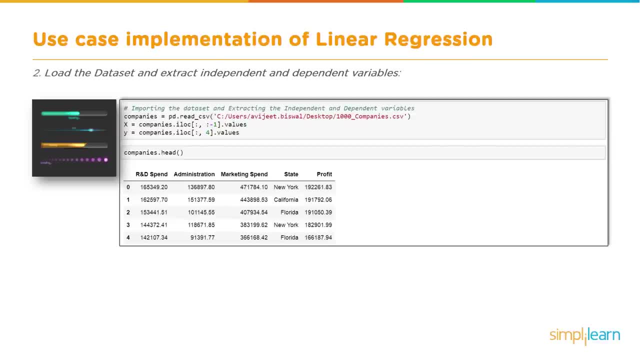 And it has a long line there with the file at the end 1000companiescsv. You're going to have to change this to fit whatever setup you have In the file itself. you can request: Just go down to the commentary below this video and put a note in there. 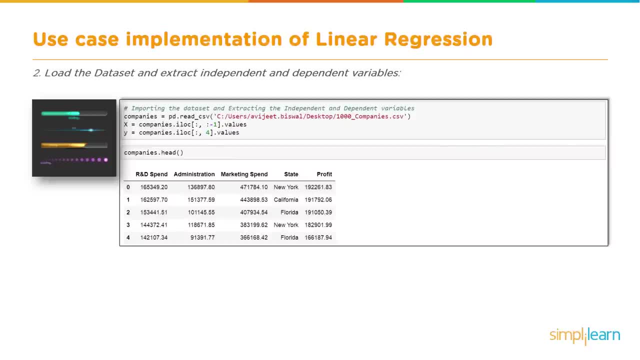 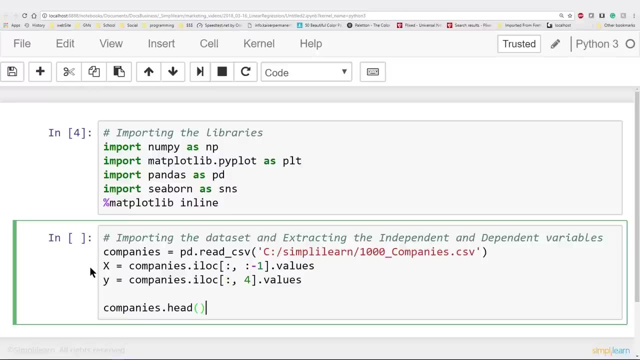 And Simply Learn, will try to get in contact with you and supply you with that file So you can try this coding yourself. So we're going to add this code in here And we're going to see that I have companies equals pdreadercsv. 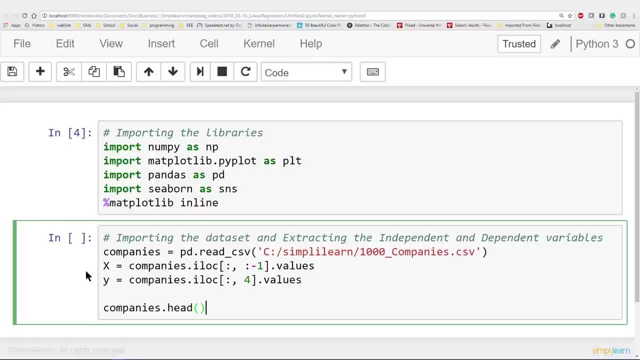 And I've changed this path to match my computer C colon slash. simply learn: slash 1000 underscore companies, dot, csv, And then below there we're going to set the x equals to companies under the i location And because this is companies is a pd data set. 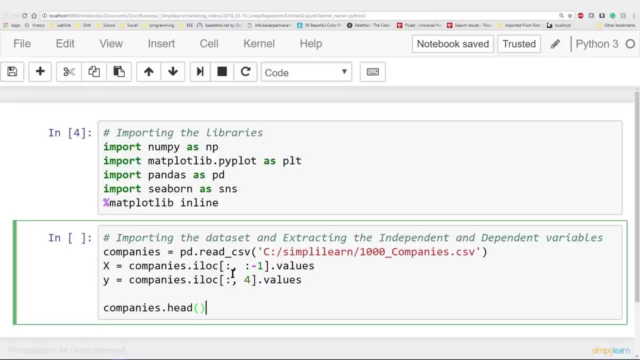 I can use this nice notation that says: take every row, That's what the colon, the first colon is comma, except for the last column. That's what the second part is, where we have a colon minus one And we want the values set into there. 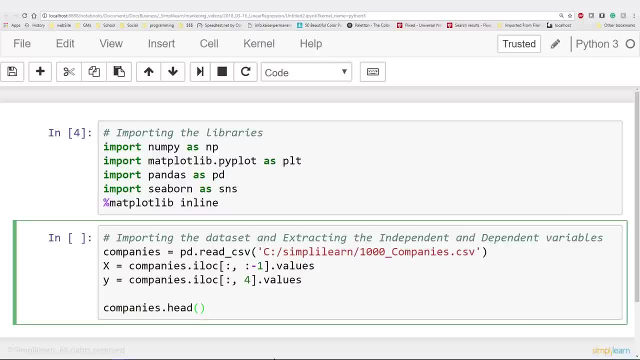 So x is no longer a data set, a pandas data set, But we can easily extract the data from our pandas data set with this notation, And then y we're going to set equal to the last row. Well, the question is going to be: what are we actually looking at? 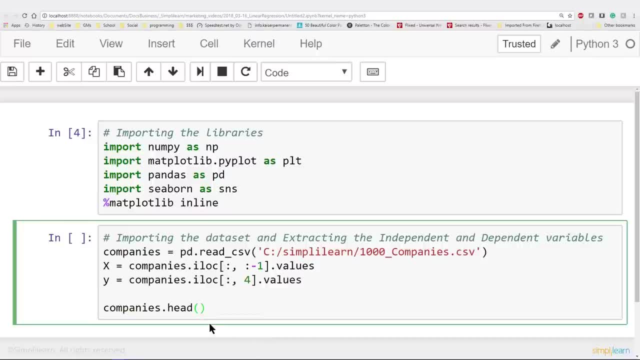 So let's go ahead and take a look at that, And we're going to look at the companies dot head, which lists the first five rows of data, And I'll open up the file in just a second so you can see where that's coming from. 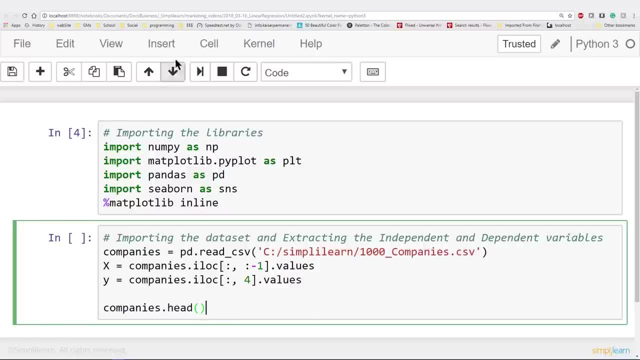 But let's look at the data in here. as far as the way the pandas sees it, When I hit run, you'll see it breaks it out into a nice setup. This is what pandas- one of the things pandas is really good about- 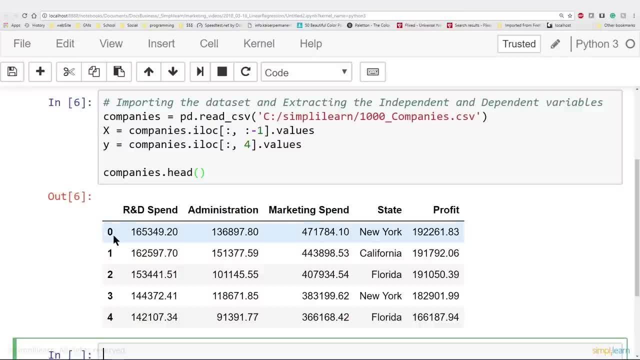 is. it looks just like an Excel spreadsheet. You have your rows And remember, when we're programming, we always start with zero, We don't start with one, So it shows the first five rows: 0, 1,, 2, 3, 4.. 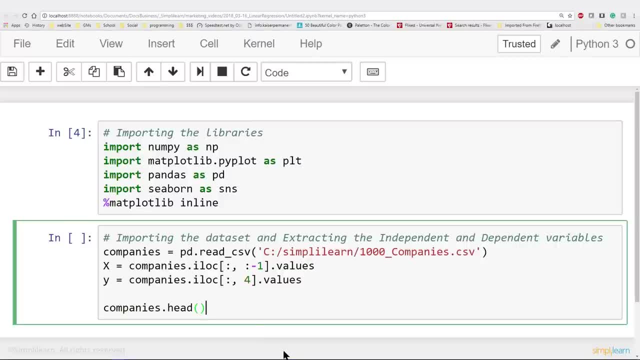 row. Well, the question is going to be: what are we actually looking at? So let's go ahead and take a look at that, and we're going to look at the companieshead, which lists the first five rows of data, And I'll open up the file in just a second so you can see where that's coming from. 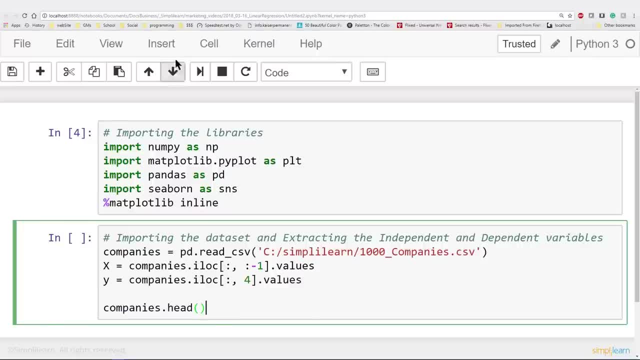 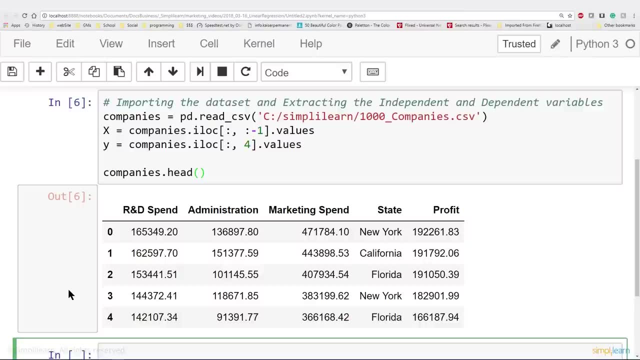 But let's look at the data in here. as far as the way the pandas sees it. When I hit run, you'll see it breaks it out into a nice setup. This is what pandas- one of the things pandas is really good about- is it looks just like an Excel spreadsheet. You have your rows and remember when we're. 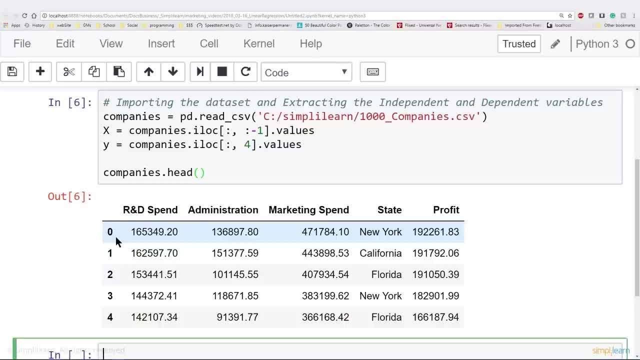 programming, we always start with zero. We don't start with zero, we start with zero, We start with one. So it shows the first five rows zero: one, two, three, four, and then it shows your different columns: R&D spend, administration, marketing spend, state profit. It even notes that 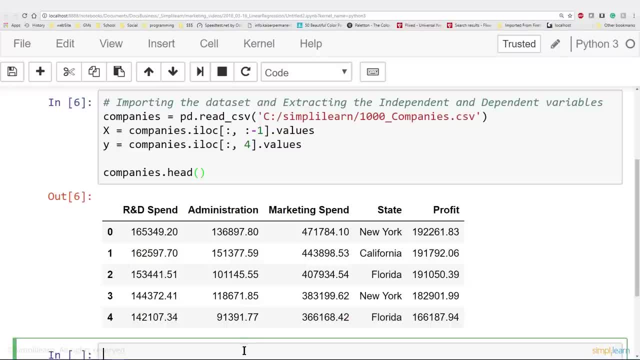 the top are column names. It was never told that, but pandas is able to recognize a lot of things- that they're not the same as the data rows. Why don't we go ahead and open this file up in a CSV so you can actually see the raw data? So here I've opened it up as a text editor and you can see at. 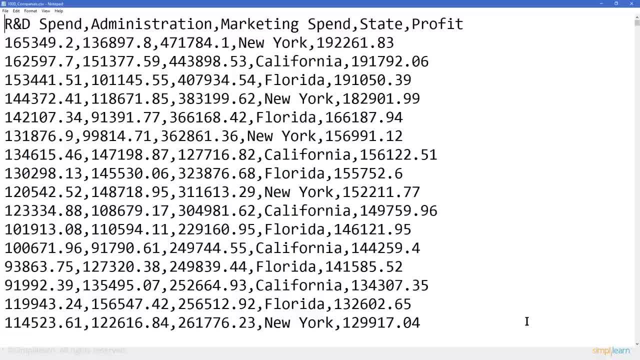 the top we have R&D spend and then we've got the column names. And we've got the column names: R&D spend, administration marketing spend, state profit, carries, return. I don't know about you, but I'd go crazy trying to read files like this. That's why we use the pandas You could also open. 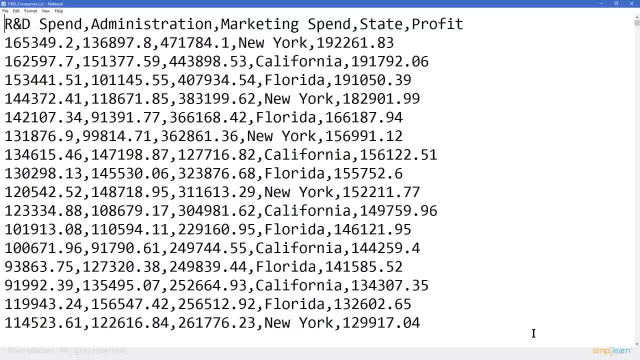 this up in an Excel and it would separate it, since it is a comma separated variable file. But we don't want to look at this one. We want to look at something we can read rather easily. So let's flip back and take a look at that top part, the first five rows. Now, as nice as this format is, 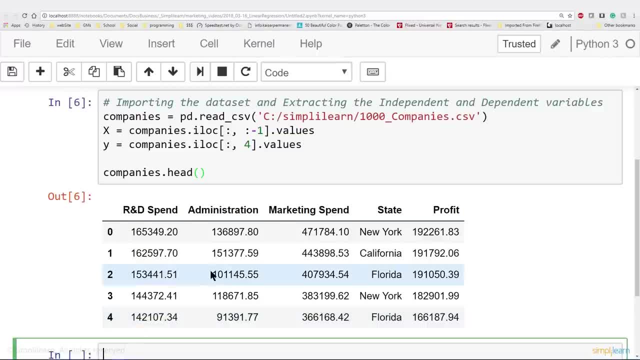 And then it shows your different columns: R&D spend, administration, marketing spend, state profit. It even notes that the top are column names. It was never told that, but pandas is able to recognize a lot of things- that they're not the same as the data rows. 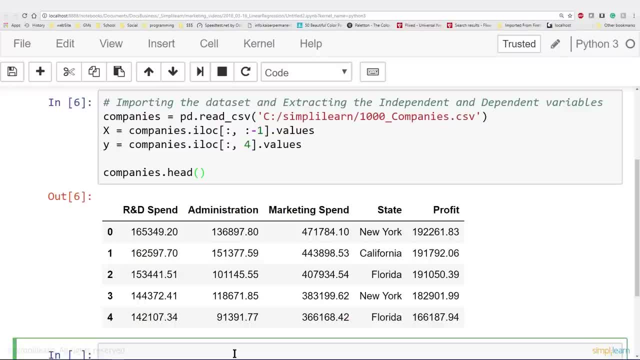 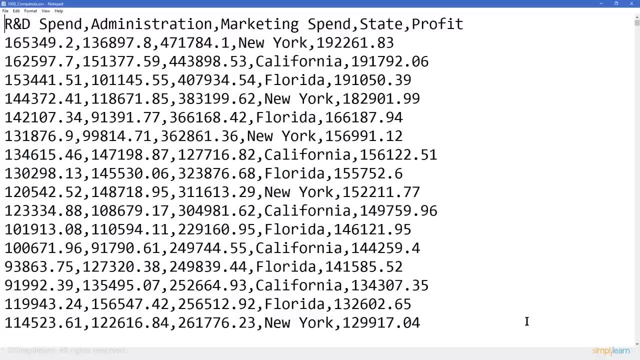 Why don't we go ahead and open this file up in a CSV so you can actually see the raw data? So here I've opened it up as a text editor And you can see at the top we have R&D spend comma administration, comma marketing, spend comma state. 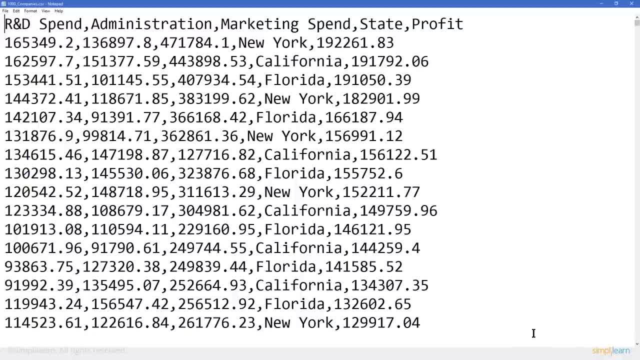 comma profit carries return. I don't know about you, but I'd go crazy trying to read files like this. That's why we use the pandas. You could also open this up in an Excel and it would separate it, since it is a comma separated variable file. 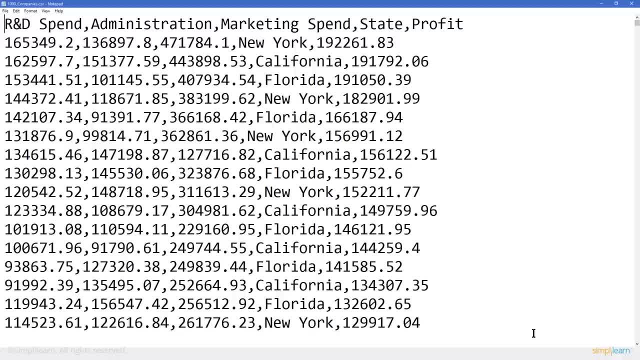 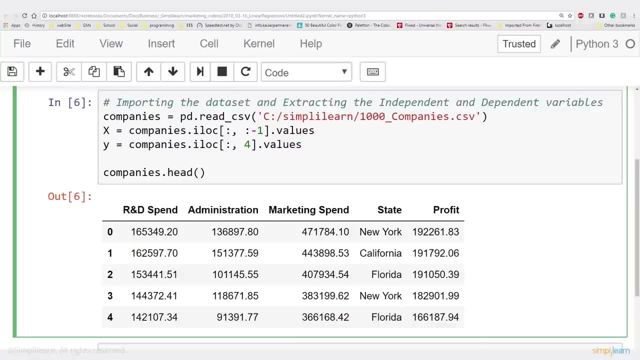 But we don't want to look at this one. We want to look at something we can read rather easily. So let's flip back and take a look at that top part, the first five rows. Now, as nice as this format is, where I can see the data, to me it doesn't mean a whole lot. 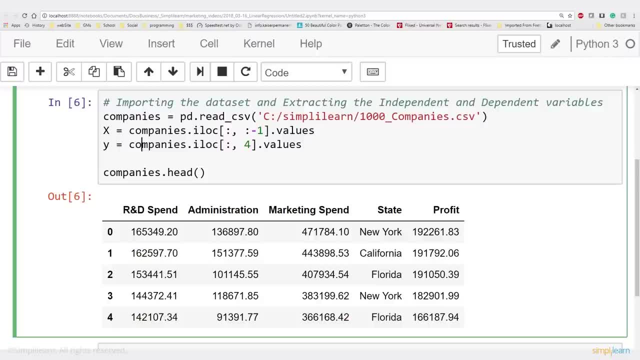 where I can see the data. to me it doesn't mean a whole lot. Maybe you're an expert in business, in investments, and you understand what $165,349.20 compared to the administration cost of $136,897.80, so on, so on, helps to create the profit of $192,261.83.. That makes no sense to me. 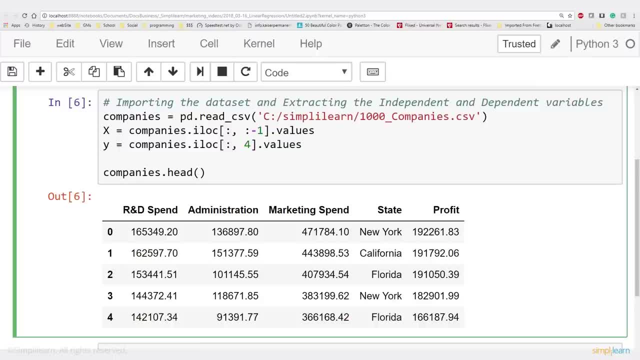 whatsoever, No pun intended. So let's flip back here and take a look at our next set of code, where we're going to graph it so we can get a better understanding of our data and what it means. So at this point we're going to use the pandas, So let's flip back here and take a look. 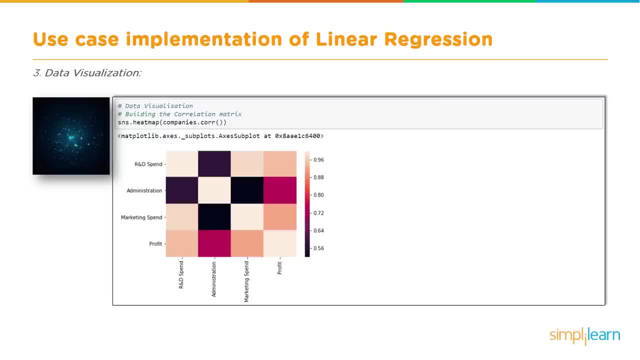 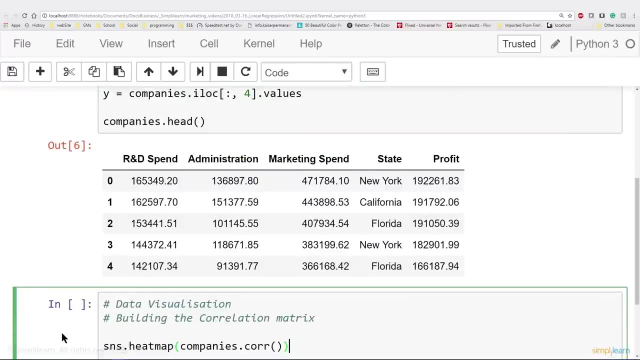 at our next set of code where we're going to use a single line of code to get a lot of information. so we can see where we're going with this. Let's go ahead and paste that into our notebook and see what we got going, And so we have the visualization and again we're using SNS. 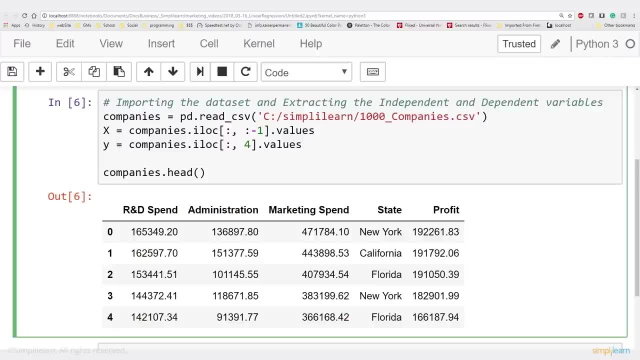 Maybe you're an expert in business And you understand what $165,349.20, compared to the administration cost of $136,897.80, so on, so on- helps to create the profit of $192,261.83.. 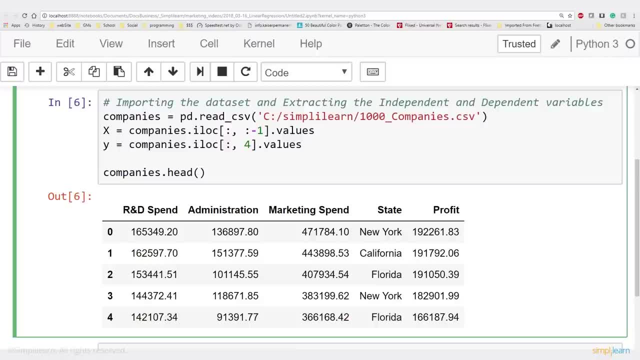 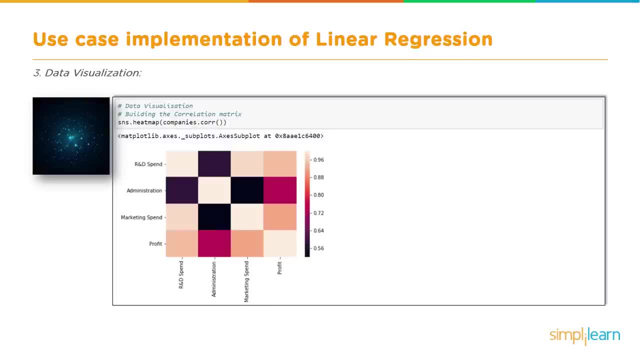 That makes no sense to me whatsoever. No pun intended. So let's flip back here and take a look at our next set of code, where we're going to graph it so we can get a better understanding of our data and what it means. So at this point we're going: 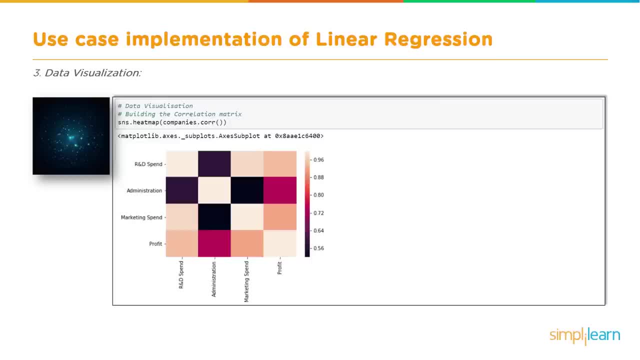 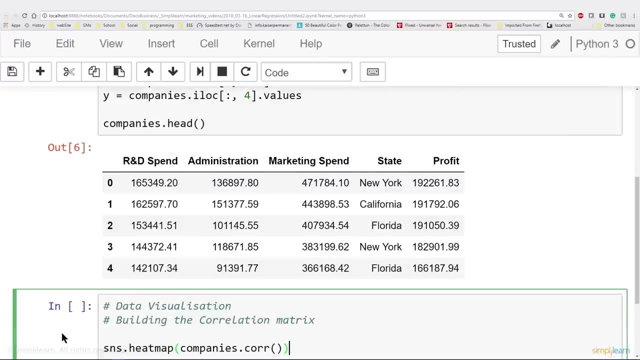 to use a single line of code to get a lot of information so we can see where we're going with this. Let's go ahead and paste that into our notebook and see what we got going. And so we have the visualization. And again we're using SNS, which is pandas. 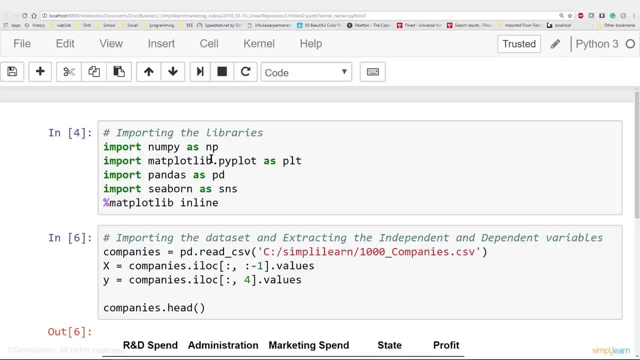 As you can see, we imported the matplotlibrarypyplot as PLT, which then the seaborn uses, And we imported the seaborn as SNS, And then that final line of code helps us show this in our inline coding. Without this we wouldn't be able to do this. 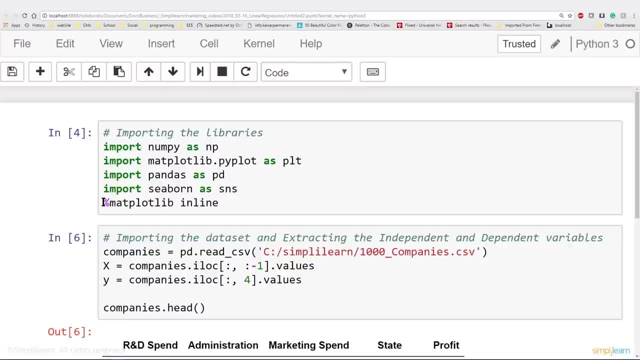 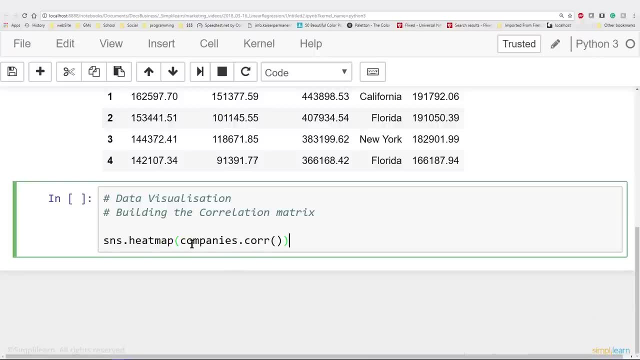 It wouldn't display And you could display it to a file and other means And that's the matplotlibrary inline with the amber sign at the beginning. So here we come down to the single line of code. Seaborn is great because it actually recognizes the panda data frame. 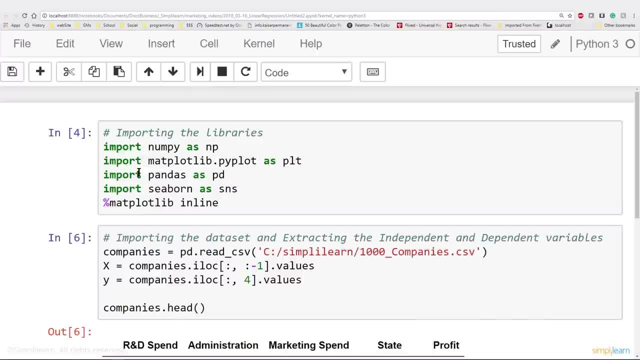 which is pandas. As you can see, we imported the matplotlibrarypyplot as PLT, which then the seaborn uses, And we imported the seaborn as SNS, And then that final line of code helps us show this in our inline coding. Without this it wouldn't work. So we're going to go ahead and 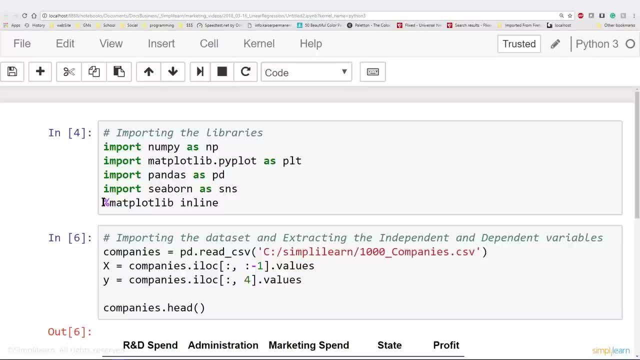 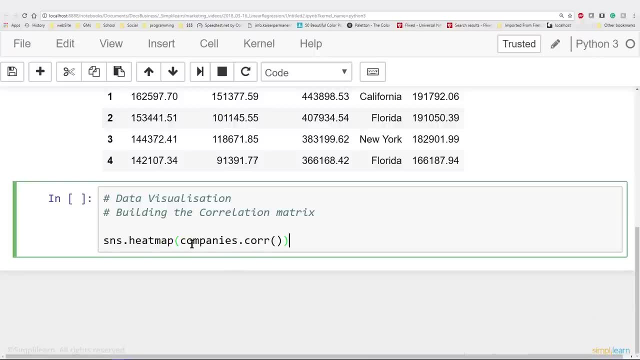 see what it would display And you can display it to a file and other means. And that's the matplotlibrary inline with the amber sign at the beginning. So here we come down to the single line of code. Seaborn is great because it actually recognizes the panda data frame. So I can just 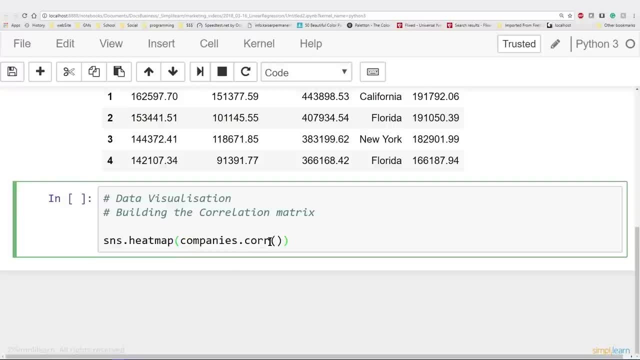 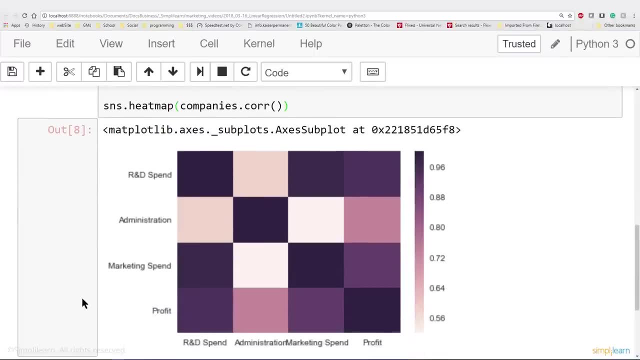 take the companiescore for coordinates and I can put that right into the seaborn. And when we run this we get this beautiful plot. And let's just take a look at what this plot means. If you look at this plot on mine, the colors are probably a little bit more purplish and blue than the original. 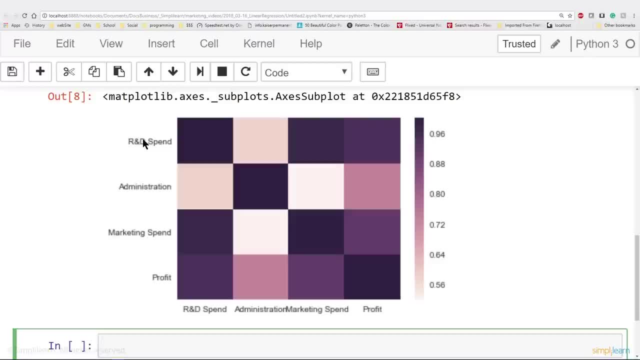 one. We have the columns and the rows, We have R and D spending, We have administration, We have marketing spending and profit And if you cross index any two of these- since we're interested in profit- if you cross index profit with profit, it's going to show up. if you look at the scale on the 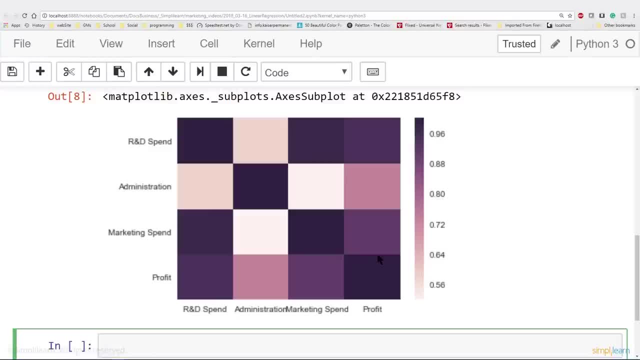 right way up in the dark. Why? Because those are the same data. They have an exact correspondence. So R and D spending is going to be the same as R and D spending and the same thing with administration costs. So right down the middle you get this dark row. 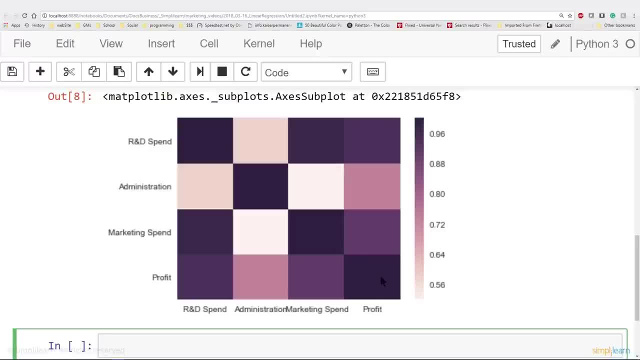 dark diagonal row that shows that this is the highest corresponding data. That's exactly the same. And as it becomes lighter there's less connections between the data. So we can see: with profit, obviously profit is the same as profit. And next, it has a very high correlation with R and D. 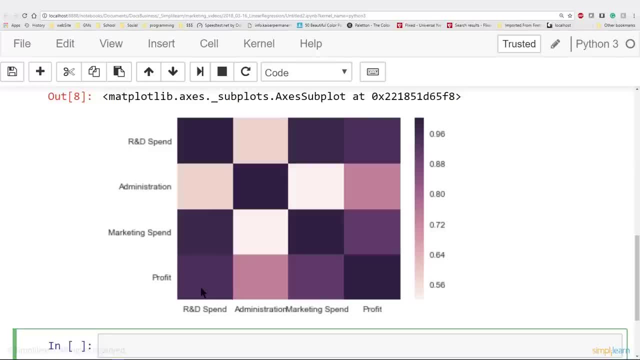 spending, which we looked at earlier, And it has a slightly less connection to marketing spending and even less to how much money we put into the administration. So now that we have a nice look at the data, let's go ahead and dig in and create a little bit of a graph And we're going to have a 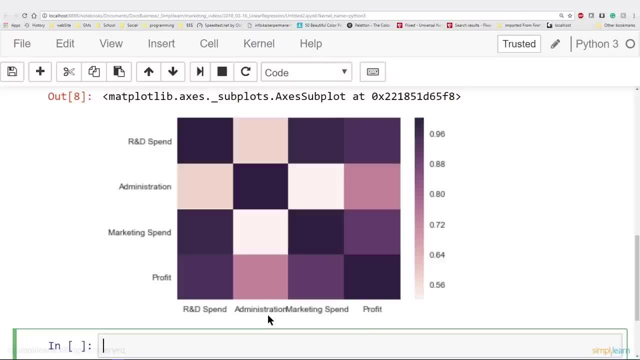 look at some actual, useful linear regression models so that we can predict values and have a better profit. Now that we've taken a look at the visualization of this data, we're going to move on to the next step. Instead of just having a pretty picture, we need to generate some hard data, some 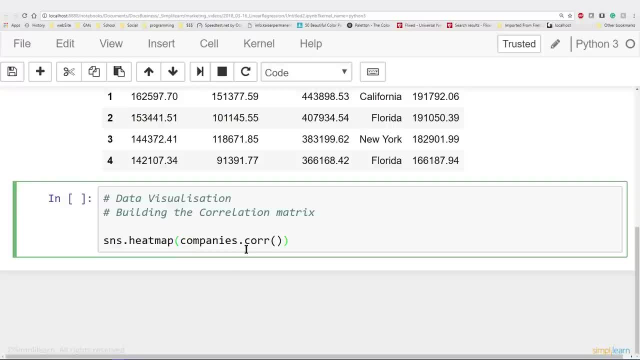 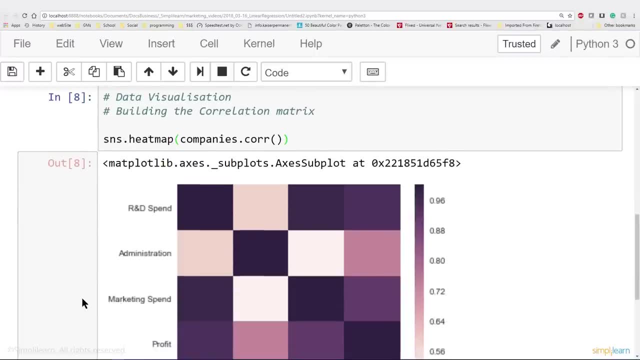 So I can just take the companiescore for coordinates And I can put that right into the seaborn. And when we run this we get this beautiful plot. And let's just take a look at what this plot means. If you look at this plot on mine, the colors are probably a little bit more purplish and blue than the original one. 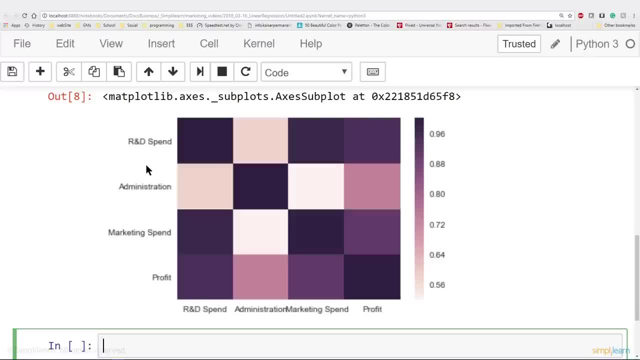 We have the columns and the rows, We have R&D spending, we have administration, we have marketing spending and profit. And if you cross-index any two of these- since we're interested in profit- if you cross-index profit with profit, it's going to show up. if you look at the scale on the right way up in the dark. 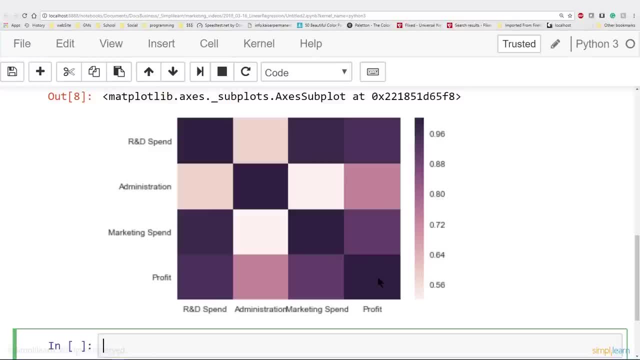 Why? Because those are the same data. They have an exact correspondence. So R&D spending is going to be the same as R&D spending and the same thing with administration costs. So right down the middle you get this dark row, Or dark diagonal row that shows that this is the highest corresponding data. that's exactly the same. 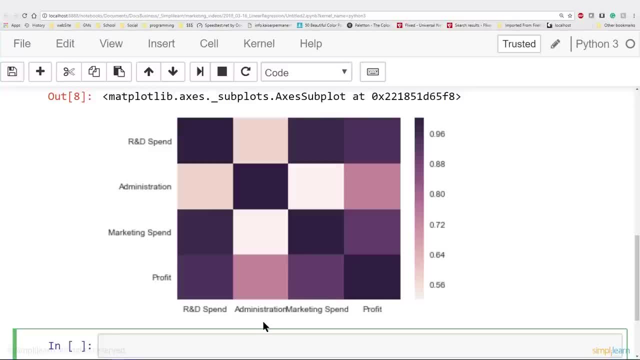 And as it becomes lighter, there's less connections between the data. So we can see: with profit, obviously profit is the same as profit And next it has a very high correlation with R&D spending, which we looked at earlier, And it has a slightly less connection to marketing spending and even less to how much money we put into the administration. 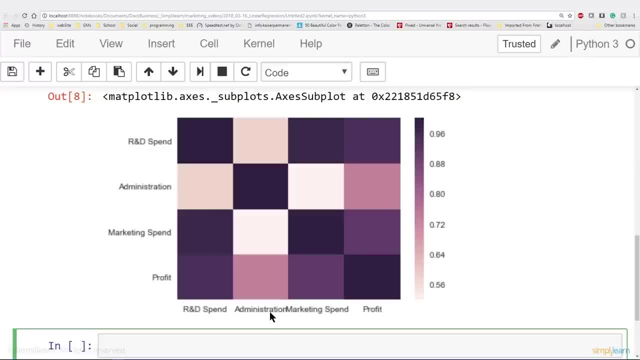 So, now that we have a nice look at the data, let's go ahead and dig in And create some actual, useful linear regression models so that we can predict values and have a better profit Now that we've taken a look at the visualization of this data. 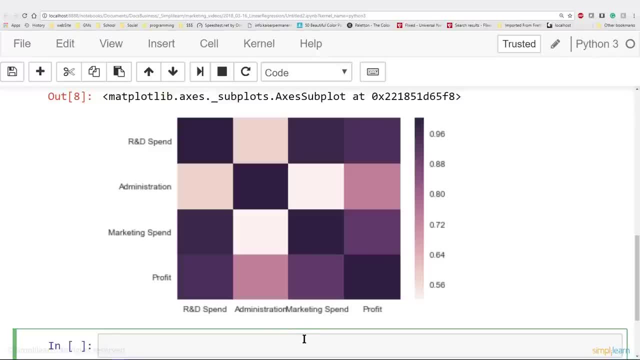 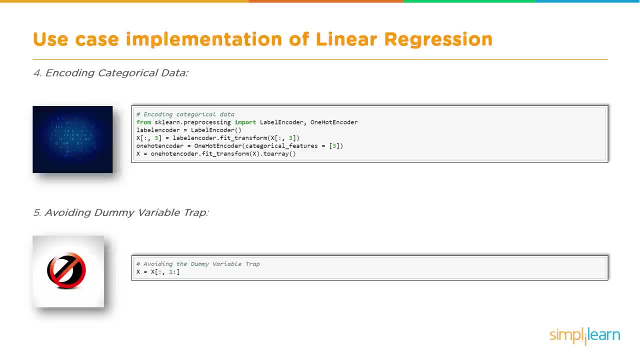 we're going to move on to the next step. Instead of just having a pretty picture, we need to generate some hard data, some hard values. So let's see what that looks like. We're going to set up our linear regression model in two steps. 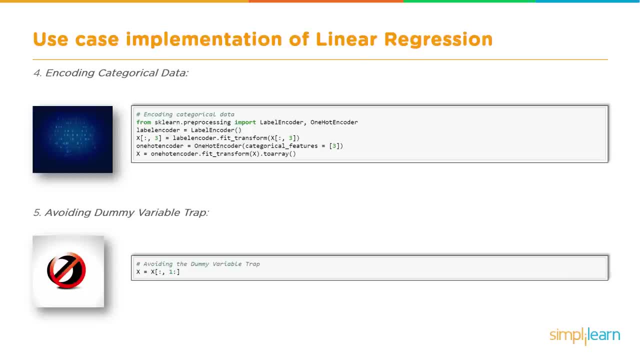 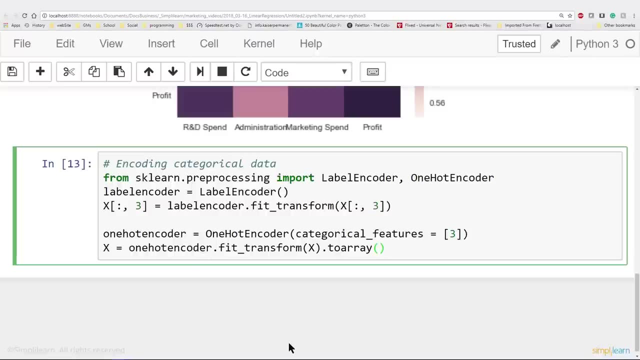 The first one is we need to prepare some of our data so it fits correctly, And let's go ahead and paste this code into our Jupyter notebook. And what we're bringing in is we're going to bring in the sklearn preprocessing where we're going to import the label encoder and the one hot encoder. 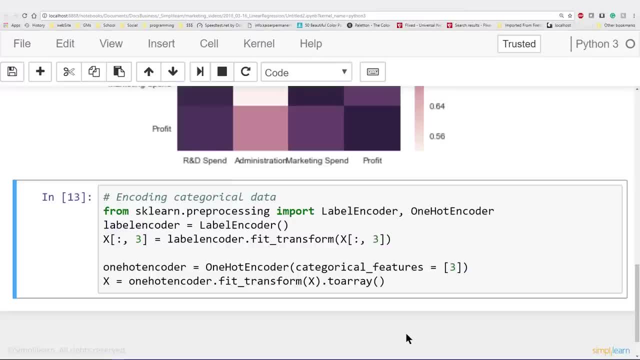 To use the label encoder. we're going to create a variable called label encoder and set it equal to capital L label capital E encoder. This creates a class that we can reuse for transferring the labels back and forth. Now about now, you should ask: what labels are we talking about? 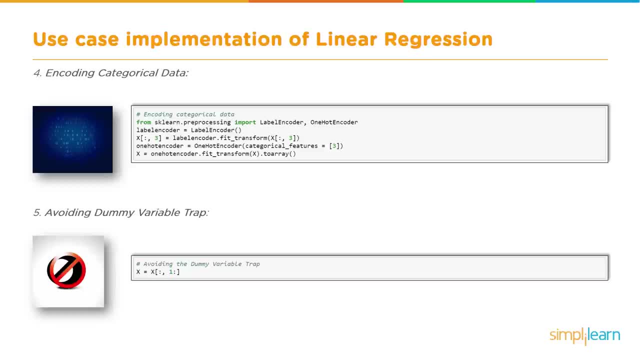 hard values. So let's see what that looks like. We're going to set up our linear regression model in two steps. The first one is we need to prepare some of our data so it fits correctly, And let's go ahead and paste this code into our Jupyter notebook. And what we're bringing. 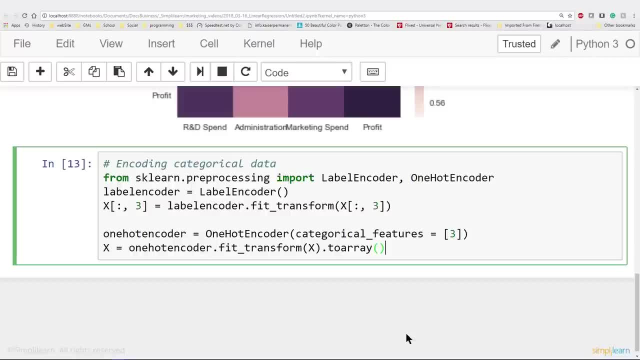 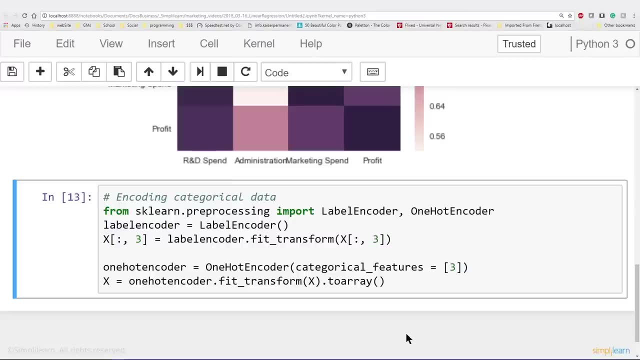 in is we're going to bring in the sklearn preprocessing where we're going to import the label encoder and the one hot encoder To use the label encoder. we're going to create a variable called label encoder and set it equal to capital L label, capital E encoder. This creates a class that we 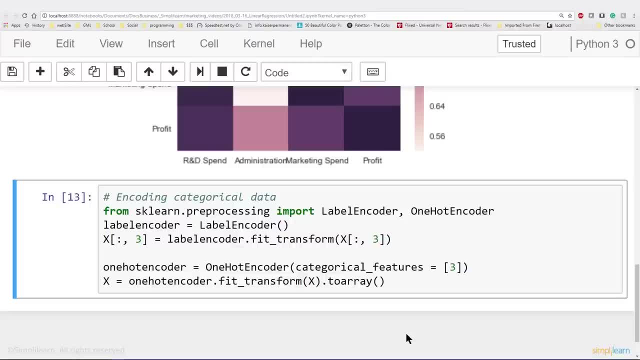 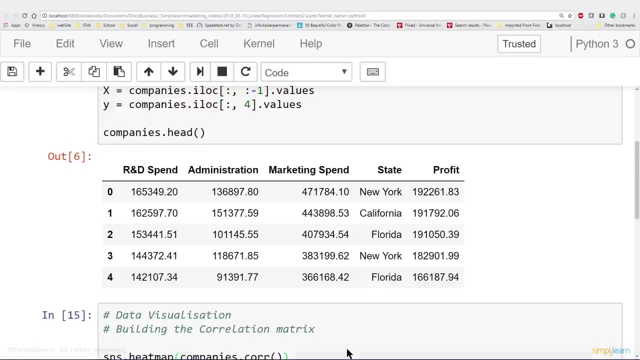 can reuse for transferring the labels back and forth. Now about now, you should ask: what labels are we talking about? Let's go take a look at the data we processed before and see what I'm talking about here. If you remember, when we did the companieshead and we printed the top, 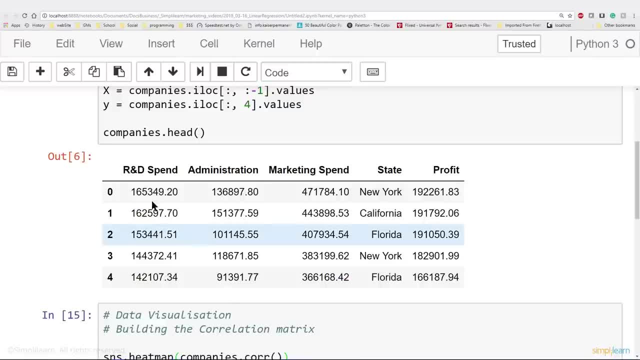 five rows of data. we have our columns going across. We have column zero, which is R&D spending, column one, which is administration, column two, which is marketing spending, and column three is state. And you'll see, under state we have New York, California, Florida. Now to do a linear, 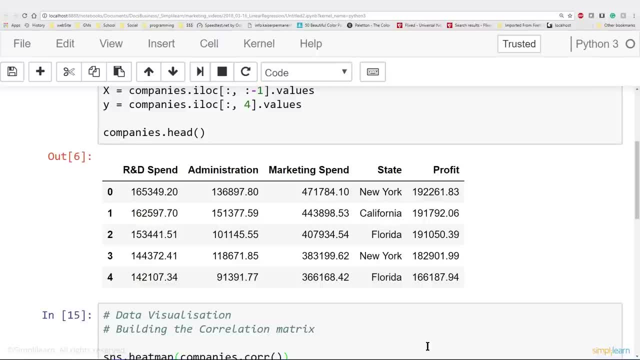 regression model. it doesn't know how to process New York. It knows how to process a number. So the first thing we're going to do is we're going to change that- New York, California and Florida- and we're going to change those to numbers. That's what this line of code 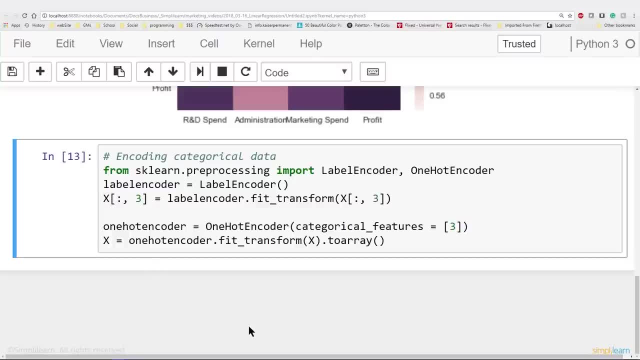 does. here X equals, and then it has the colon comma three in brackets. The first part. the colon comma, means that we're going to look at all the different rows, So we're going to keep them all together. But the only row we're going to edit is the third row, And in there we're going to take. 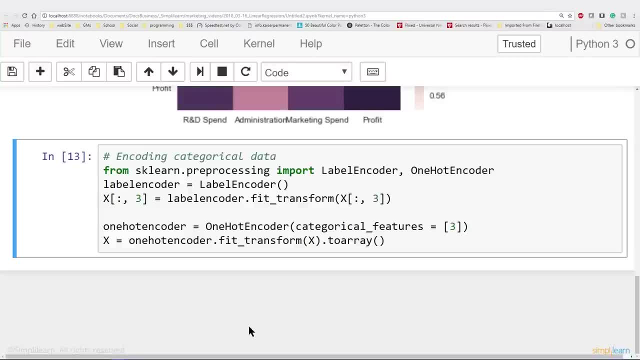 the label coder and we're going to fit and transform the X, also the third row. So we're going to take that third row, we're going to set it equal to a transformation And that transformation basically tells it that instead of having a New York, it has a zero or a one. 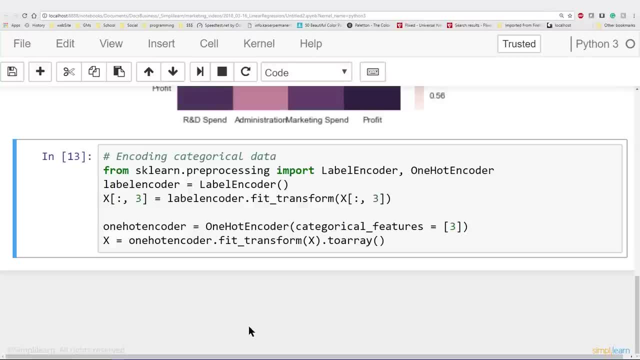 or a two. And then, finally, we need to do a one hot encoder, which equals one hot encoder categorical features equals three. And then we take the X and we go ahead and do that. equal to one hot encoder. fit, transform X to array. This final transformation preps our data for us. 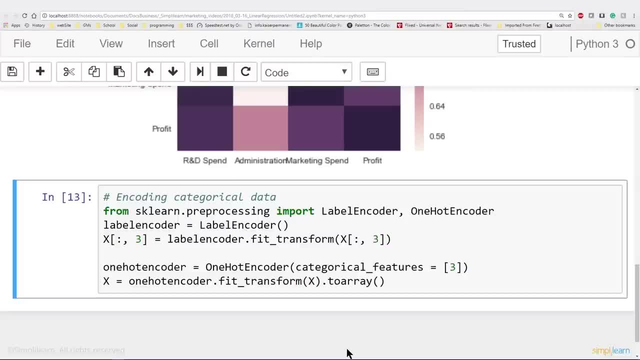 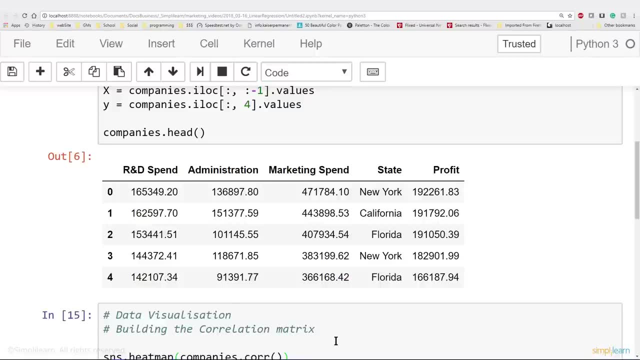 Let's go take a look at the data we processed before and see what I'm talking about here. If you remember, when we did the companieshead, we printed the top five rows of data. We have our columns going across. We have column 0,, which is R&D spending. 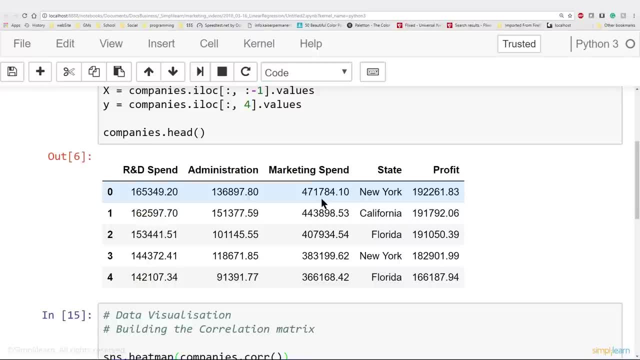 Column 1, which is administration, Column 2,, which is marketing spending, And column 3 is state. And you'll see, under state we have New York, California, Florida, Now to do a linear regression model. it doesn't know how to process New York. 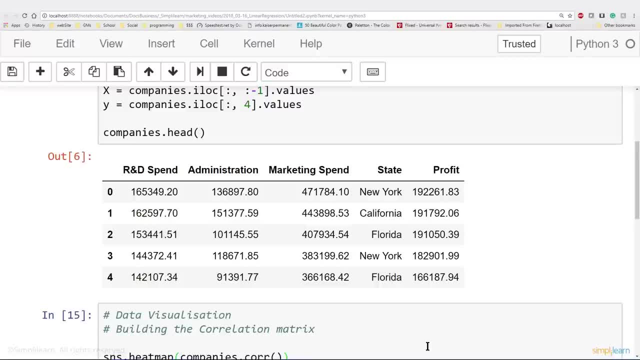 It knows how to process a number. So the first thing we're going to do is we're going to change that- New York, California and Florida- And we're going to change those to numbers, And that's what this line of code does here. 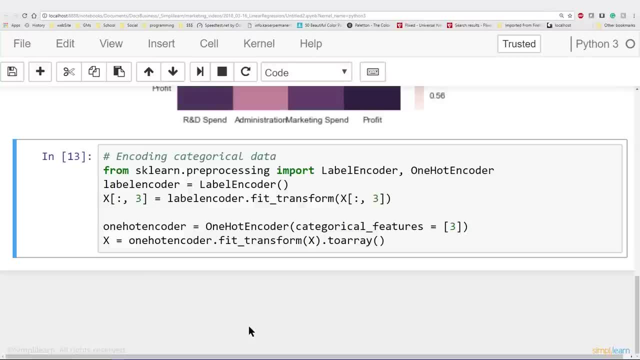 X equals, and then it has the colon comma 3 in brackets, The first part. the colon comma means that we're going to look at all the different rows, So we're going to keep them all together, But the only row we're going to edit is the third row. 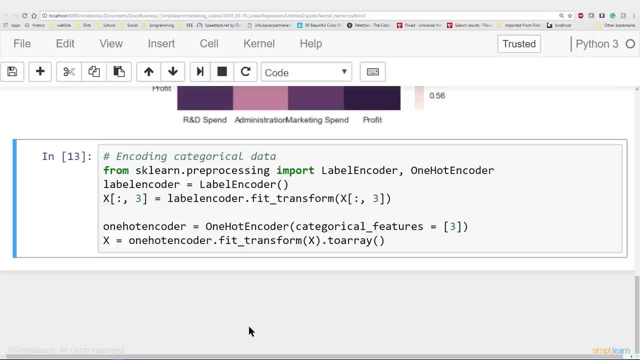 And in there we're going to take the label coder And we're going to fit and transform the X, also the third row. So we're going to take that third row, We're going to set it equal to a transformation And that transformation basically tells it that instead of having a New York, 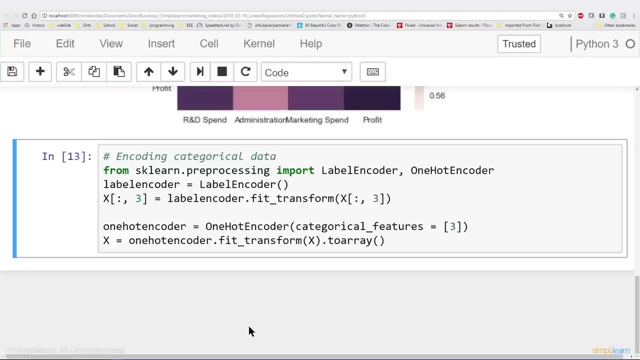 we're going to have a zero or a one or a two, And then finally, we need to do a one hot encoder which equals one hot encoder categorical features equals three. And then we take the X and we go ahead and do that. equal to one hot encoder. fit. transform X to array. 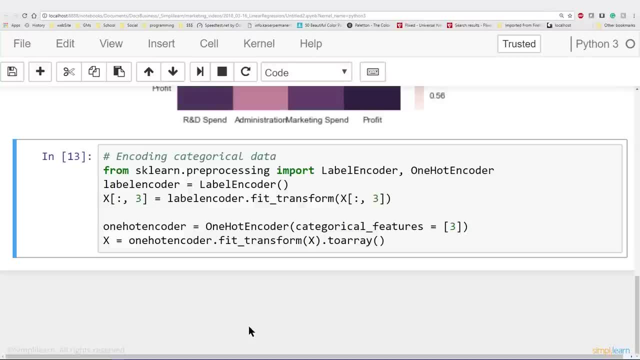 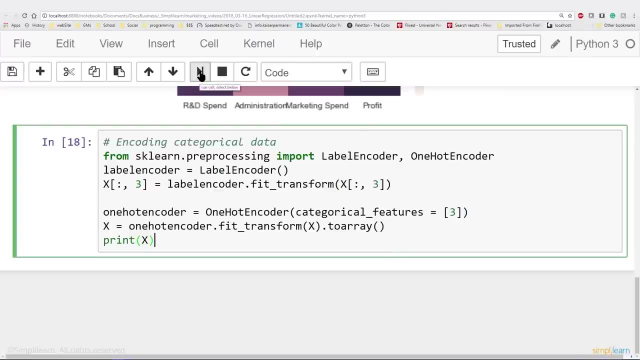 This final transformation preps our data for us, so it's completely set the way. we need it as just a row of numbers. Even though it's not in here, let's go ahead and print X and just take a look at what this data is doing. 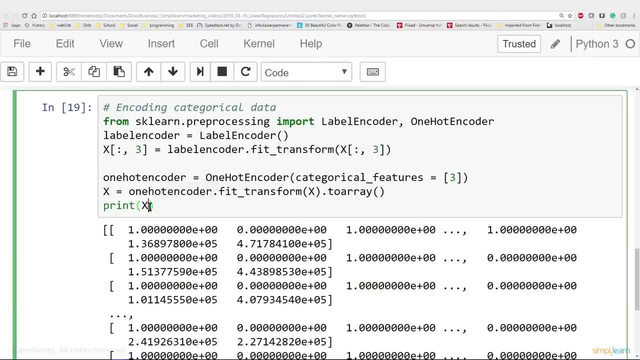 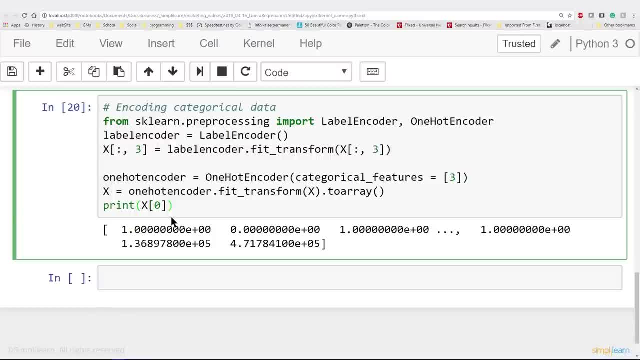 You'll see you have an array of arrays. It's a row of numbers, And if I go ahead and just do row zero, you'll see I have a nice organized row of numbers that the computer now understands. We'll go ahead and take this out there, because it doesn't mean a whole lot to us. 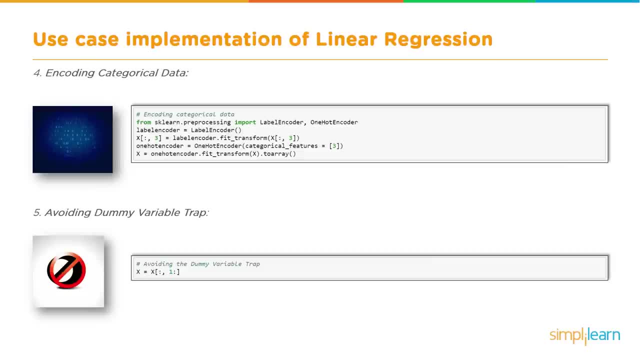 It's just a row of numbers. Next, on setting up our data, we have avoiding dummy variable trap. This is very important. Why? Because the computer has automatically transformed our header into the setup And it's automatically transferred all these different variables. 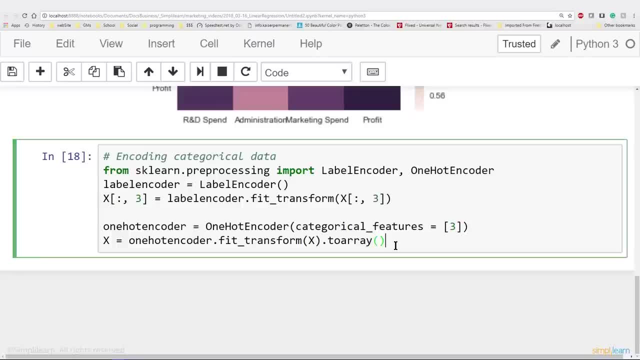 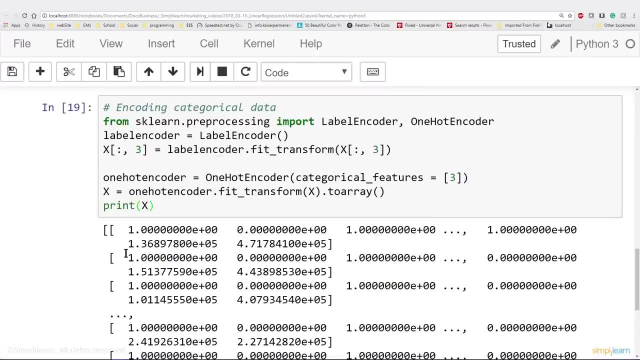 so it's completely set the way. we need it as just a row of numbers. Even though it's not in here, let's go ahead and print X and just take a look at what this data is doing. You'll see you have an array of arrays and then each array is a row of numbers. 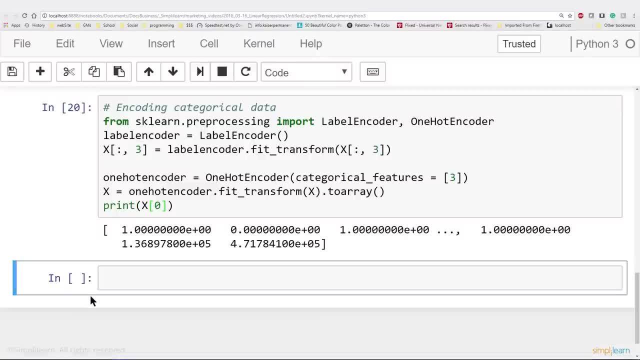 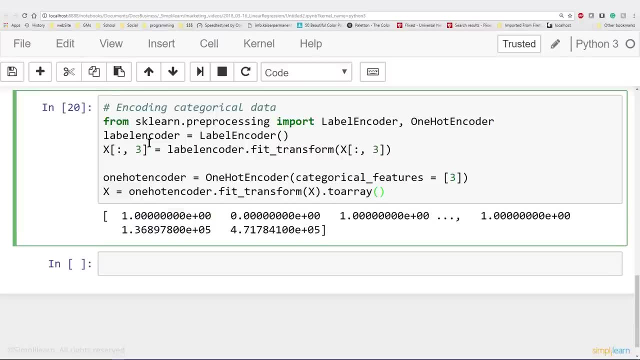 And if I go ahead and just do row zero, you'll see I have a nice organized row of numbers that the computer now understands. We'll go ahead and take this out there, because it doesn't mean a whole lot to us, it's just a row of numbers. Next, on setting up our data, we have avoiding dummy. 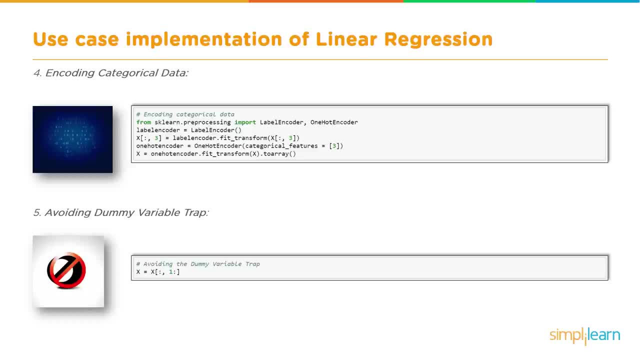 variable trap. This is very important. Why? Because the computer has automatically transformed our header into the setup and it's automatically transferred all these different variables. So when we did the encoder, the encoder automatically transformed our header into the setup and it's. 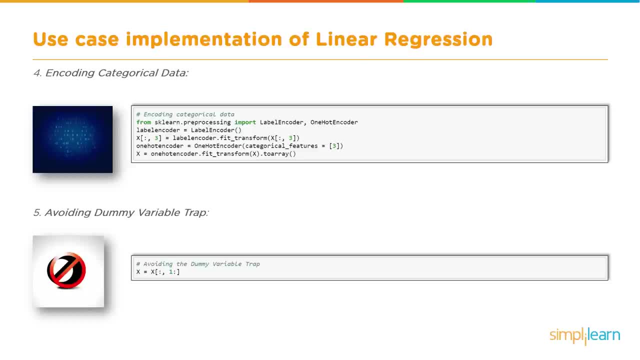 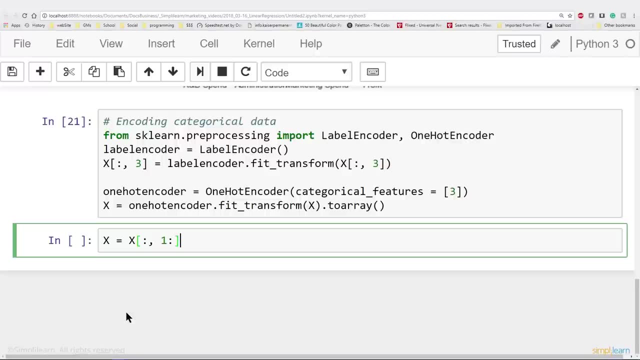 automatically transformed all these different variables. So when we did the encoder, the encoder created two columns And what we need to do is just have the one, because it has both the variable and the name. That's what this piece of code does here. Let's go ahead and paste this in here and we: 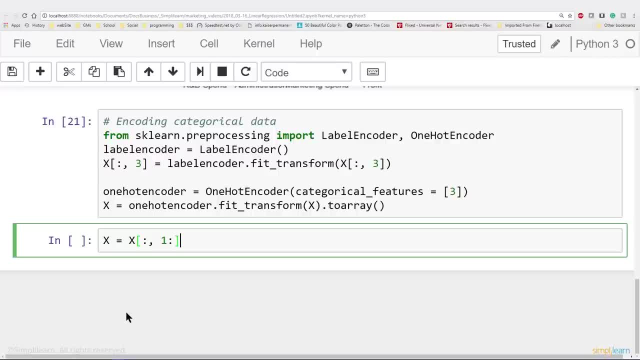 have X equals X colon, comma, one colon. All this is doing is removing that one extra column we put in there when we did our one hot encoder and our label encoding. Let's go ahead and run that And now we get to create our linear regression model And let's see what that looks like here And we're 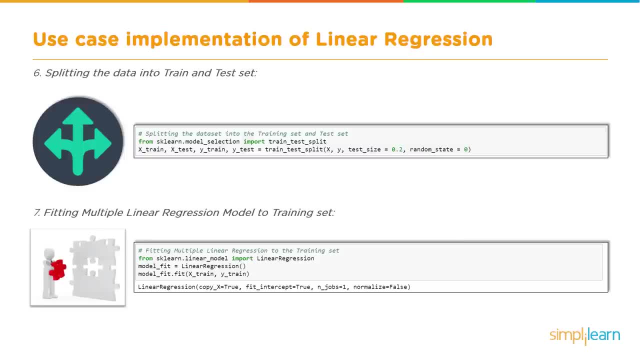 going to do that in two steps. The first step is going to be in splitting the data. Now, whenever we create a predictive model of data, we always want to split it up. so we have a training set and we have a testing set. That's. 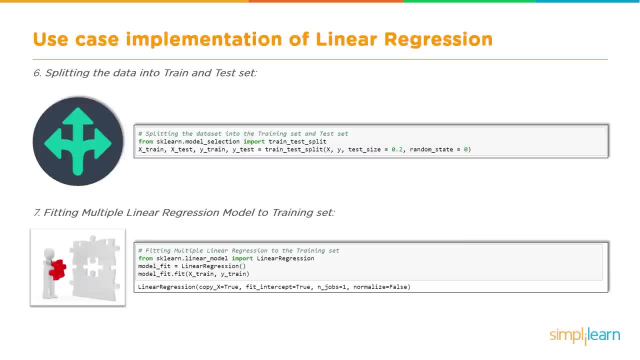 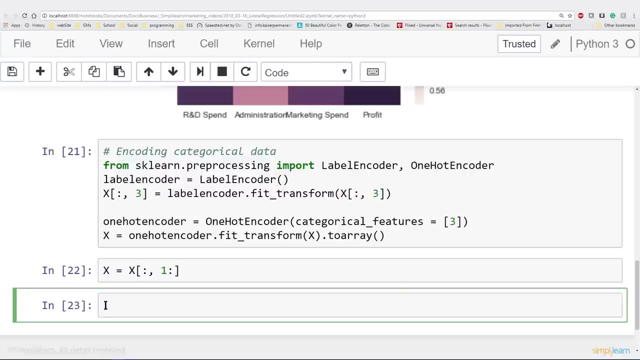 very important- otherwise we'd be very unethical- without testing it to see how good our fit is, And then we'll go ahead and create our multiple linear regression model and train it and set it up. Let's go ahead and paste this next piece of code in here and I'll go ahead and shrink it down a. 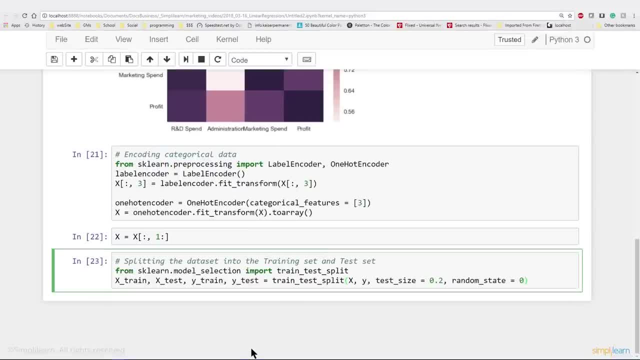 size or two, so it all fits on one line. So from the sklearn module selection we're going to import train test split And you'll see that we've created four completely different variables. We have capital X train, capital X test, smallercase y train. smallercase y test. 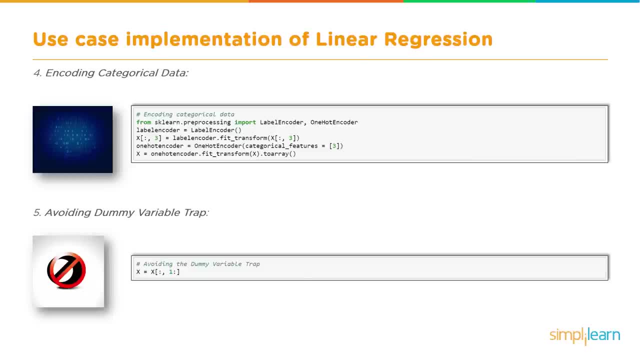 So when we did the end, the encoder created two columns And what we need to do is just have the one, because it has both the variable and the name. That's what this piece of code does here. Let's go ahead and paste this in here. 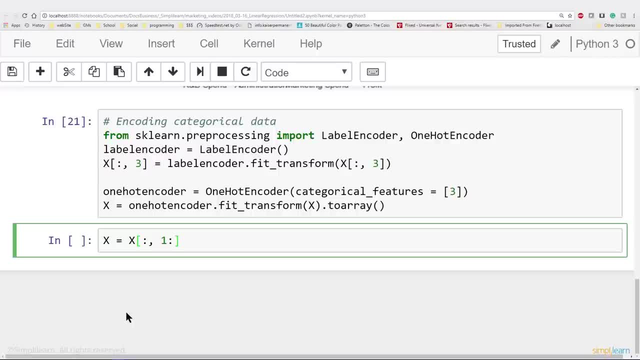 And we have X equals X colon, comma, one colon. All this is doing is removing that one extra column we put in there when we did our one hot encoder and our label encoding. Let's go ahead and run that And now we get to create our linear regression model. 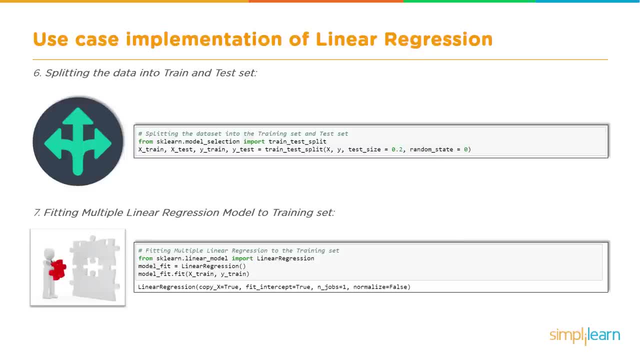 And let's see what that looks like here. We're going to do that in two steps. The first step is going to be in splitting the data. Now, whenever we create a predictive model of data, we always want to split it up. so we have a training set and we have a testing set. 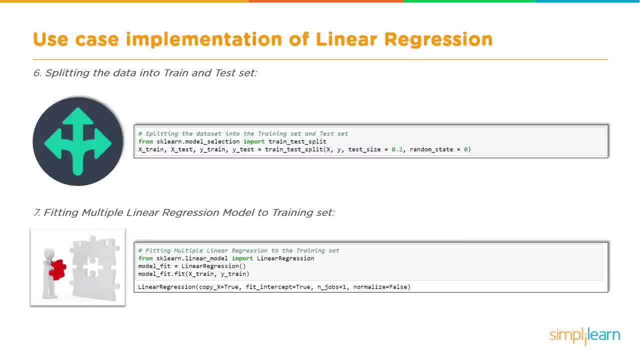 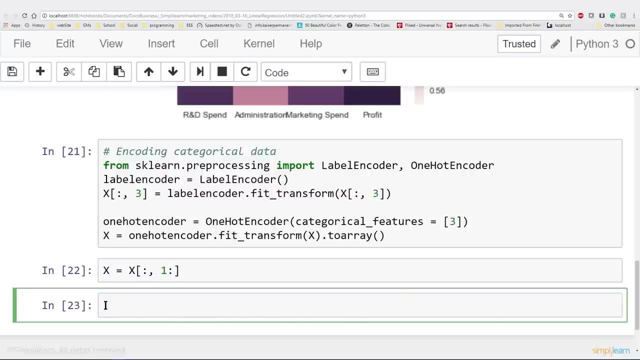 That's very important, Otherwise we'd be very unethical without testing it to see how good our fit is, And then we'll go ahead and create our multiple linear regression model and train it and set it up. Let's go ahead and paste this next piece of code in here: 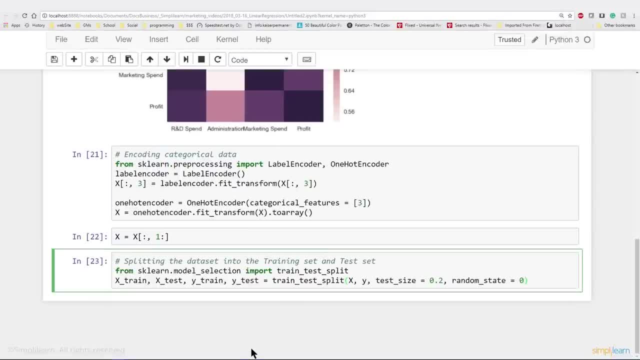 And I'll go ahead and shrink it down a size or two. It's on one line. So from the sklearn module selection we're going to import train test split And you'll see that we've created four completely different variables. We have capital X train. capital X test, smallercase y train. smallercase y test. 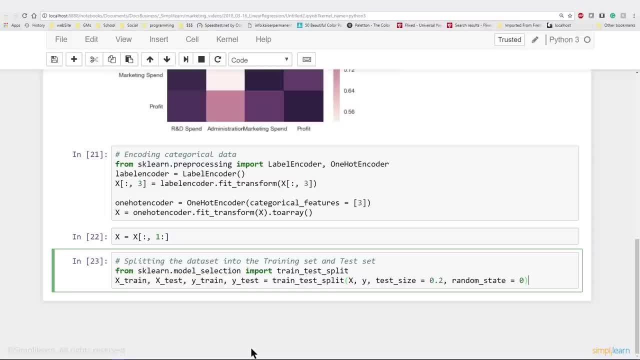 That is the standard way that they usually reference these. when we're doing different models, You usually see that at capital X You see the train and the test and the lowercase y. What this is is X is our data going in, That's our R&D spin, our administration, our marketing. 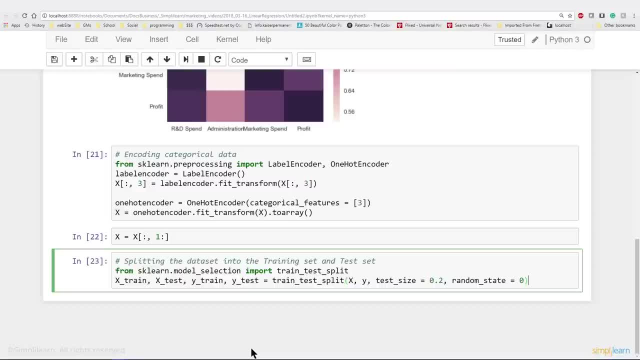 And then Y, which we're training, is the answer. That's the profit, Because we want to know the profit of an unknown entity. That's what we're going to shoot for in this tutorial. The next part, train test split. we take X and we take Y. 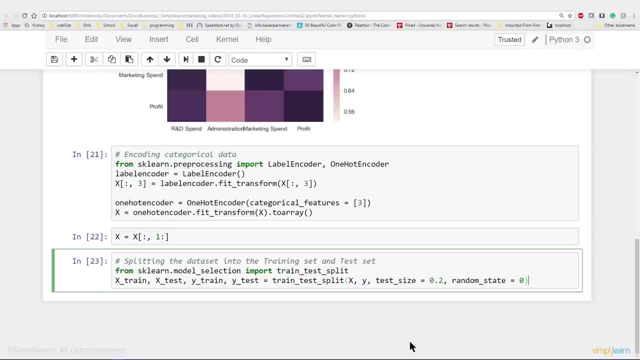 We've already created those. X has the columns with the data in it, and Y has a column with profit in it, And then we're going to set the test size equals 0.2.. That basically means 20%, So 20%. 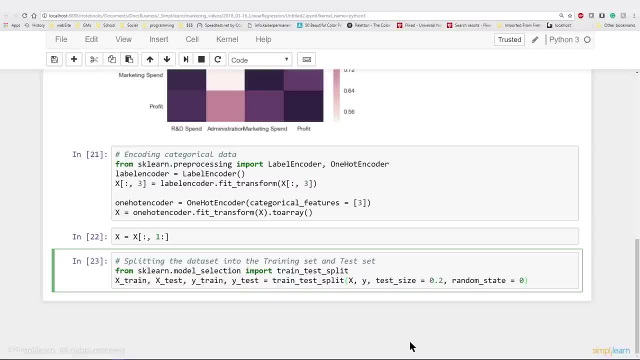 20% of the rows are going to be tested, We're going to put them off to the side. So, since we're using 1,000 lines of data, that means that 200 of those lines we're going to hold off to the side to test for later. 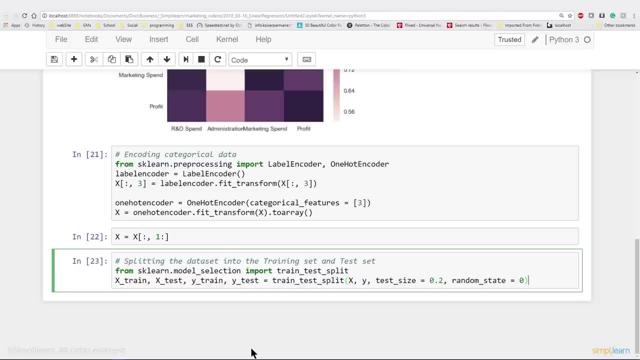 That is the standard way that they usually reference these. when we're doing different models, You usually see that a capital X, and you see the train and the test and the lowercase y. What this is is X. is our data going in? 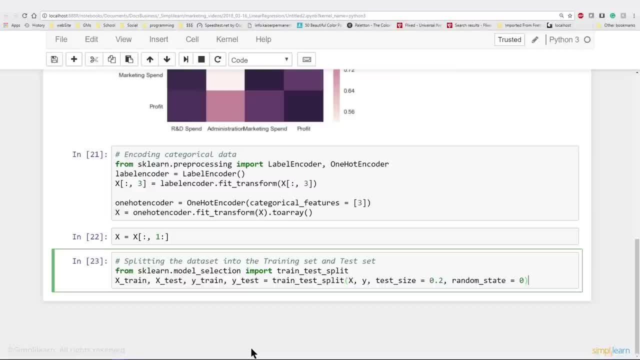 That's our R&D spin, our administration, our marketing, And then Y, which we're training, is the answer. That's the profit, Because we want to know the profit of an unknown entity. That's what we're going to shoot for in this tutorial. 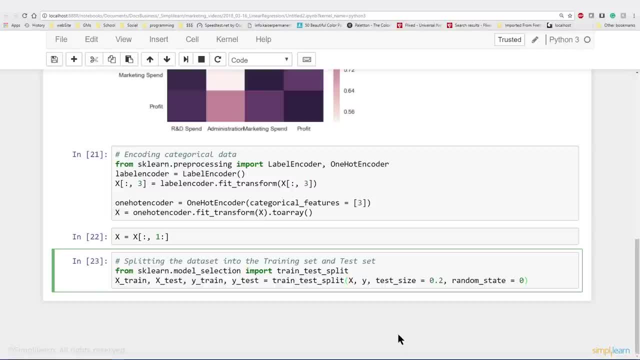 The next part, train test split. we take X and we take Y. We've already created those. X has the columns with the data in it and Y has a column with profit in it, And then we're going to set the test size equals 0.2.. 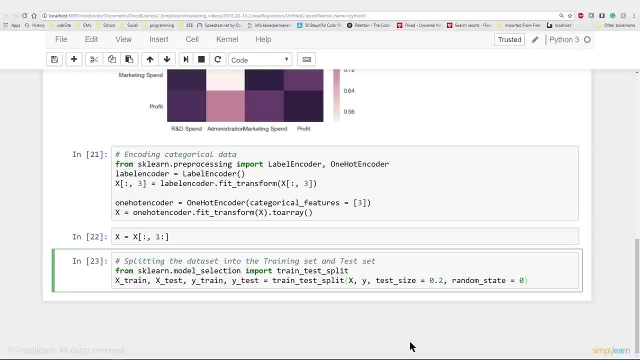 That basically means 20%. So 20%- 20% of the rows are going to be tested. We're going to put them off to the side. So, since we're using 1,000 lines of data, that means that 200 of those lines we're going to hold off to the side to test for later. 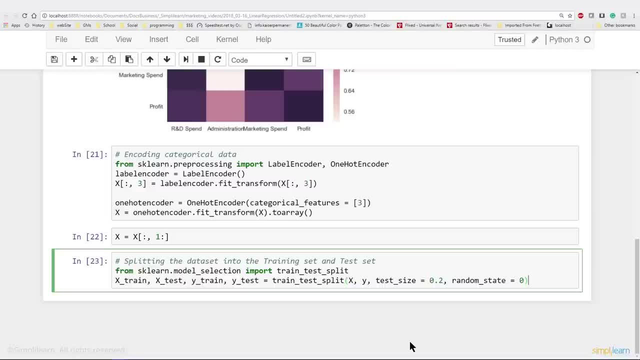 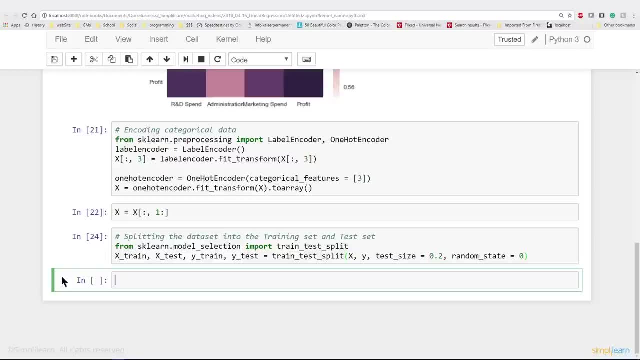 And then the random state equals 0.. We're going to randomize which ones it picks to hold off to the side. We'll go ahead and run this. It's not overly exciting because it's setting up our variables, But the next step is the next step. we actually create our linear regression model. 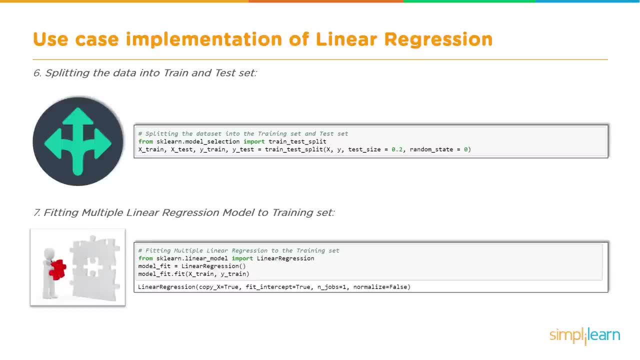 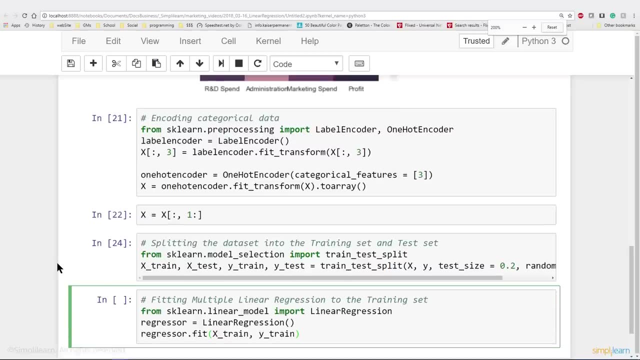 Now that we got to the linear regression model, we get that next piece of the puzzle. Let's go ahead and put that code in there and walk through it. So here we go, We're going to paste it in there And let's go ahead. and since this is a shorter line of code, let's zoom up there so we can get a good look. 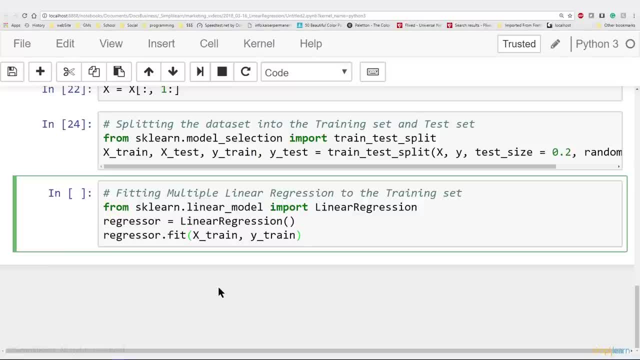 And we have from the sklearnlinear underscore model. we're going to import linear regression Now. I don't know if you recall from earlier when we were doing all the math. let's go ahead and flip back there and take a look at that. 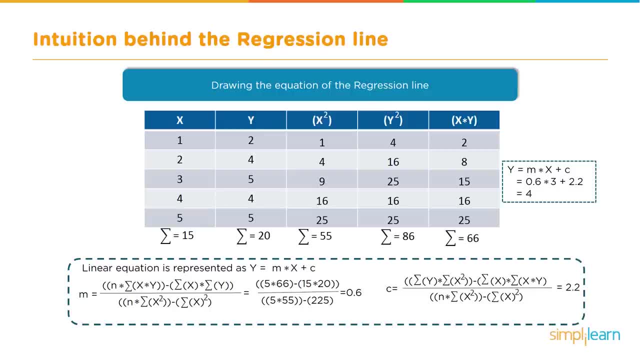 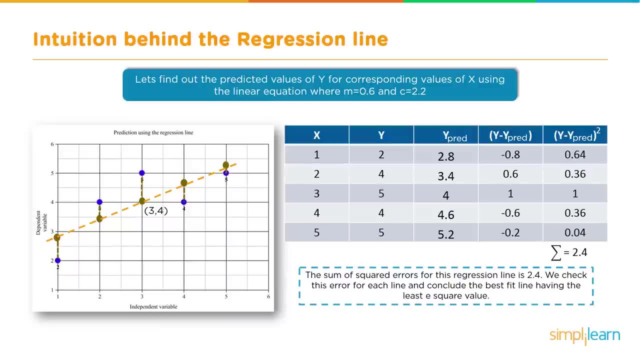 Do you remember this, where we had this long formula on the bottom and we were doing all this summarization, And then we also looked at setting it up with the different lines, And then we also looked all the way down to Multiple linear regression where we're adding all those formulas together. 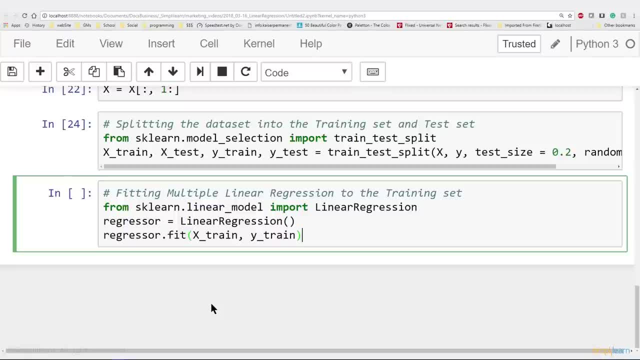 All of that is wrapped up in this one section. So what's going on here is I'm going to create a variable called regressor, And the regressor equals the linear regression. That's a linear regression model that has all that math built in. 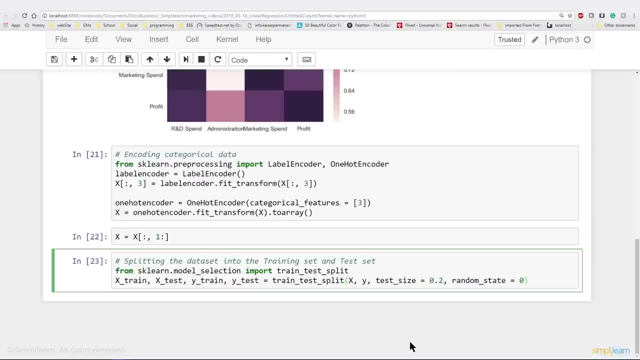 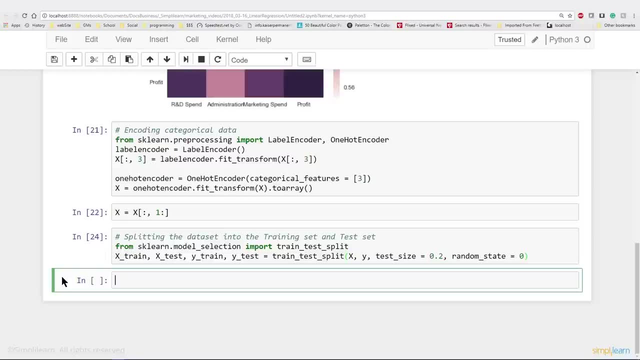 And then the random state equals 0.. We're going to randomize which ones it picks to hold off to the side. We'll go ahead and run this. It's not overly exciting because it's setting up our variables, But the next step is the next step. we actually create our linear regression model. 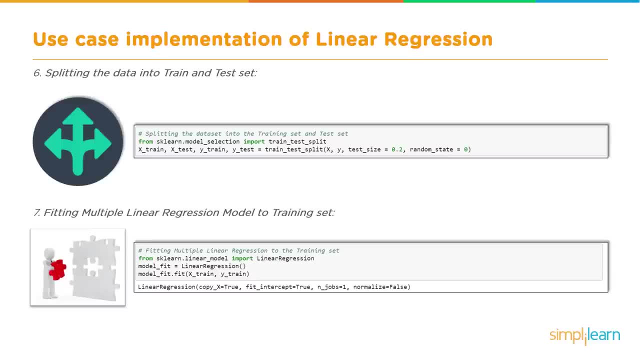 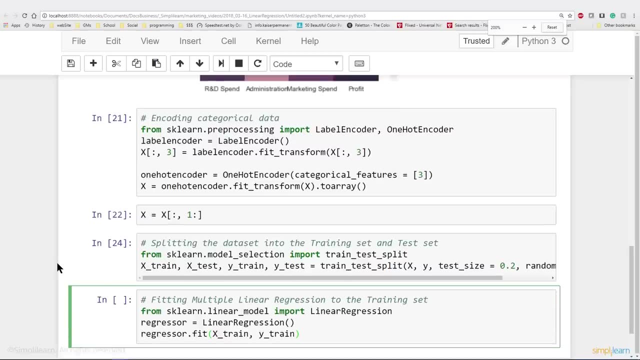 Now that we got to the linear regression model, we get that next piece of the puzzle. Let's go ahead and put that code in there and walk through it. So here we go, We're going to paste it in there And let's go ahead. and since this is a shorter line of code, let's zoom up there so we can. 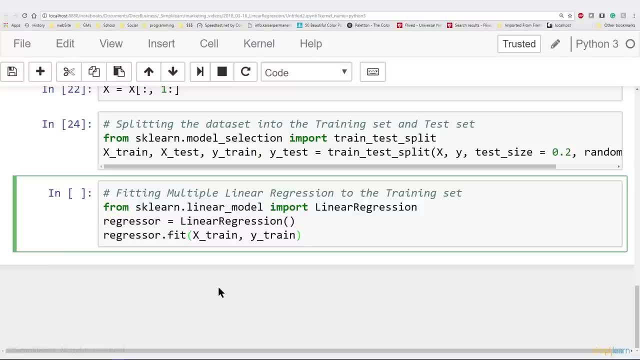 get a good look And we have from the sklearnlinear underscore model. we're going to import linear regression Now. I don't know if you recall from earlier when we were doing all the math. Let's go ahead and flip back there and take a look at that. 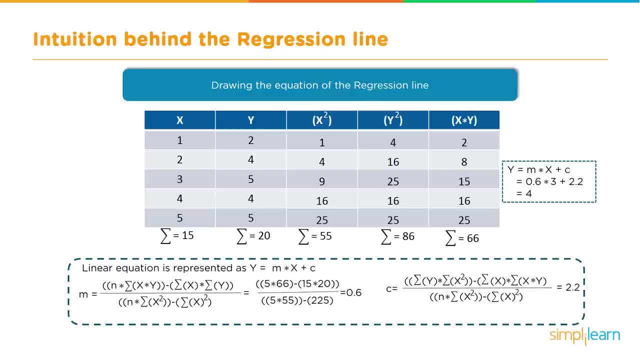 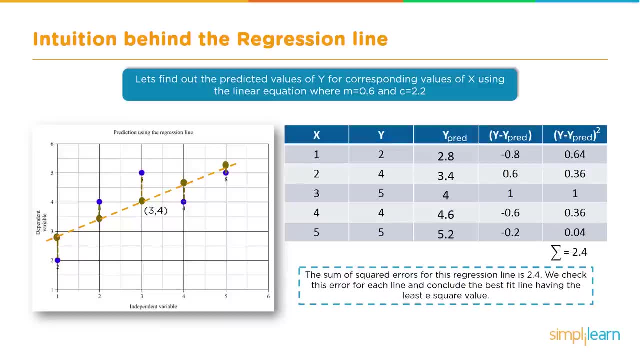 Do you remember this where we had this long formula on the bottom and we were doing all this sumization, And then we also looked at setting it up with the different lines, And then we also looked all the way down to Multiple linear regression, where we're adding all those formulas together. 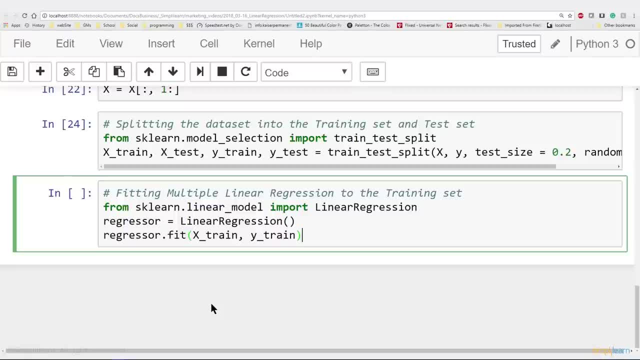 All of that is wrapped up in this one section. So what's going on here is I'm going to create a variable called regressor, And the regressor equals the linear regression. That's a linear regression model that has all that math built in. 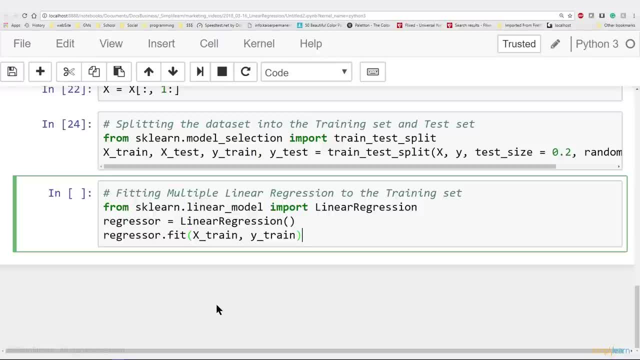 So we don't have to have it all memorized or have to compute it individually. And then we do the regressor dot fit. In this case we do X train and Y train, because we're using the training data, X being the data in and Y being profit. 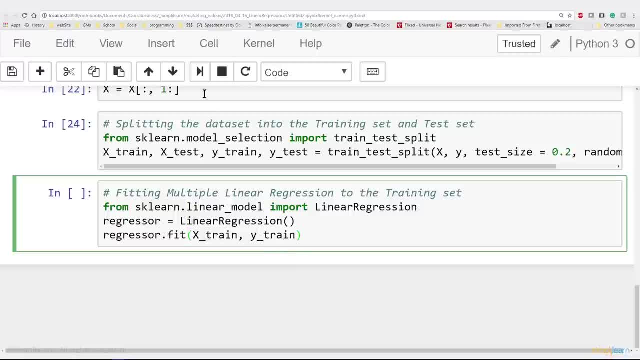 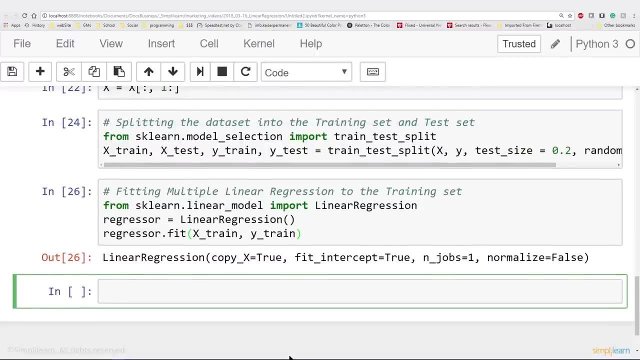 What we're looking at And this does all that math for us. So within one click and one line we've created the whole linear regression model And we fit the data to the linear regression model And you can see that when I run the regressor it gives an output: linear regression. 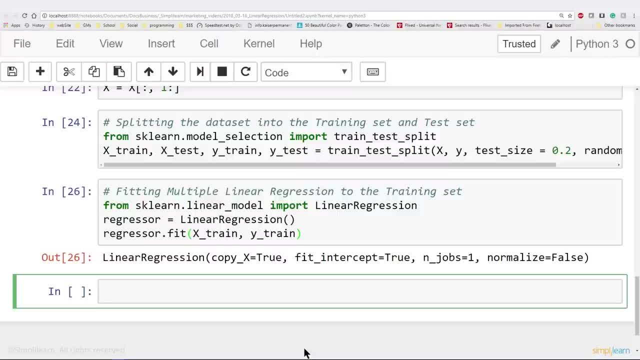 It says: copy X equals true, fit intercept equals true. in jobs equal one, normalized equals false. It's just giving you some general information on what's going on with that regressor model. Now that we've created our linear regression model, let's go ahead and use it. 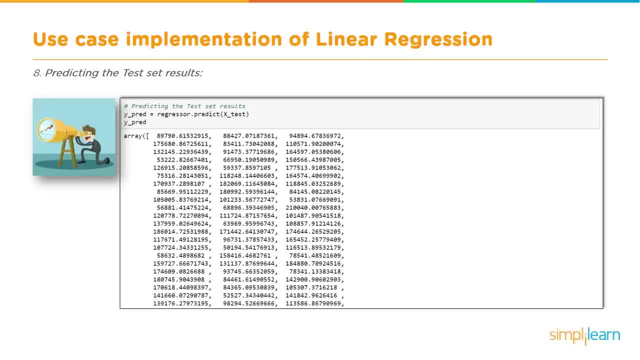 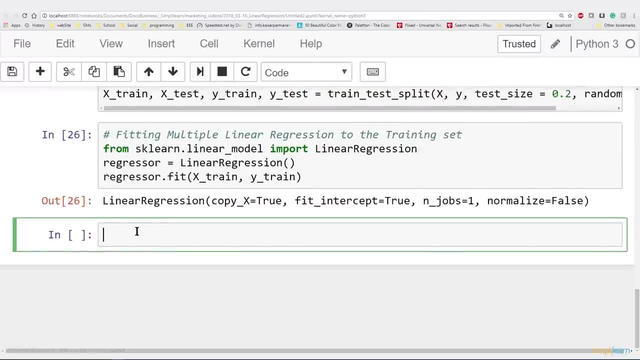 And, if you remember, we kept a bunch of data Data side. So we're going to do a Y predict variable And we're going to put in the X test And let's see what that looks like. Scroll up a little bit. 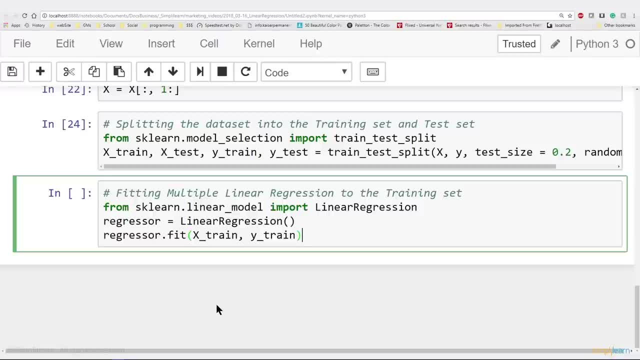 So we don't have to have it all memorized or have to compute it individually. And then we do the regressorfit. In this case, we do x train and y train, because we're using the training data, X being the data in and y being profit. what we're looking at. 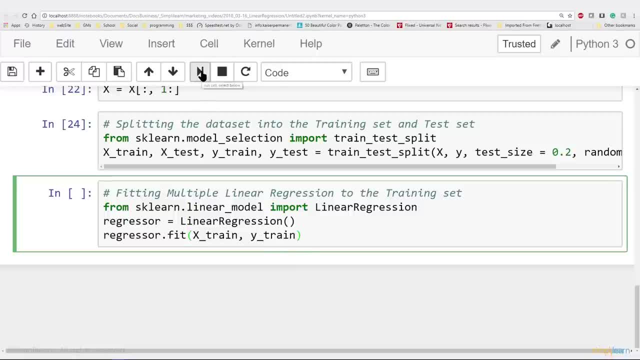 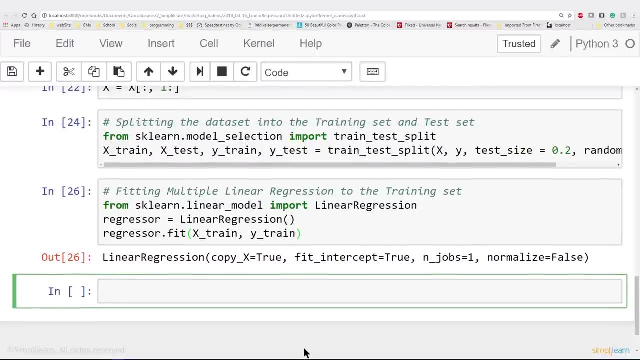 And this does all that math for us. So within one click and one line we've created the whole linear regression model And we fit the data to the linear regression model And you can see that when I run the regressor it gives an output: linear regression. 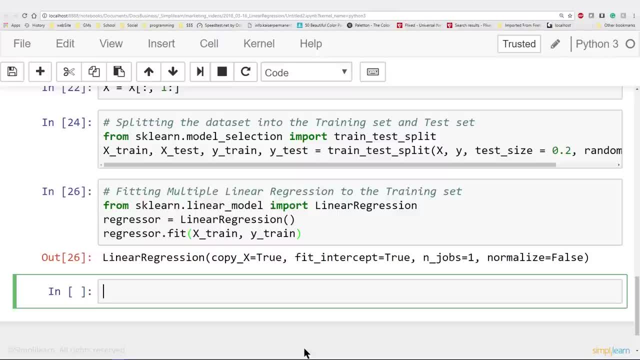 It says: copy x equals true, fit intercept equals true. in jobs equal one, normalize equals false. It's just giving you some general information on what's going on with that regressor model. Now that we've created our linear regression model, let's go ahead and use it. 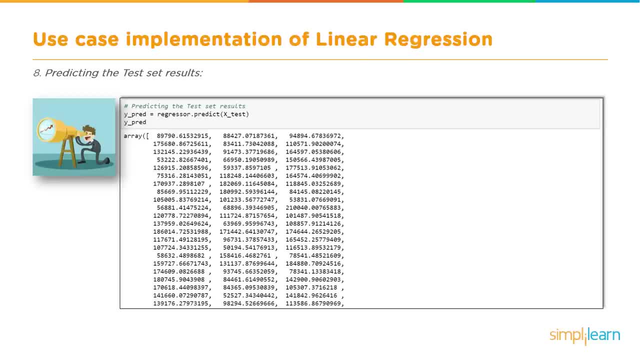 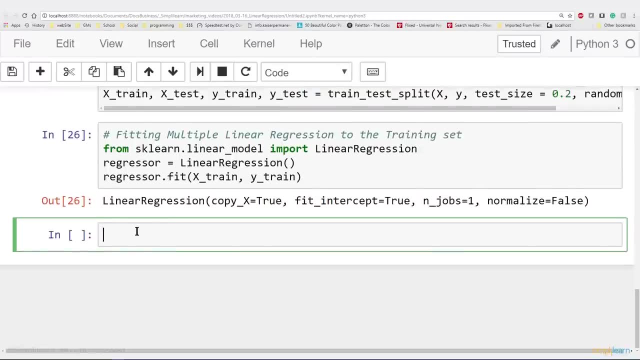 And, if you remember, we kept a bunch of data. So we're going to do a y predict variable And we're going to put in the x test And let's see what that looks like. Scroll up a little bit, paste that in here. 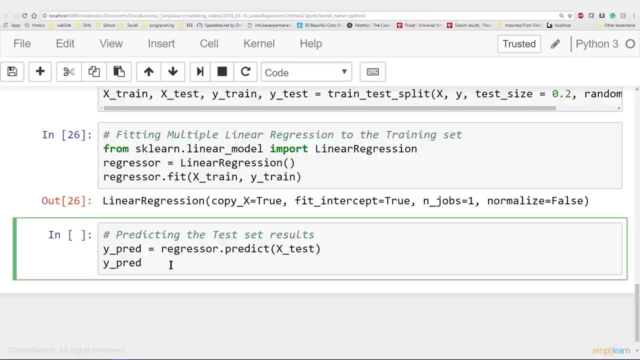 Predicting the test set results. So here we have y predict equals regressorpredict x test going in And this gives us y predict. Now, because I'm in Jupyter inline, I can just put the variable up there And when I hit the run button it'll print that array out. 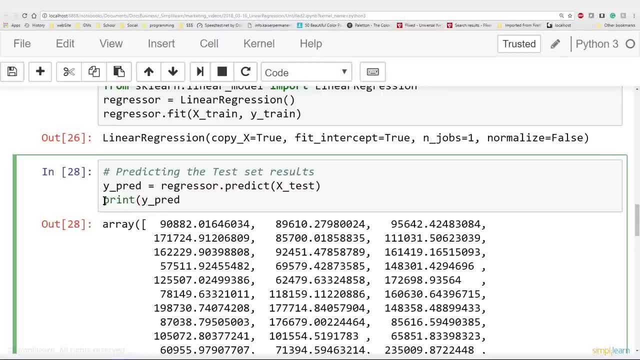 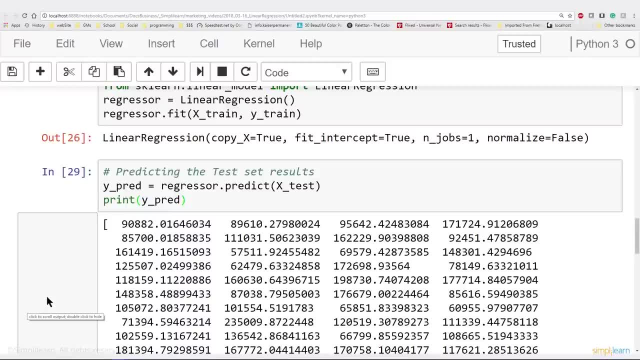 I could have just as easily done print Y predict. So if you're in a different IDE- that's not an inline setup like the Jupyter Notebook- you can do it this way: Print y predict And you'll see that for the 200 different test variables we kept off to the side, it's 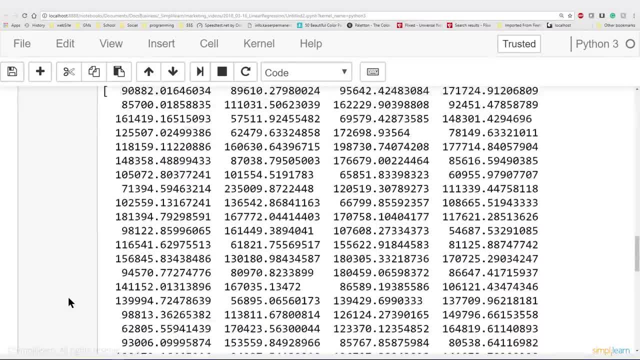 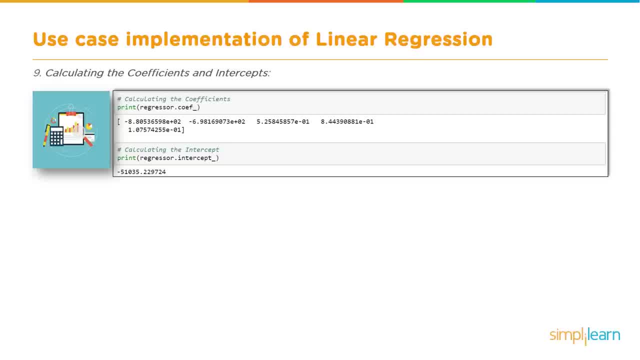 going to produce 200 answers. This is what it says the profit are for those 200 predictions. But let's don't stop there, Let's keep going and take a couple. look, We're going to take just a short detail here in calculating the coefficients and the intercepts. 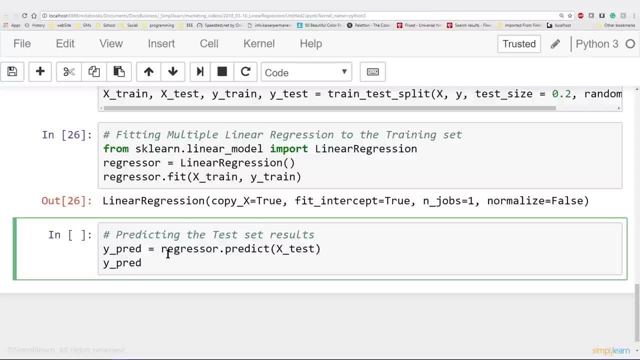 Paste that in here. Predicting the test set results. So here we have Y predict equals regressor dot predict X test going in And this gives us Y predict. Now, because I'm in Jupyter inline, I can just put the variable up there. 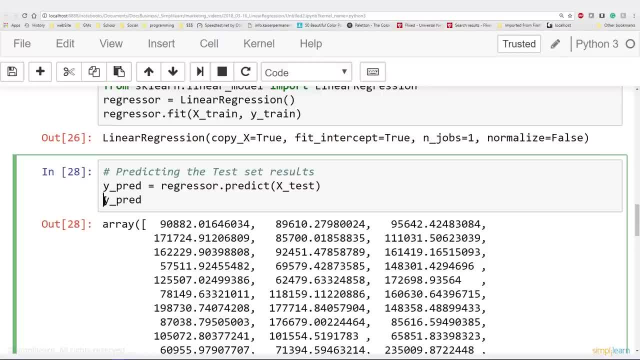 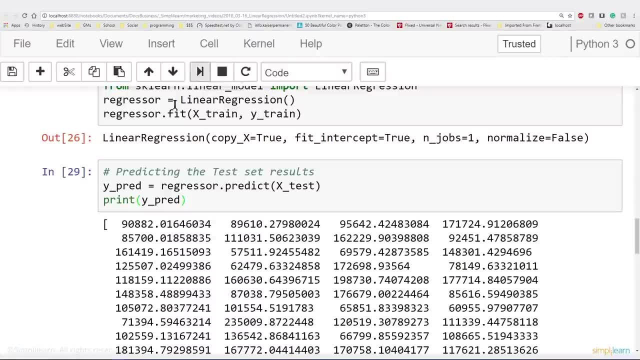 And when I hit the run button it'll print that array out. I could have just as easily done print Y, predict. So if you're in a different IDE- that's not an inline setup like the Jupyter notebook- you can do it this way. 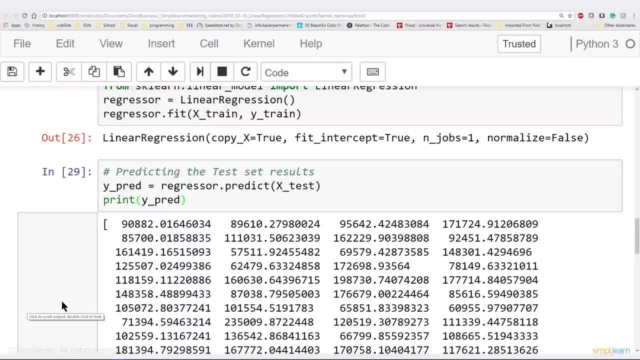 Print Y predict And you'll see that for the 200 different test variables we kept off to the side, it's going to produce 200 answers. This is what it says. the profit are for those 200 predictions. But let's don't stop there. 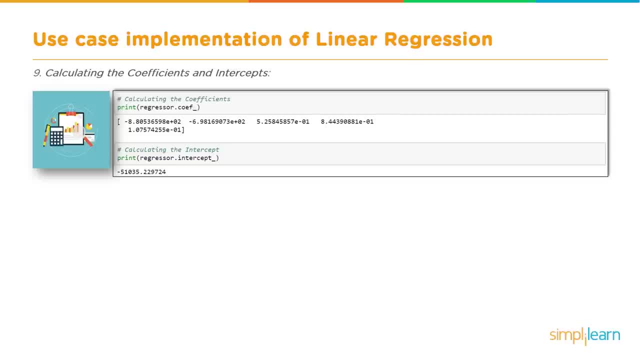 Let's keep going and take a couple look- We're going to take just a short detail here- and calculating the coefficients and the intercepts. This gives us a quick flash at what's going on behind the line. We're going to take a short detour here. 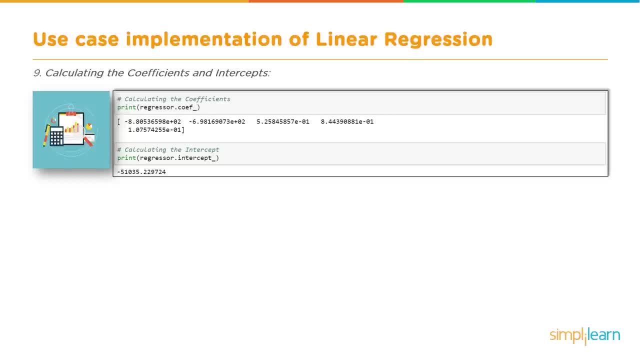 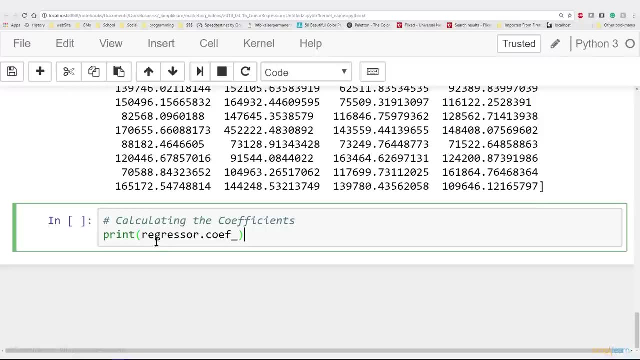 And we're going to be calculating the coefficient and intercepts So you can see what those look like. What's really nice about our regressor we created is it already has a coefficients for us. We can simply just print regressor dot coefficient underscore. 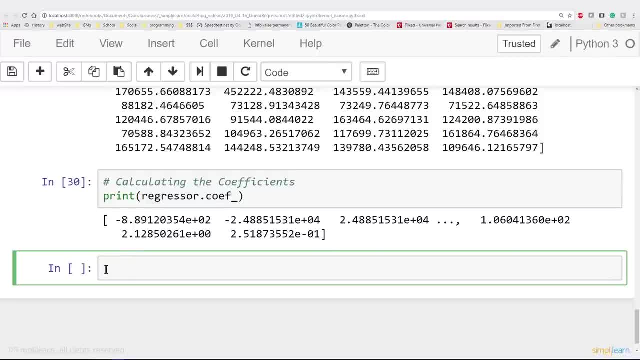 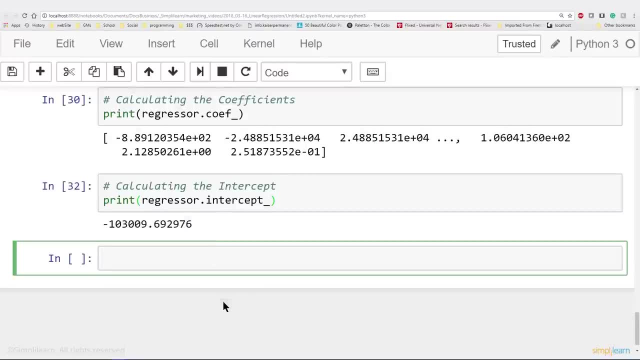 When I run this, you'll see our coefficients here, And if we can do the regressor coefficient, we can also do the regressor intercept. Let's run that and take a look at that. This all came from the multiple regression model. 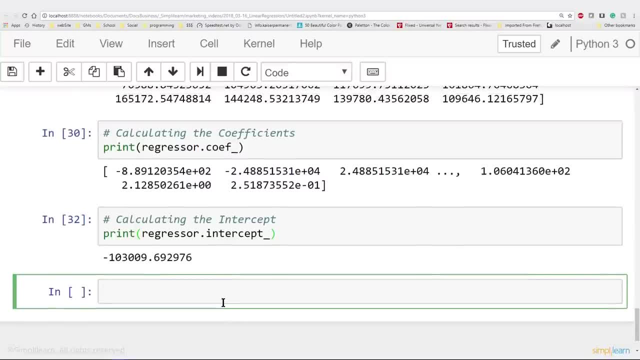 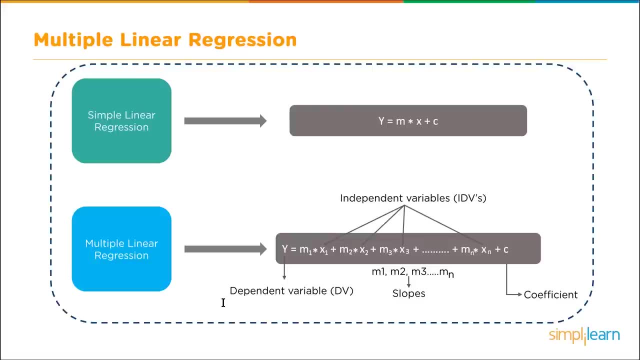 And we'll flip over So you can remember where this is going into and where it's coming from. You can see the formula down here, where y equals m1 times x1 plus m2 times x2, and so on and so on, plus c, the coefficient. 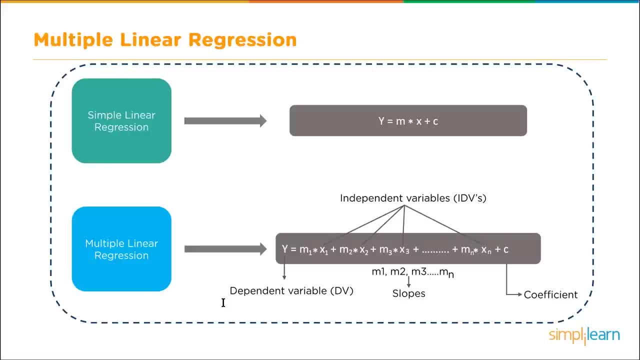 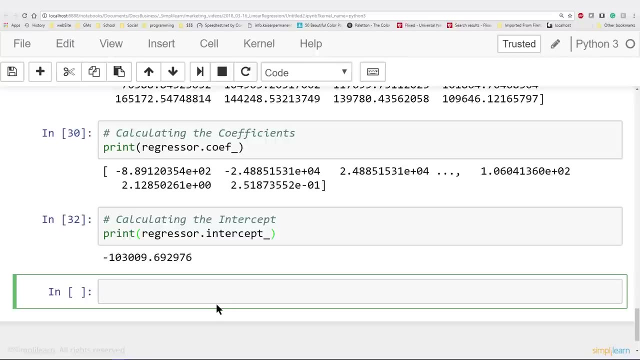 So these variables fit right into this formula. y equals slope 1 times column 1 variable, plus slope 2 times column 2 variable, all the way to the m, to the n and x to the n plus c, the coefficient, Or in this case you have minus 8.89 to the power of 2.. 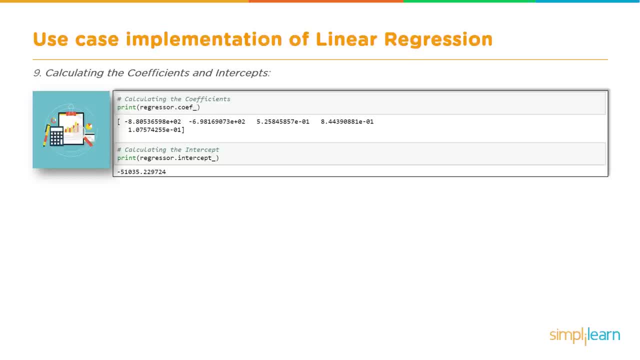 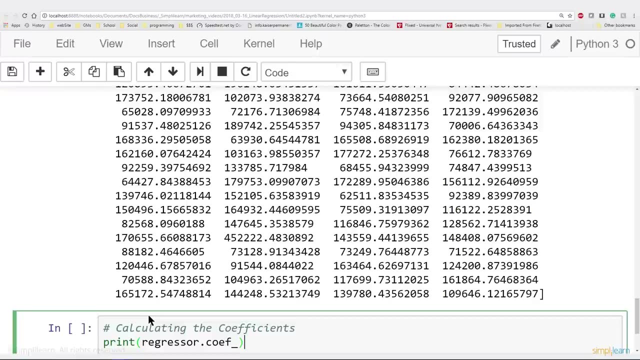 This gives us a quick flash at what's going on behind the line. We're going to take a short look, We're going to take a short detour here and we're going to be calculating the coefficient and intercepts So you can see what those look like. 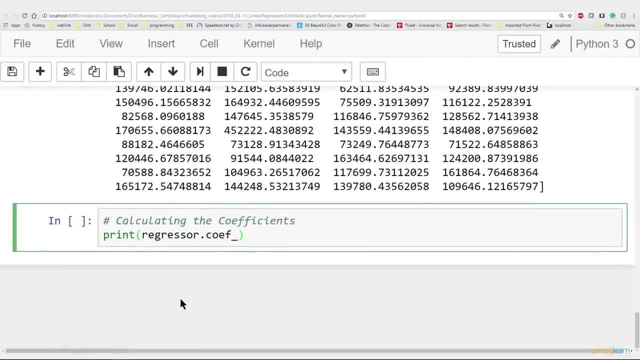 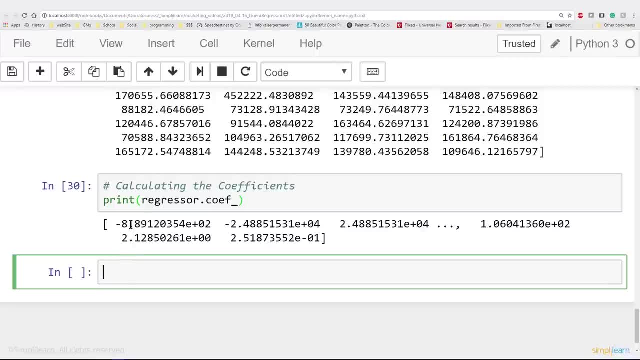 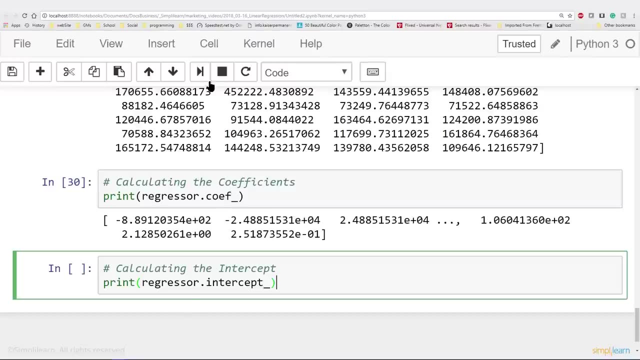 What's really nice about our regressor we created is it already has the coefficients for us. We can simply just print regressorcoefficient underscore. When I run this, you'll see our coefficients here, And if we can do the regressor coefficient, we can also do the regressor intercept. 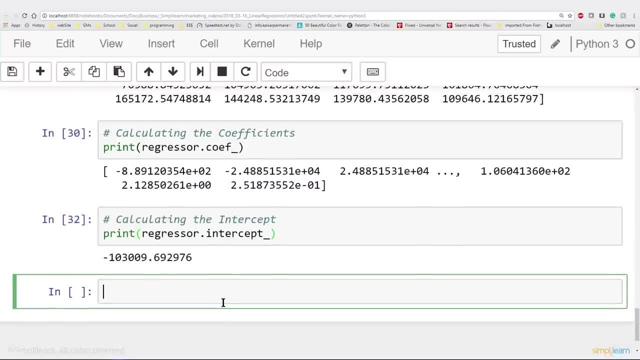 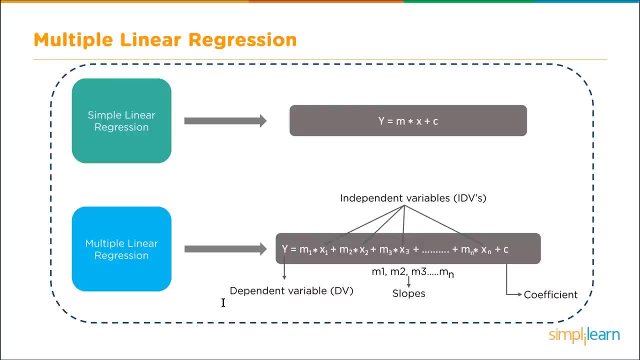 Let's run that and take a look at that. This all came from the multiple regression model And we'll flip over so you can remember where this is going into and where it's coming from. You can see the formula down here, where y equals m1 times x1 plus m2 times x2, and so 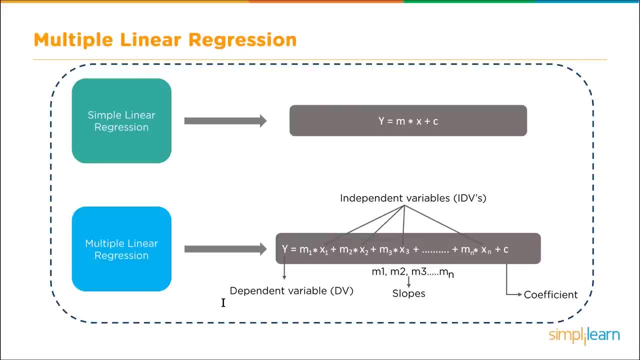 on and so on, plus c the coefficient. So these variables fit right into this formula. Y equals slope 1 times column 1 variable, plus slope 2 times column 2 variable, all the way to the m, to the n and x to the n, plus c the coefficient. 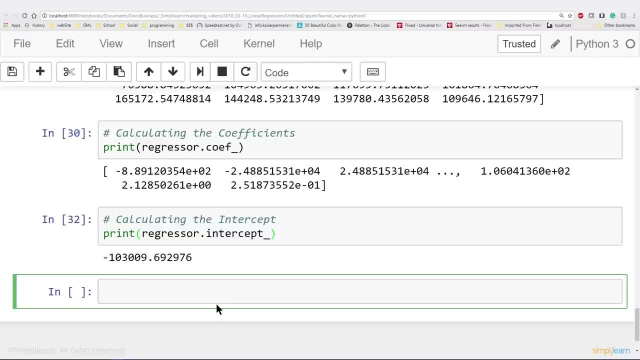 Or in this case, you have minus 8.89 to the power of 2.5.. So that's the coefficient And we'll flip over so you can remember where this is going into and where it's coming from. So we have minus 8.89 to the power of 2, et cetera, et cetera times the first column. 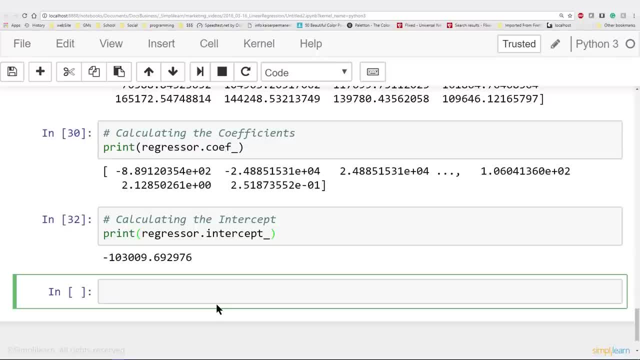 and the second column and the third column, And then our intercept is the minus 103009 point. Boy, it gets kind of complicated when you look at it. This is why we don't do this by hand anymore. This is why we have the computer to make these calculations easy to understand and calculate. 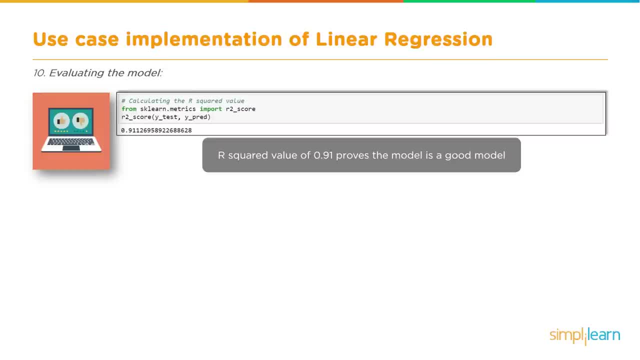 Now I told you that was a short detour and we're coming towards the end of our script. As you remember, from the beginning I said, if we're going to divide this information, we have to make sure it's a valid model, That this model works. 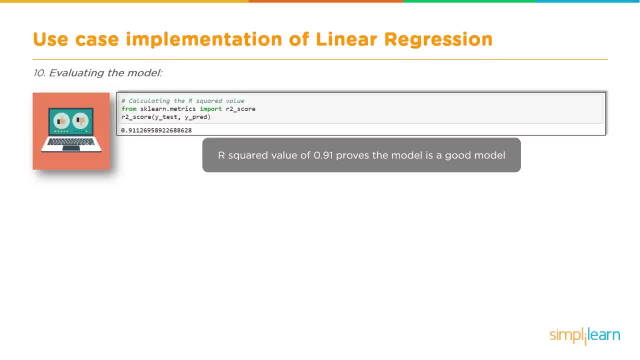 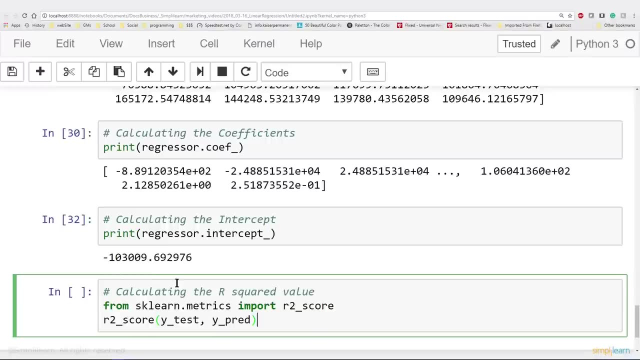 And how good it works. So, calculating the r-squared value, that's what we're going to use to predict how good our prediction is. And let's take a look at what that looks like in code. And so we're going to use this from sklearnmetrics. 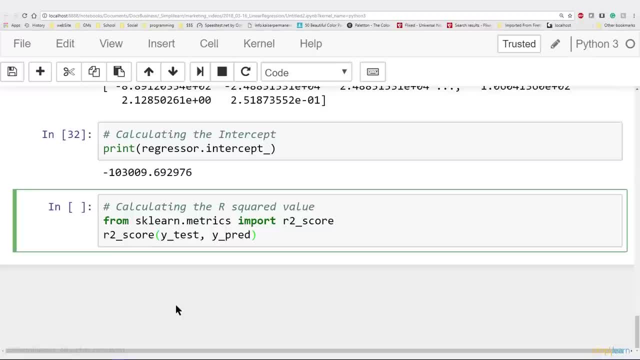 We're going to import r2score. That's the r-squared value. We're looking at the error. So in the r2score we take our ytest versus our ypredict. Ytest is the actual values we're testing. 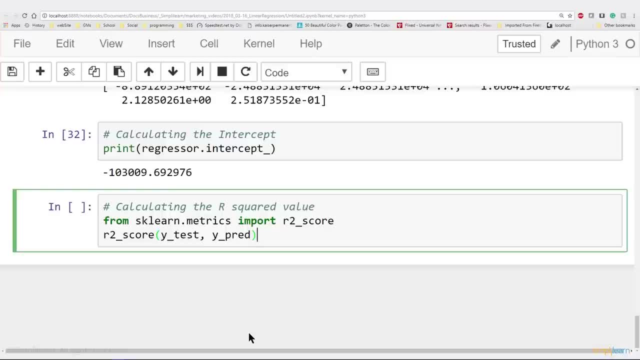 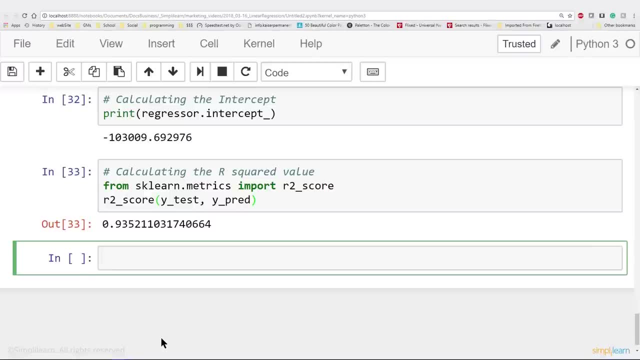 That was the one that was given to us that we know are true. Ypredict of those 200 values is what we think it was true And when we go ahead and run this we see we get a .9352.. That's the r2score. 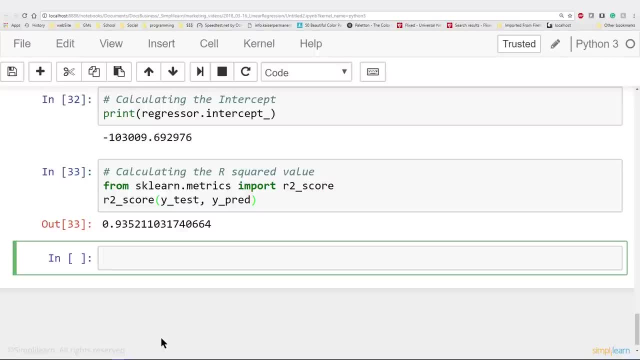 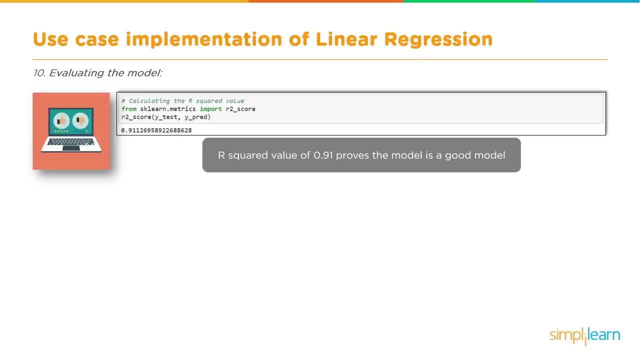 Now it's not exactly a straight percentage, So it's not saying it's 93% correct, But you do want. that in the upper 90s and higher shows that this is a very valid prediction based on the r2score And if r-squared value of .91 or 92, as we got on our model, remember it does have a. 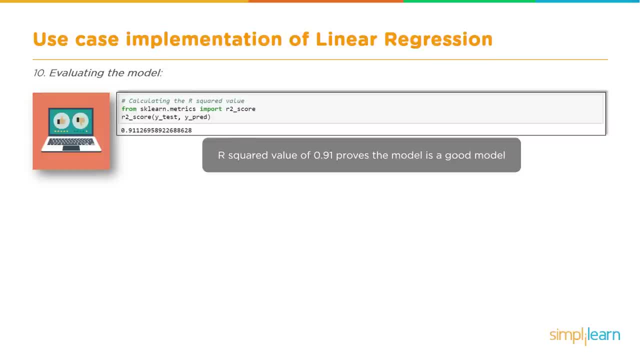 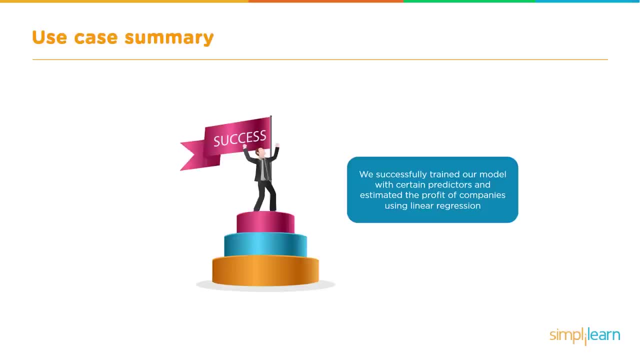 random generation involved. This proves the model is a good model, which means success. Yay, We successfully trained our model with certain predictors and estimated the profit of the companies using linear regression. So now that we have a successful linear regression model, let's take a look at what we went over. 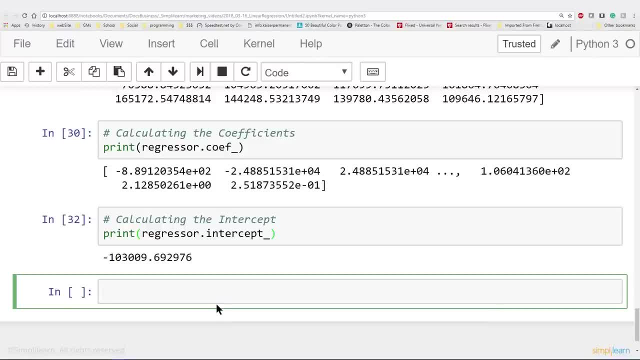 And that's actually what Iなんです here. So that looks like a nice structure. And you see the all the way to the left. I've got the unit and I've got the opposite, And I've got the intersection, the minus 1 and the minus 2.. 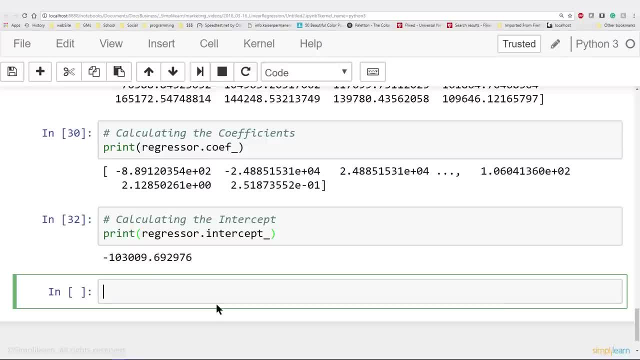 And then I've got the first column and the second column, like that, And then I've got the center of the value of 1. And I've got the inner value of 1. And I've got the upper value of 1.. 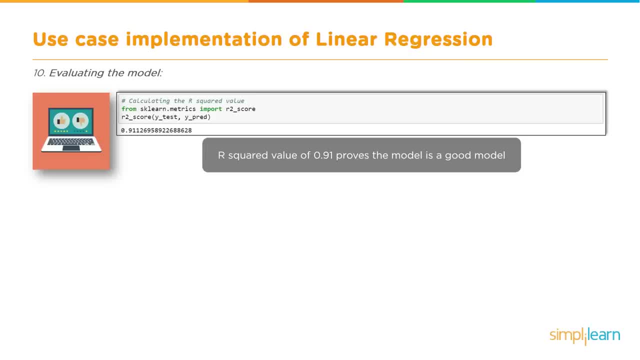 And then I've got the first column and the second column and the third column, And then our intercept is the minus 1, 0, 3, 0, 0, 9 point. Boy, it gets kind of complicated when you look at it. 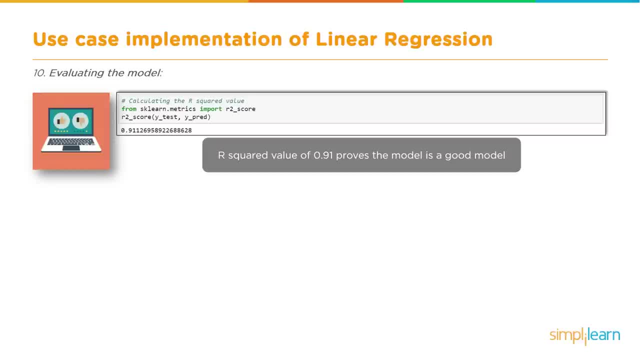 This is why we don't do this by hand anymore. This is why we have the computer to make these calculations easy to understand and calculate. So, calculating the R squared value, That's what we're going to use to predict how good our prediction is. 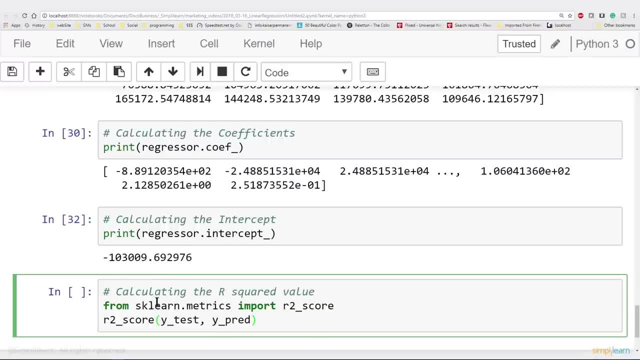 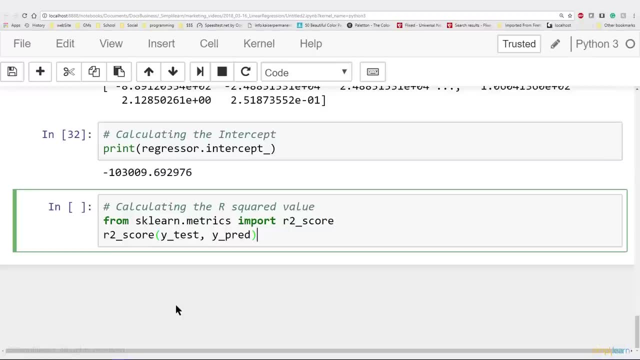 And let's take a look at what that looks like in code. And so we're going to use this from sklearnmetrics. We're going to import R2 score. That's the R squared value. We're looking at the error. So in the R2 score we take our Y test versus our Y predict. 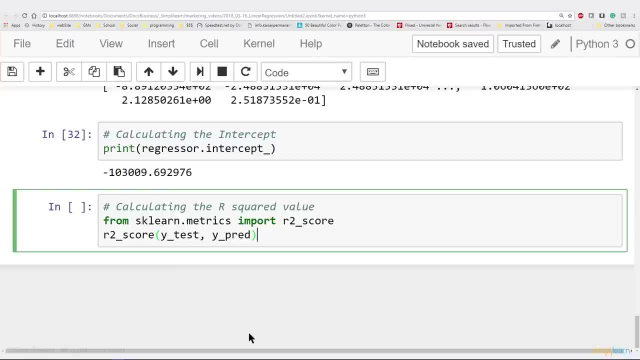 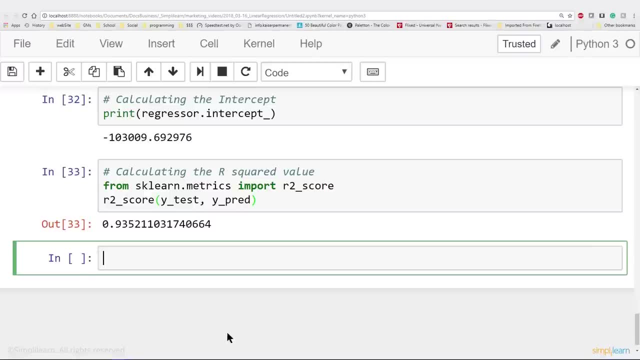 Y test is the actual values we're testing. That was the one that was given to us that we know are true. The Y predict of those 200 values is what we think it was true And when we go ahead and run this we see we get a .9352.. That's the R2 score. 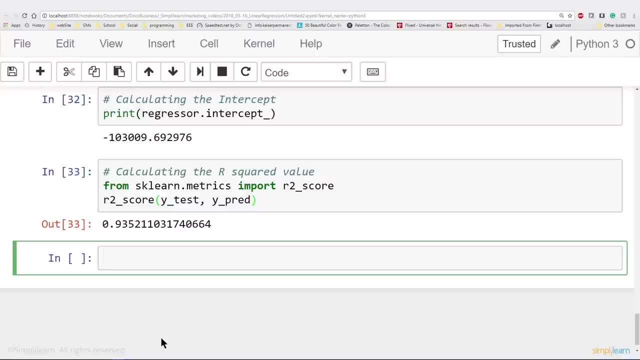 Now it's not exactly a straight percentage, so it's not saying it's 93% correct, But you do want that in the upper 90s. Oh and higher shows that this is a very valid prediction based on the R2 score. 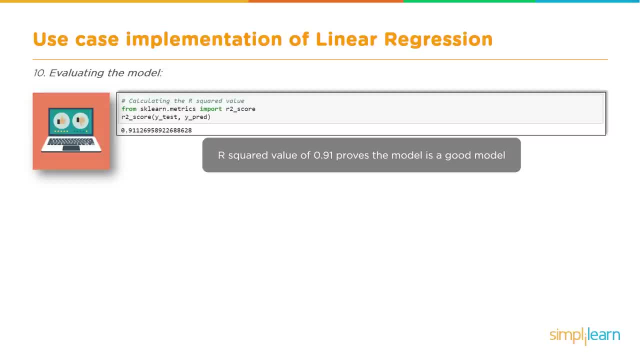 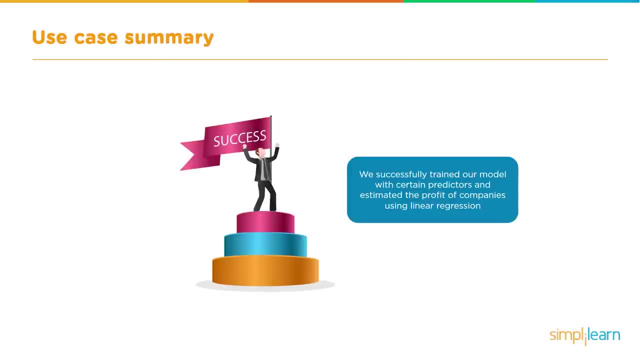 And if R squared value of .91 or 92, as we got on our model- because, remember, it does have a random generation involved, this proves the model is a good model, which means success. Yay, We successfully trained our model with certain predictors and estimated the profit of the companies using linear regression. 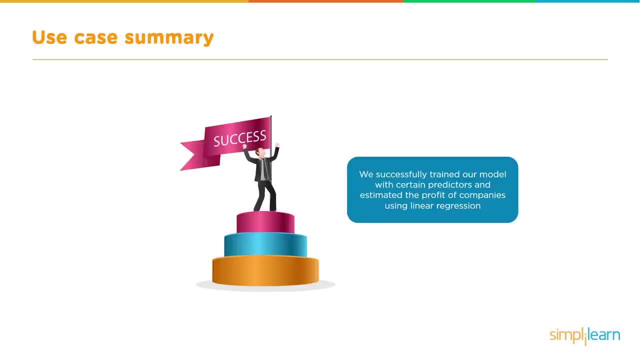 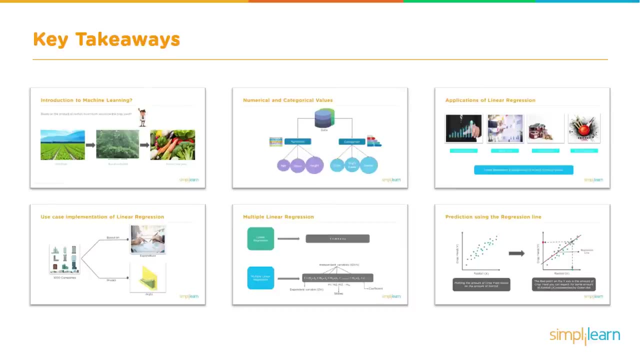 So, now that we have a successful linear regression model, let's take a look at what we went over today and take a look at our key takeaways. First, we have an introduction to machine learning. We talked about some general setup in predicting crops and weather. 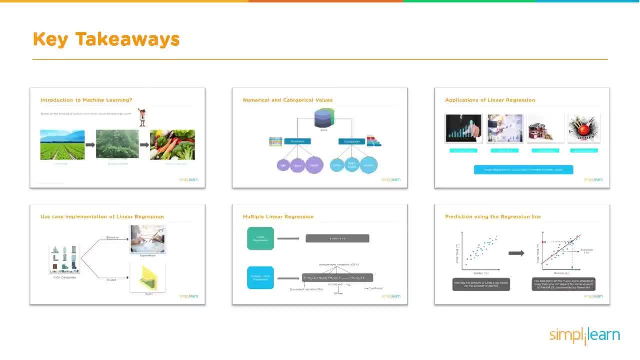 We saw this: that numbers are age, salary and so on. We have categorical color. When we did our actual regression model, we saw that we had numbers which was dollar amounts And we had a location which was Florida and New York, which was categorical, that we had to convert. 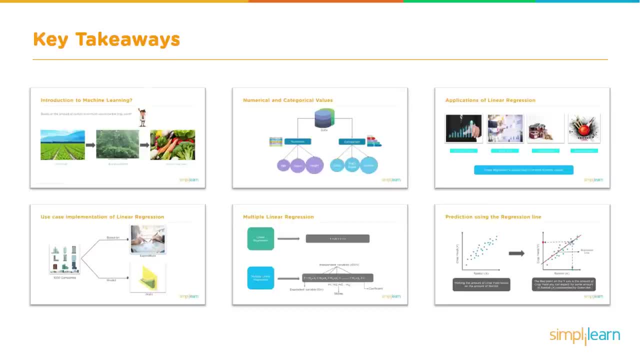 Next we have application of a linear regression model. We had some- I'm showing here some different applications you could use it for. We had our use case implementation of linear regression where we dug in deep and showed how those are set up.